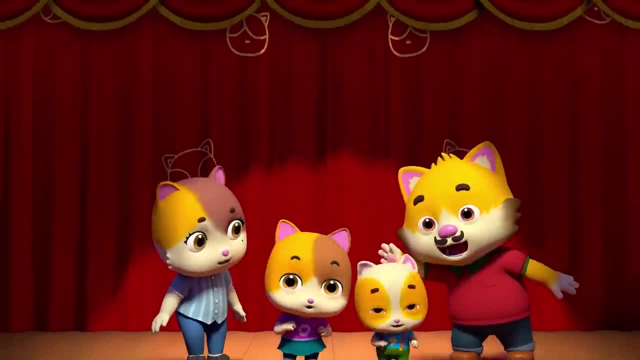 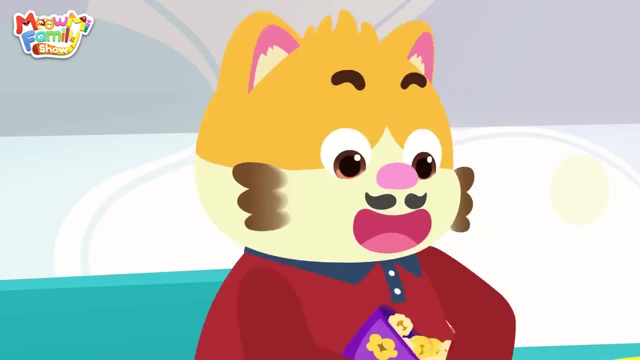 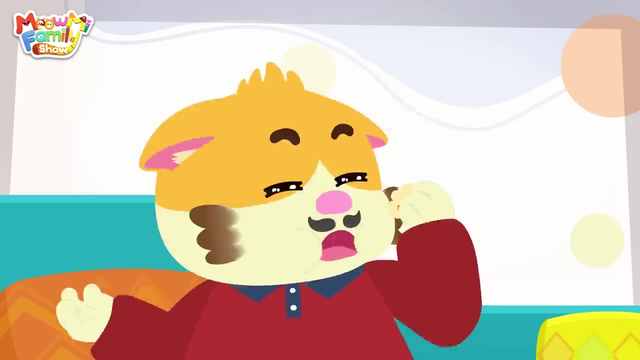 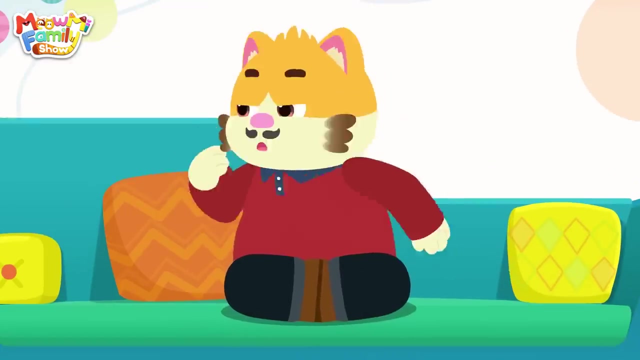 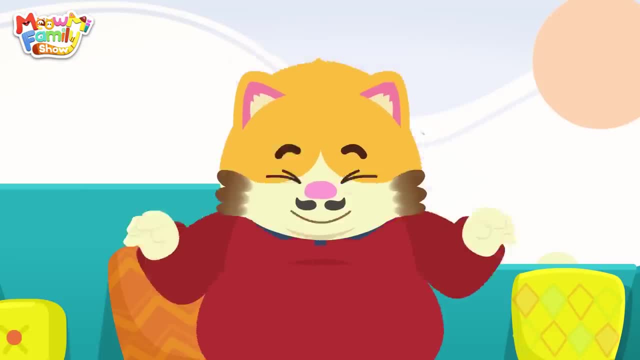 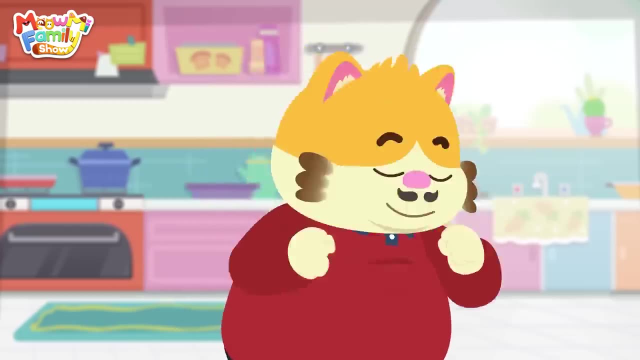 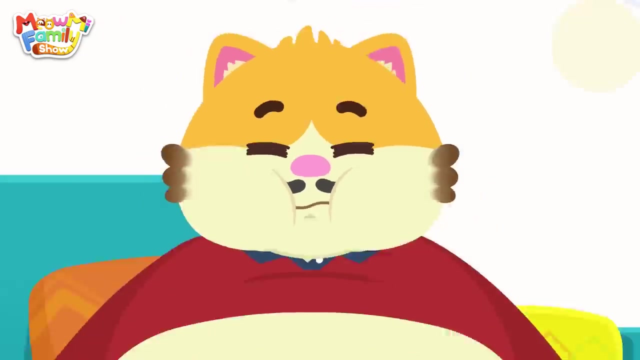 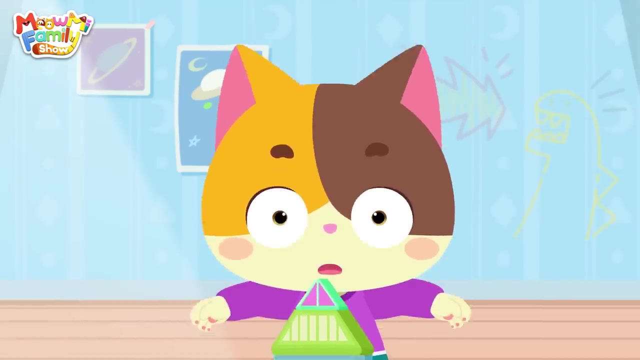 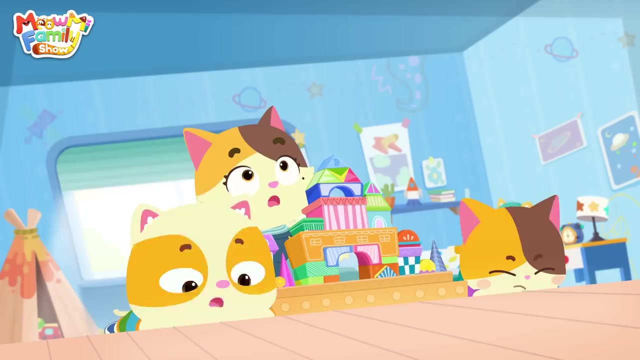 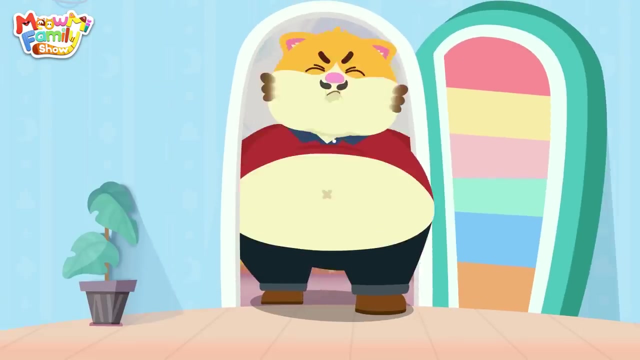 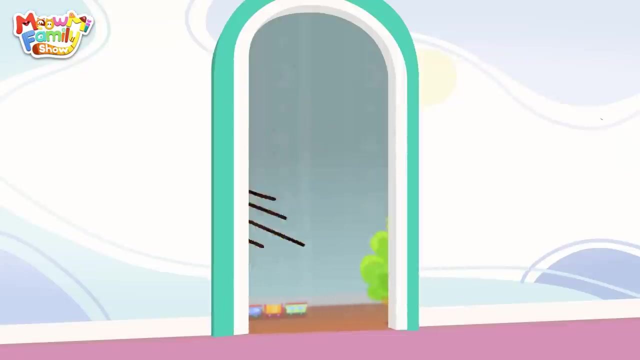 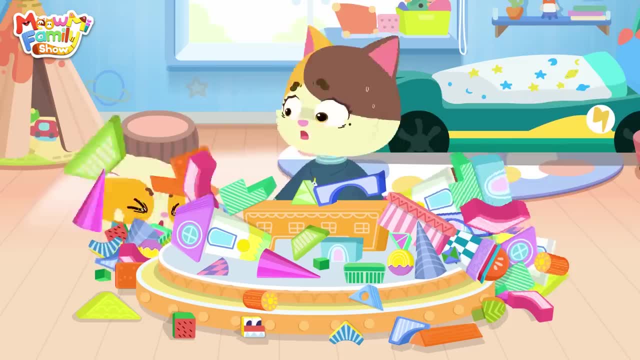 The door got smaller, Rrrrrrrrrrrrrrrrrrrrr, Rrrrrrrrrrrrrrrrr, Rrrrrrrrrrrrrrrrrrrrr, Rrrrrrrrrrrrrrrrrr Ah. 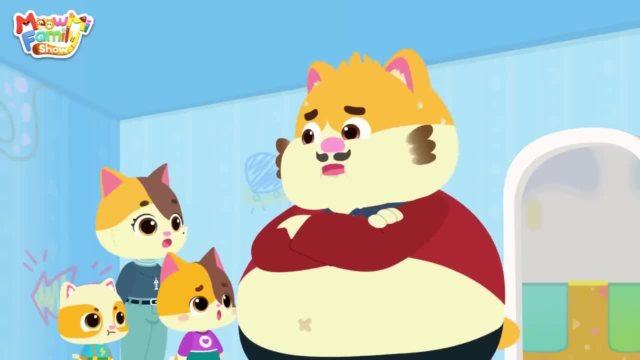 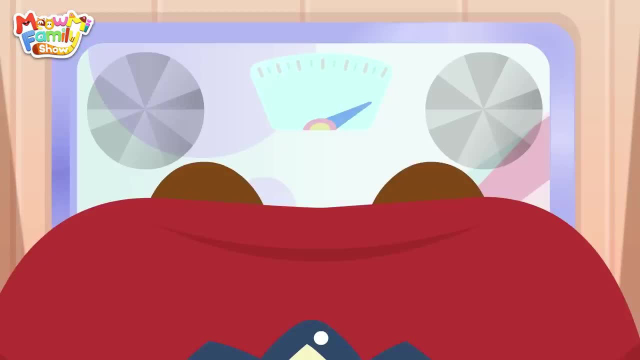 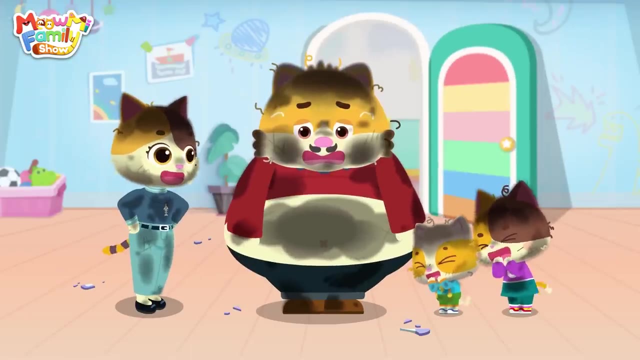 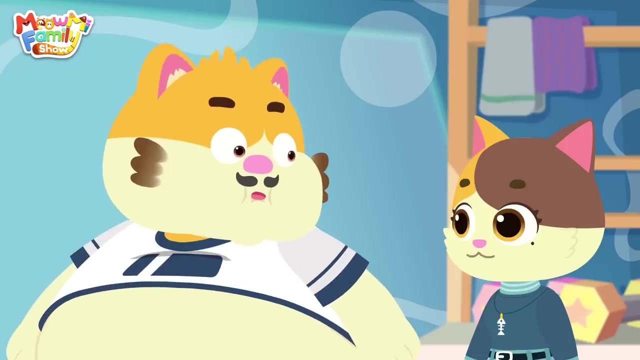 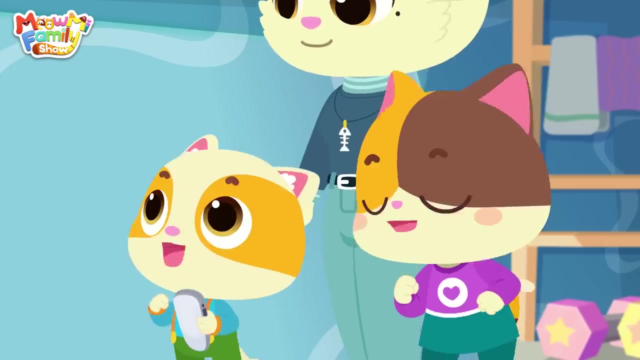 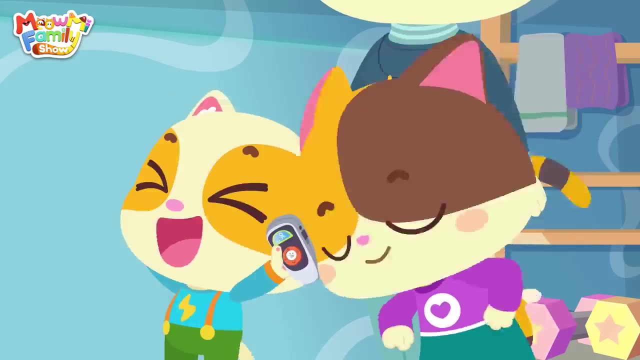 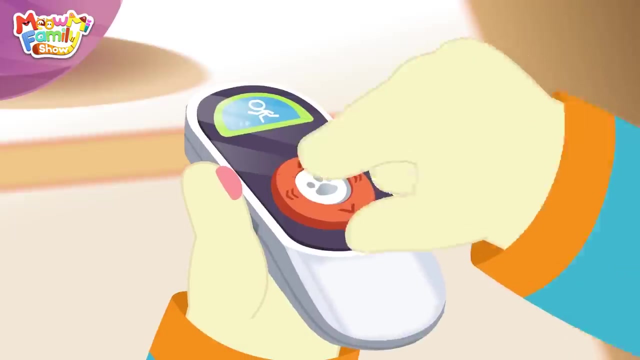 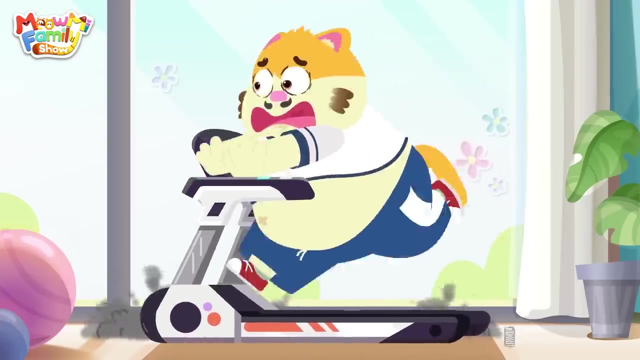 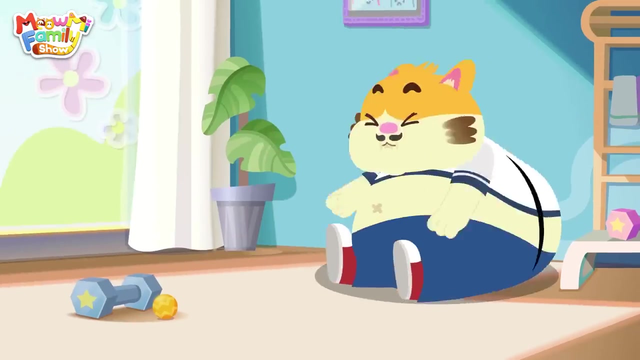 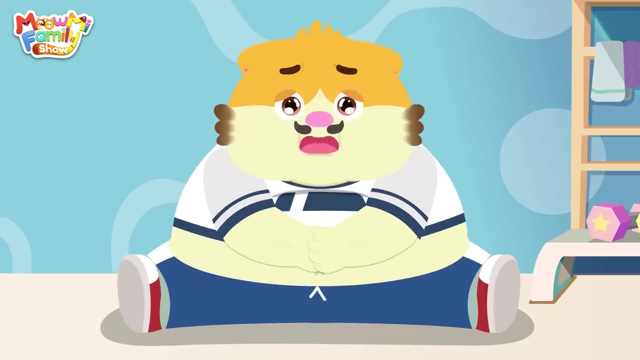 My castle Daddy's gained too much weight. Uh, oh, No way. Go, weigh yourself yourself. you need to lose weight, honey. running can help you lose weight. I'm really good at running faster. faster, that's so easy, are you? okay? it's all my fault. the 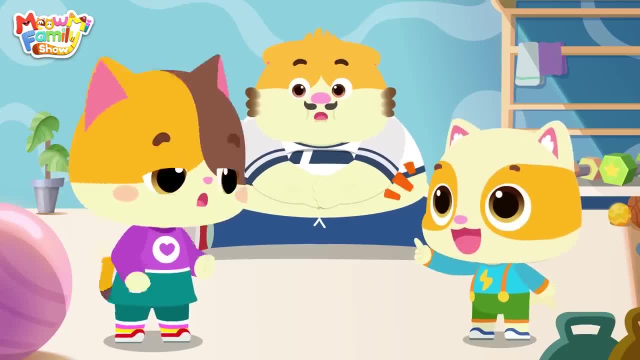 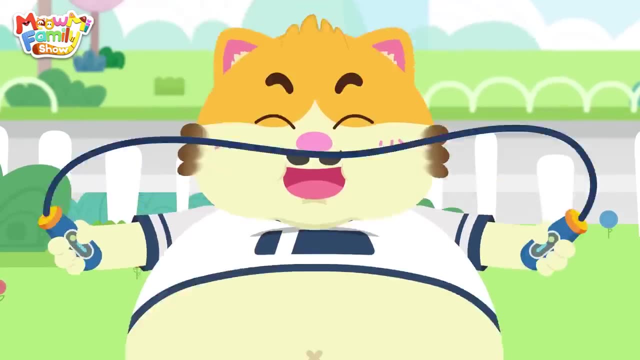 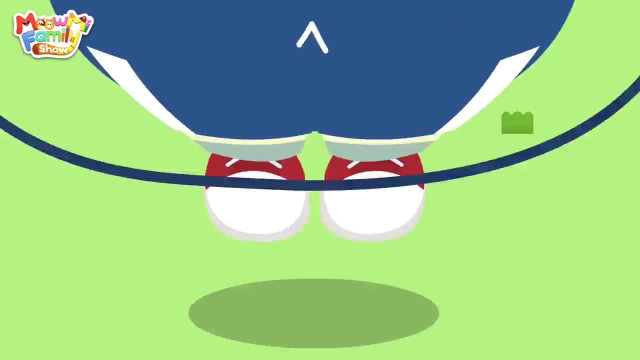 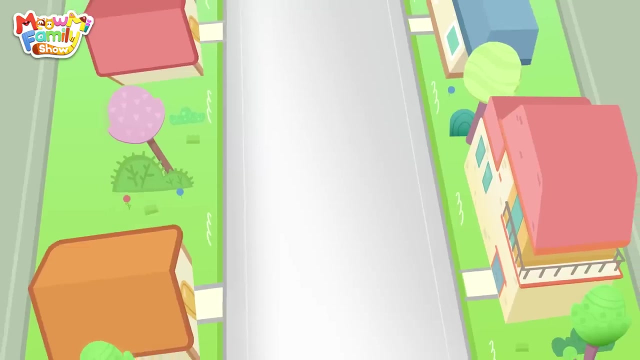 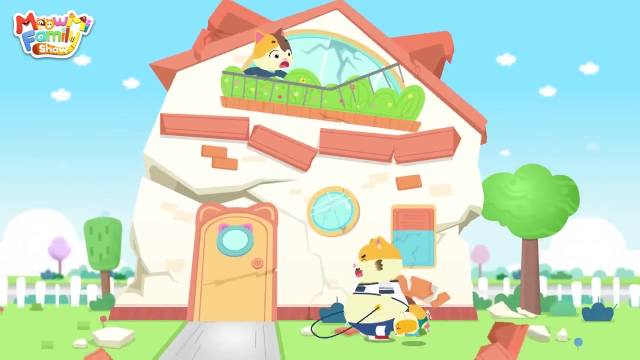 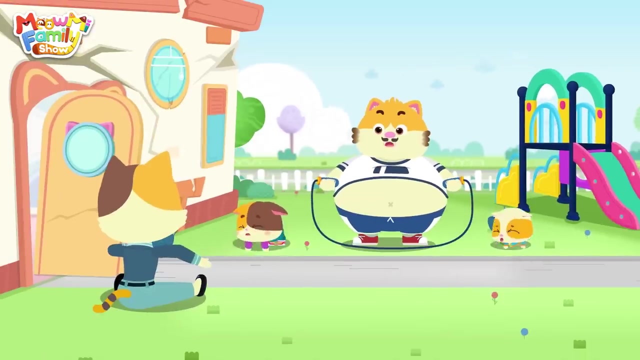 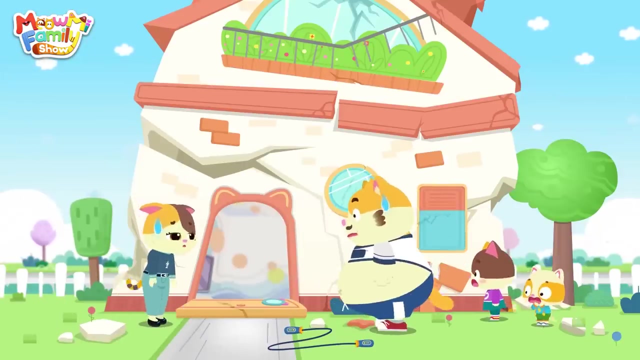 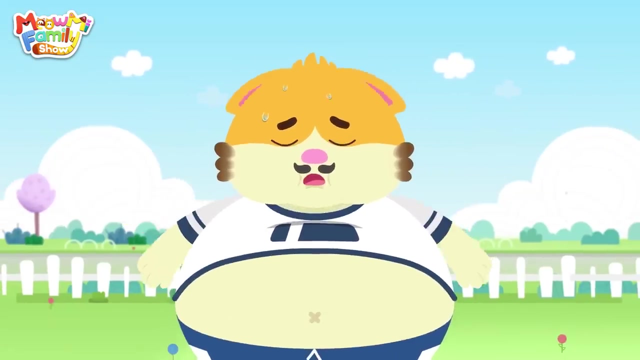 treadmills broken. let's try another exercise. how about jumping rope? great, go for it. what's wrong, honey? if you keep jumping like that, we'll have to find a new home. I'm not losing any weight. does exercise really help? Oh, Oh, Oh, Oh Oh. I have an idea. 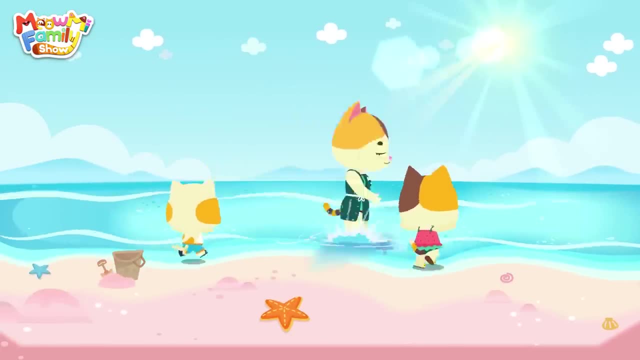 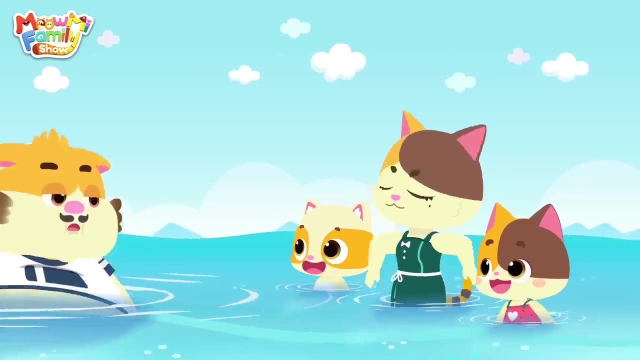 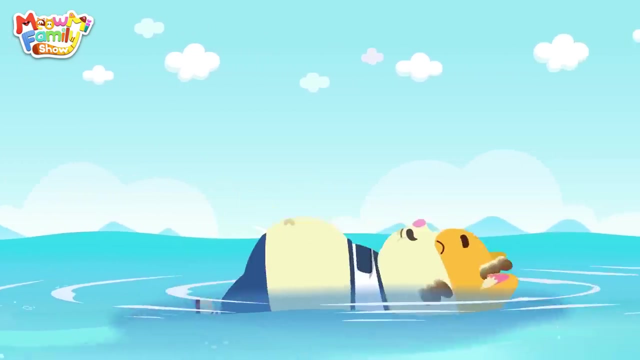 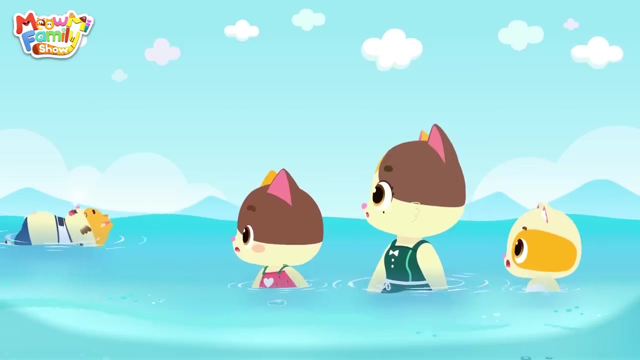 okay, you can do it. we're sure you lose a way to exercise. doesn't help anyway, I'll just take it easy. that's it I'm. I'll just take it easy, that's it I'm. I'll just take it easy, that's it I'm. 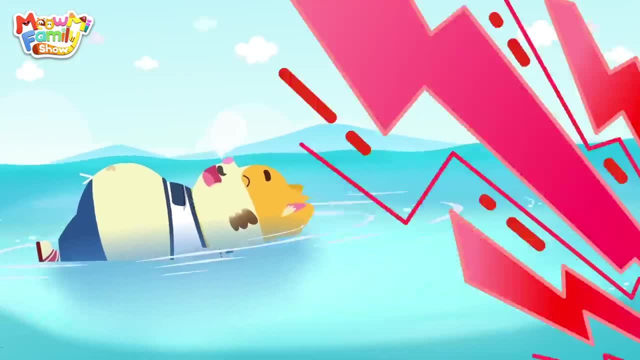 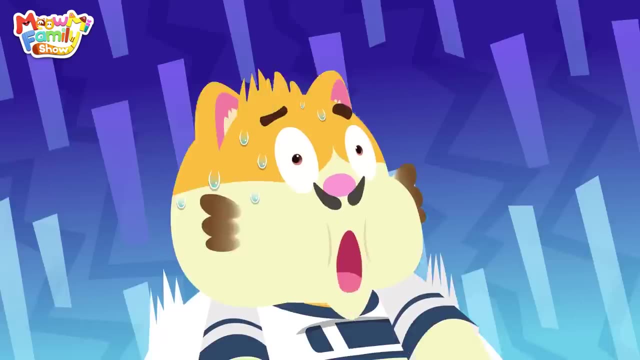 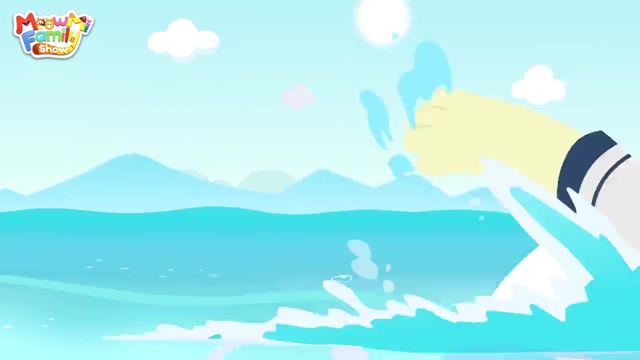 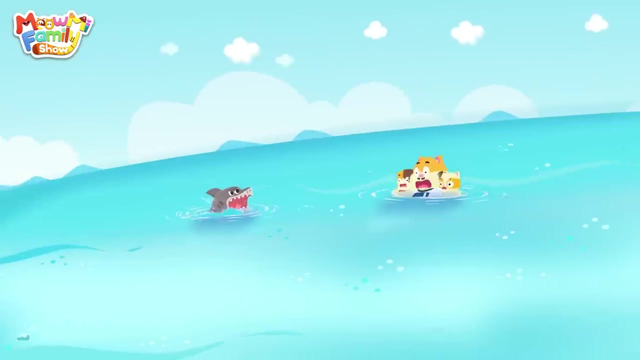 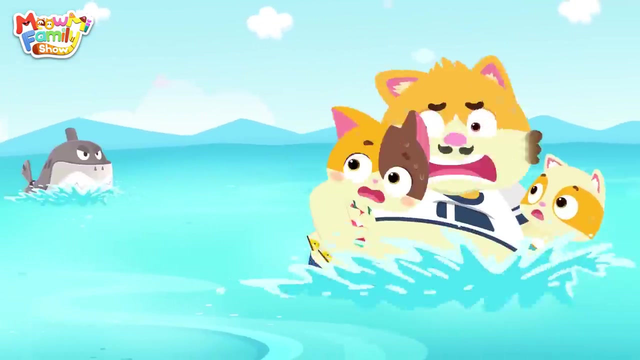 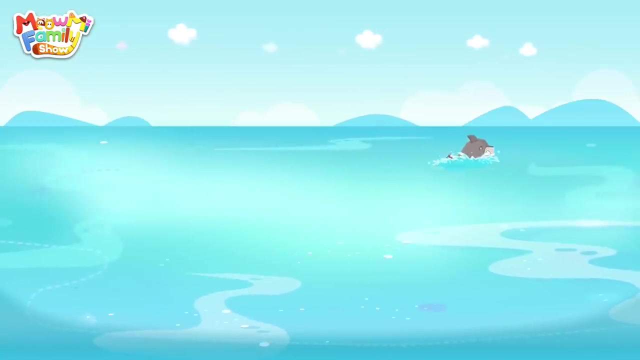 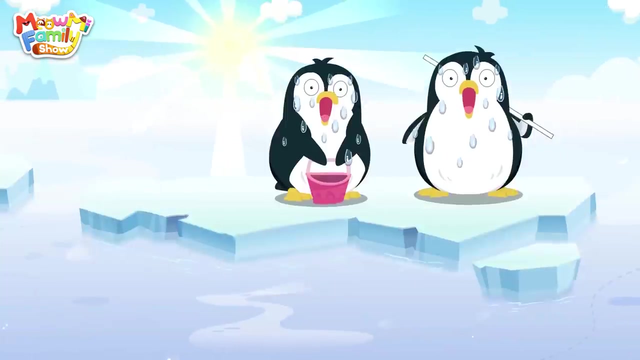 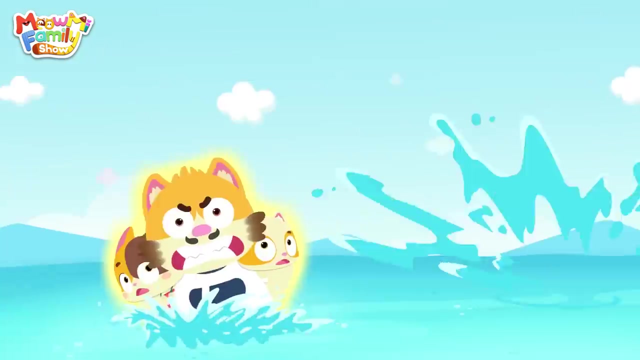 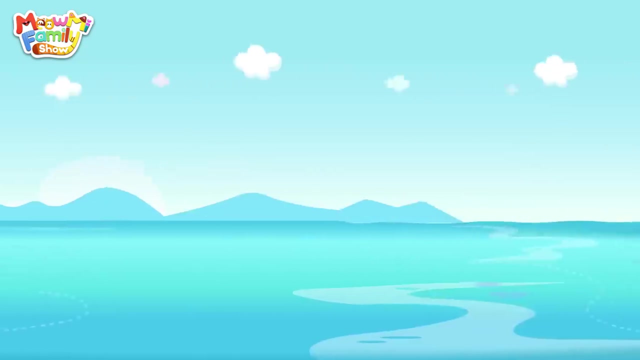 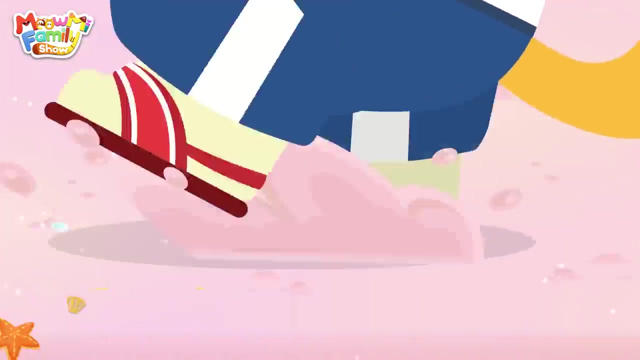 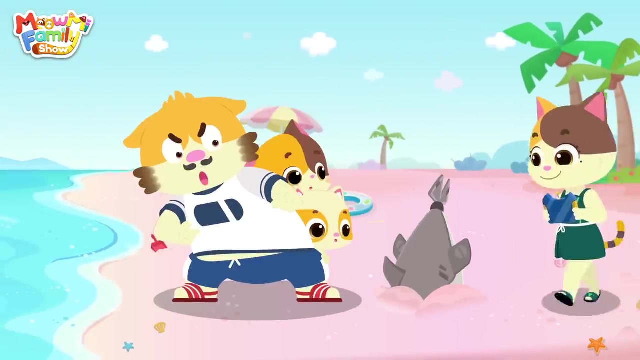 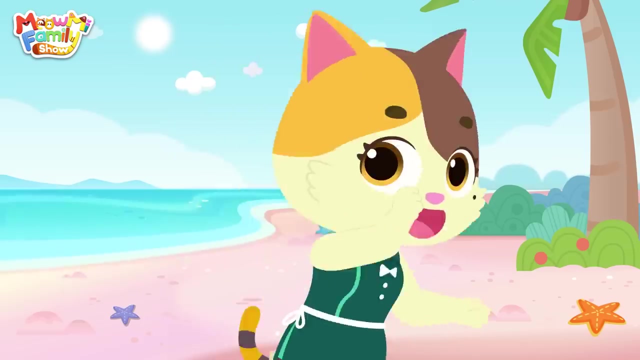 Oh Oh, It's coming. -oh, oh, Oh, Okay, let's take another, because you- it's good, Watch me, Didn't catch any fish today. Aaaaaaah, Huh, It's just a toy shark, Honey, you are swimming pretty fast. 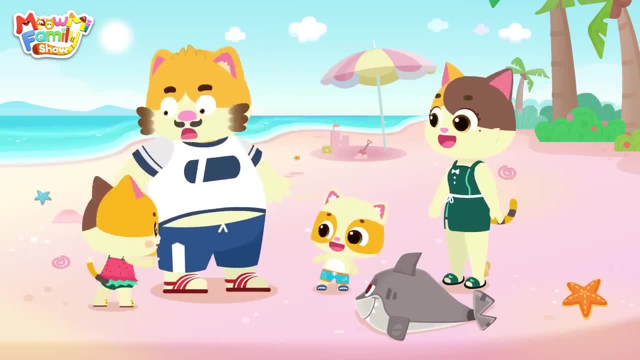 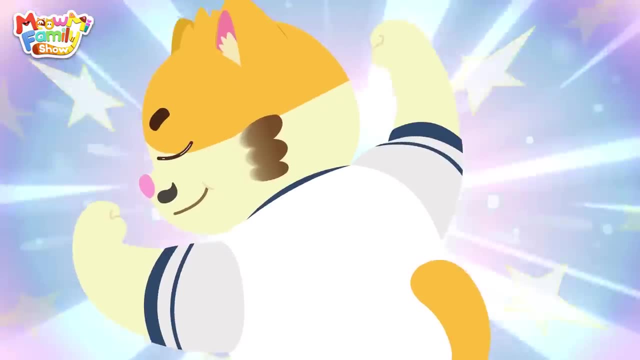 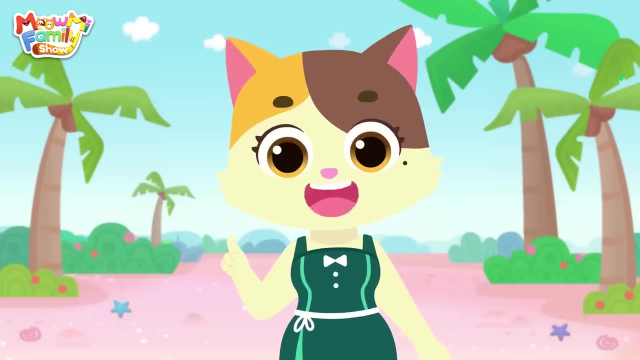 Oh phew, That really scared me. Look, Daddy, Your belly got smaller. What Really I did? lose weight. Exercise really helped me lose weight. Still, you should eat healthy and exercise regularly. Okay, Let's exercise together then. 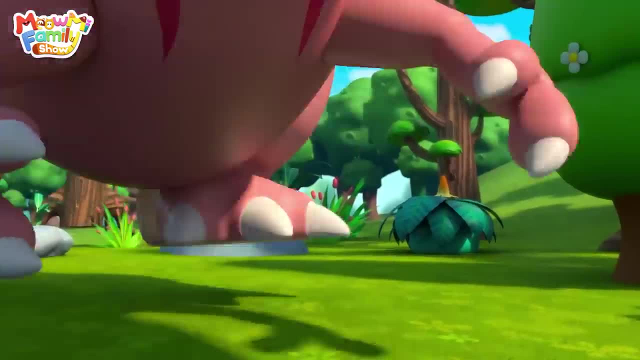 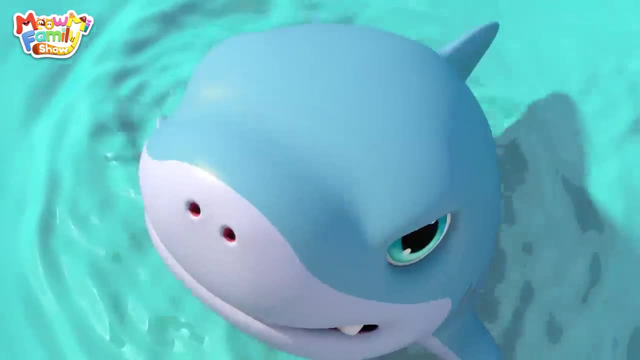 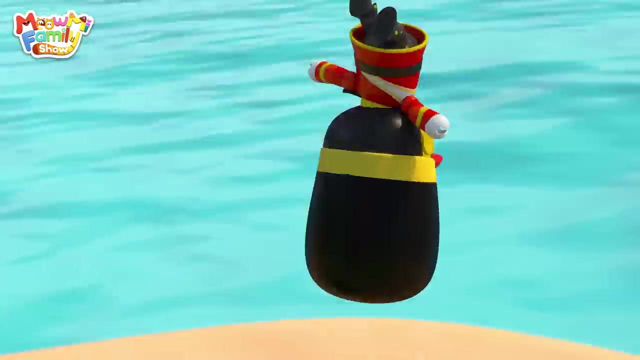 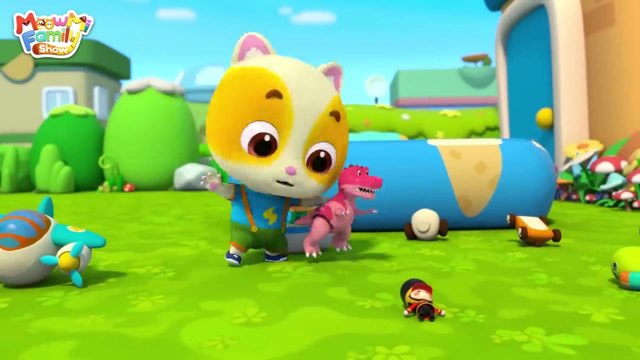 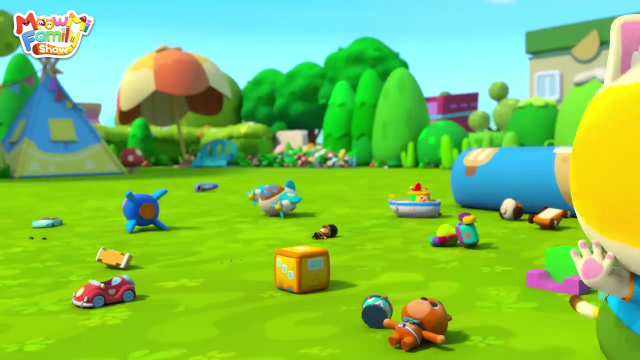 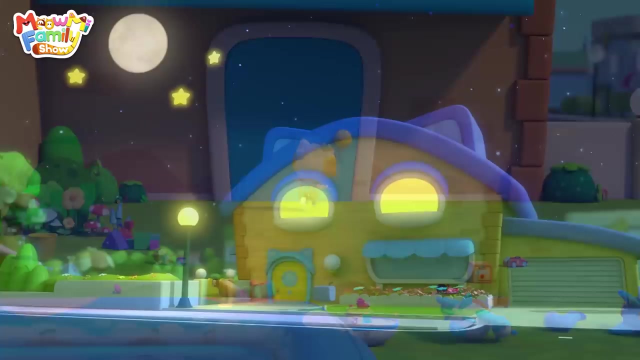 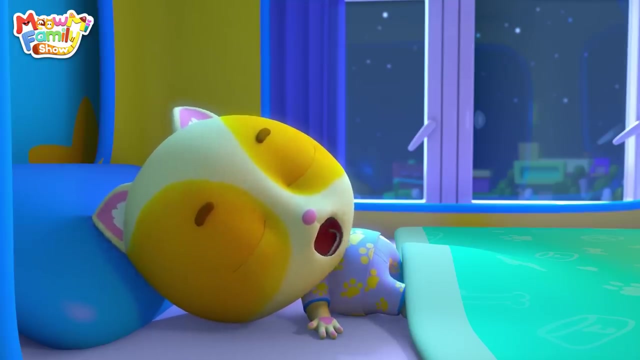 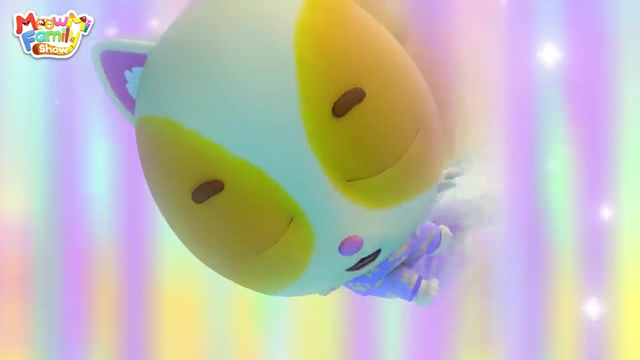 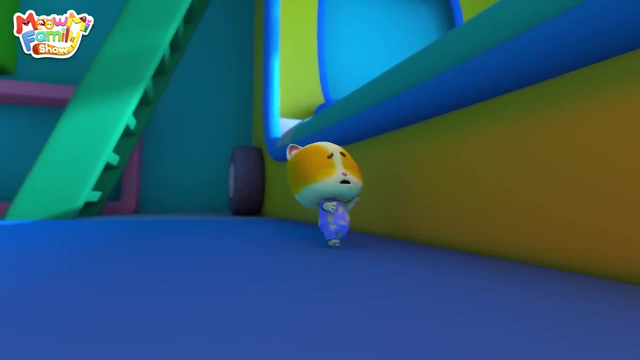 The T-Rex is coming, Run, It's a big shark. Oh, Run, T-Rex is awesome. Timmy, Time for dinner Coming. Phew, I am, I am, Ouch, Ouch, Huh. What's this? 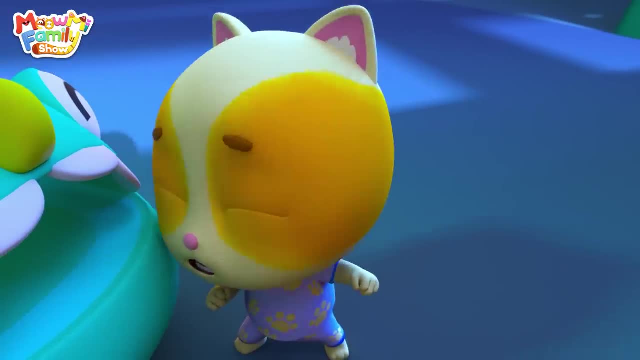 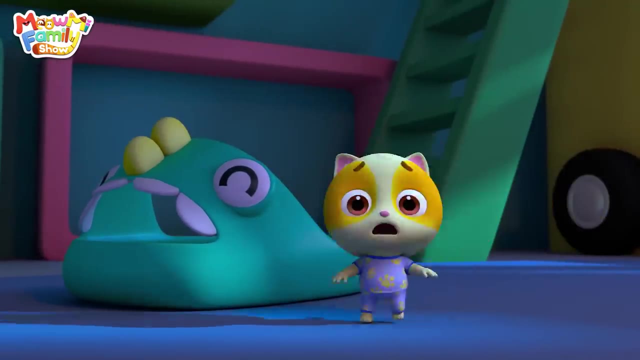 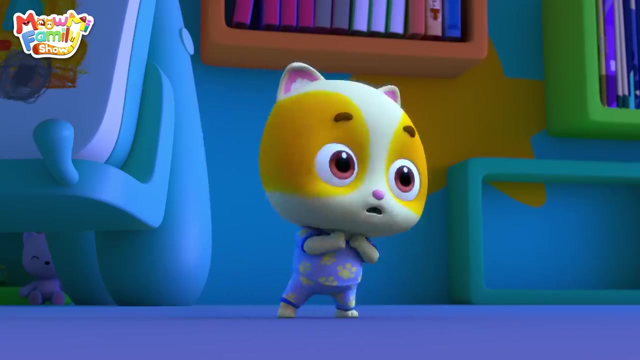 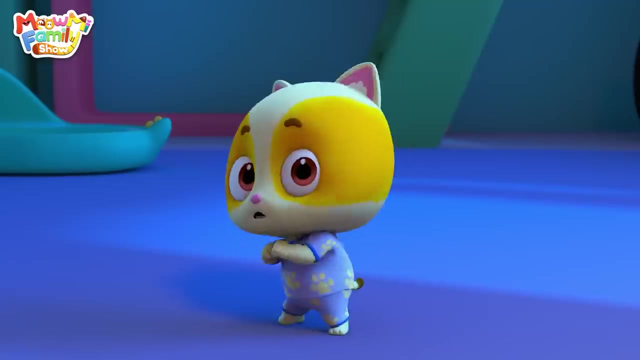 Huh, Why is my bed so big? Huh, And my slippers are so big too. Huh, That's not it, I got smaller. Huh, Huh, It's a drumming bear. What's going on? G-g-go away. 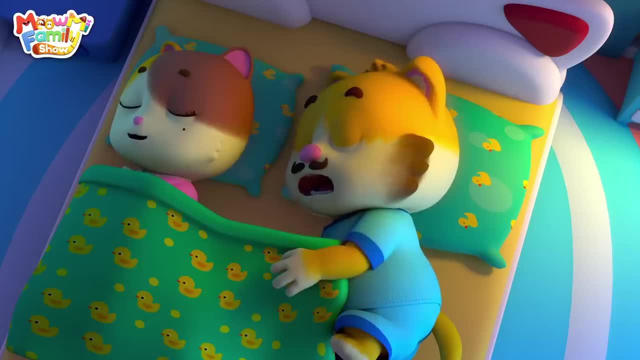 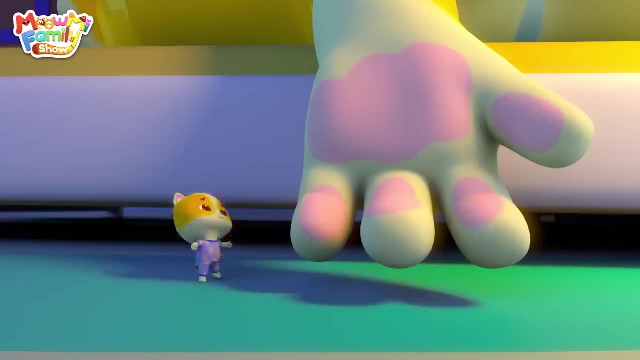 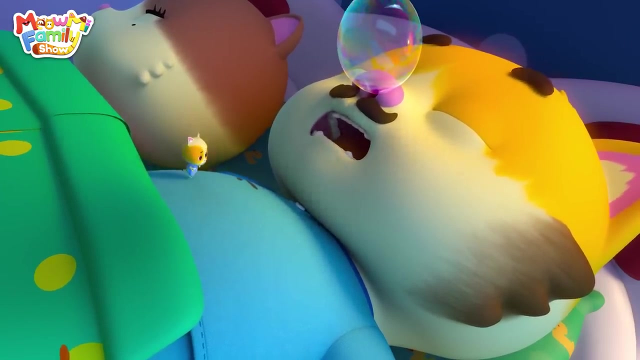 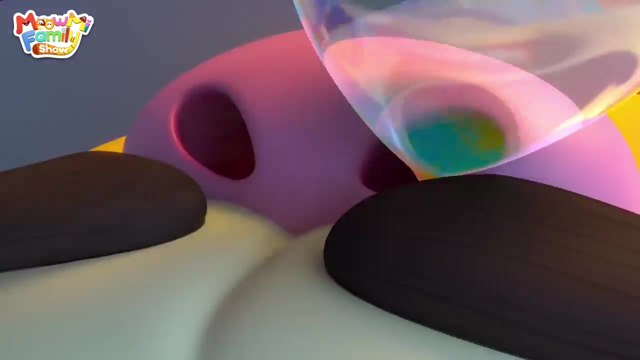 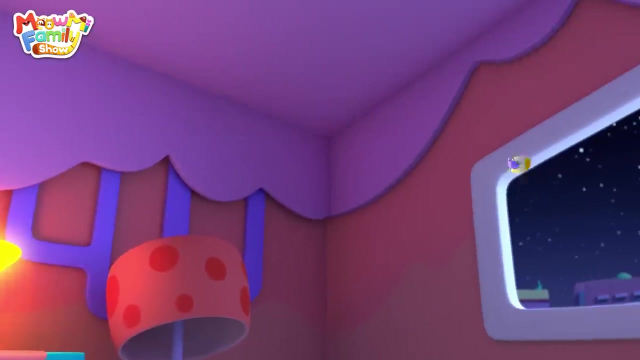 Mommy Daddy, Help me Ouch. Mommy Daddy, Oh, Daddy, Wake up, Daddy, Ah, Come on, Wake up, Stop snoring. Ah Huh, Ah, Ah, Ah, Daddy Ouch. 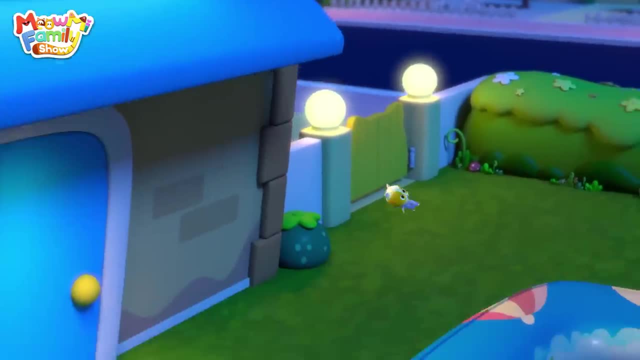 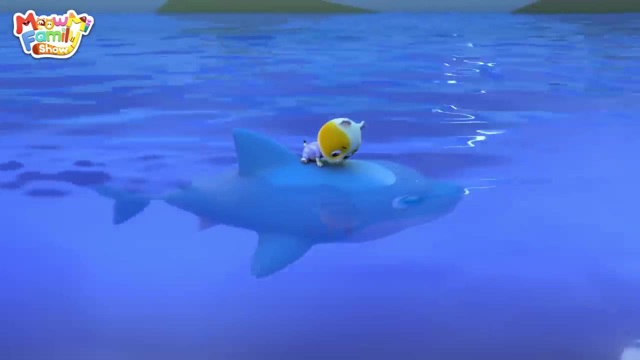 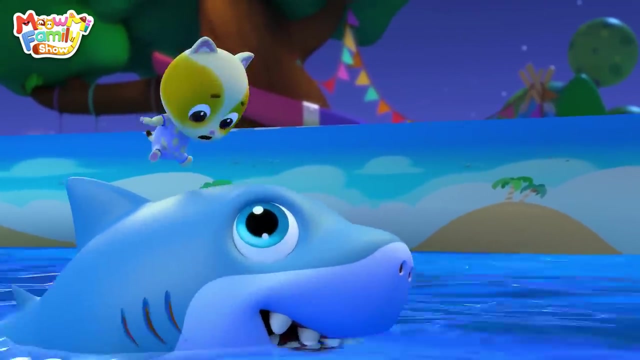 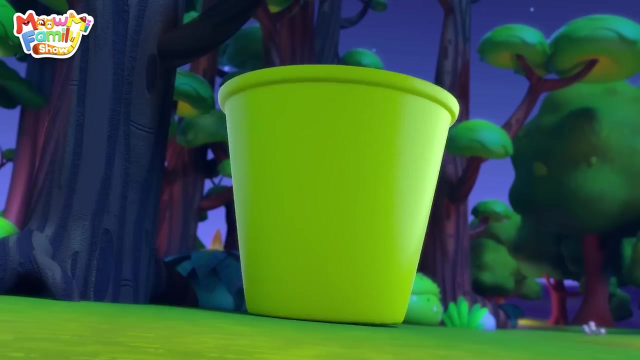 Ah, Ouch, Ouch, Ouch, Oh, help, Somebody help. Huh, What's going on? Huh Huh, Ah, It's the big shark. Don't eat me. Uh Huh, What's that sound? 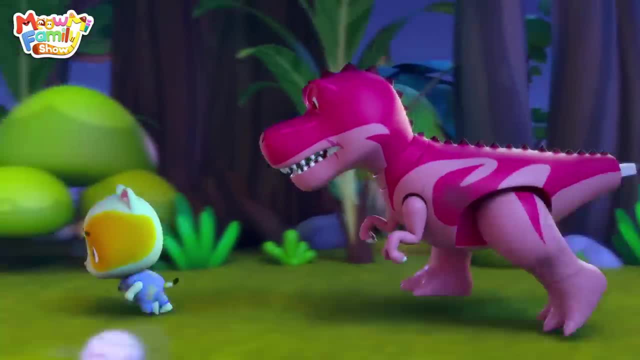 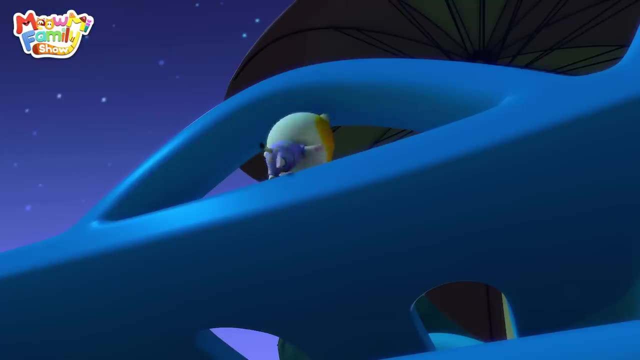 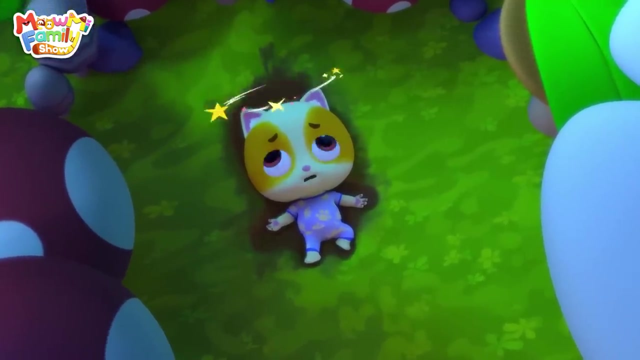 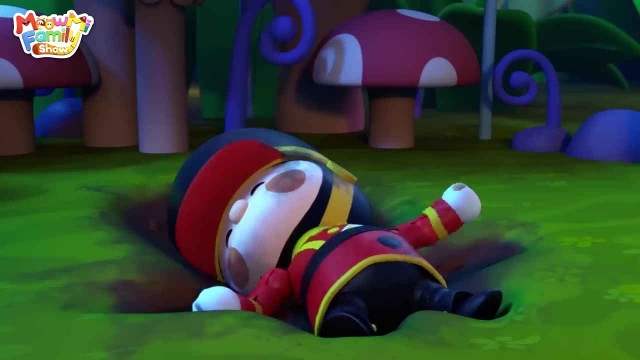 Ah, T-Rex, I didn't mean to break your tail. Huh, Stop following me. Stay, Stay away from me. Uh Ah, that hurts. Huh, Ah. Oh, you were sitting on me. Huh, Stay away from me. 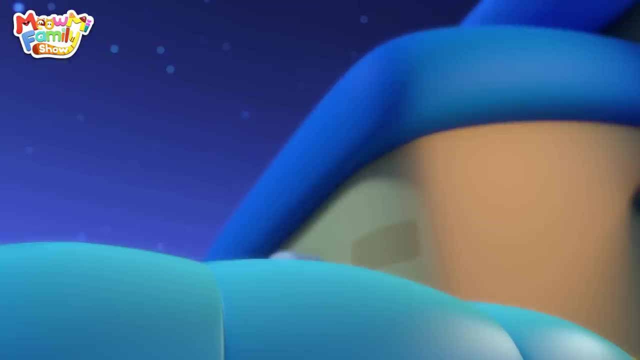 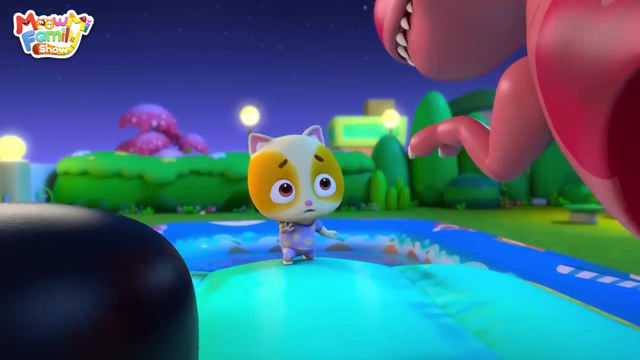 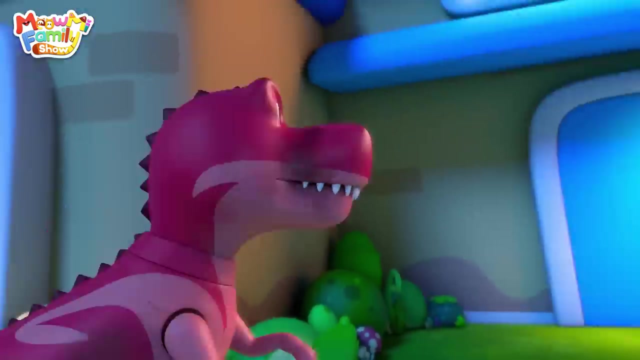 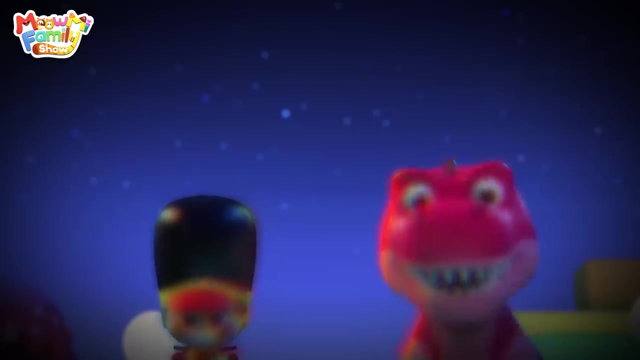 Timmy, Don't run, Huh, Ah, Oh no, I'm stuck, Please, I didn't mean to hurt you guys. Ah, Help me. Ah, Stay away. Stay away from me, Don't be afraid, Timmy. 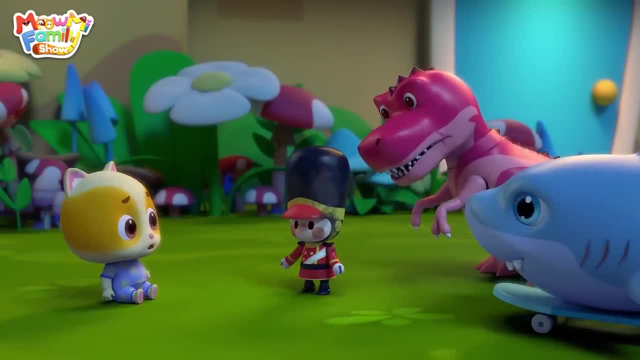 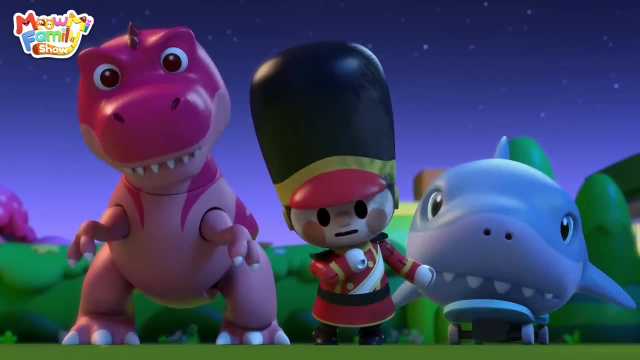 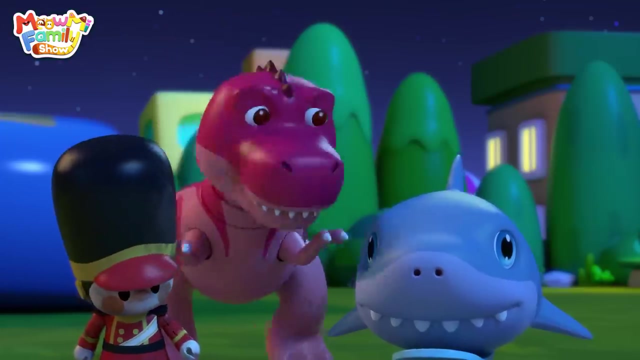 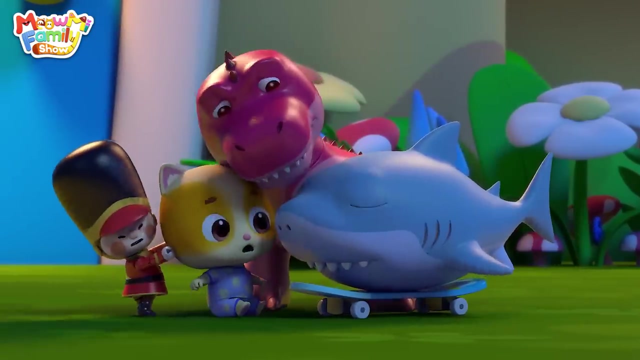 We're here to say goodbye. Huh, Say goodbye, Yes. If our owner doesn't care for us, we'll have to leave. Huh, Where are you going? The train's here. Goodbye, Timmy, We'll miss you. 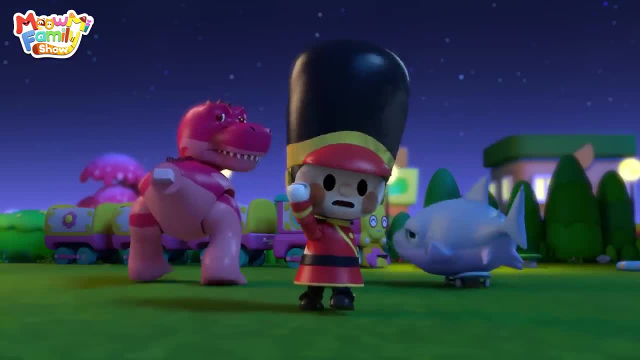 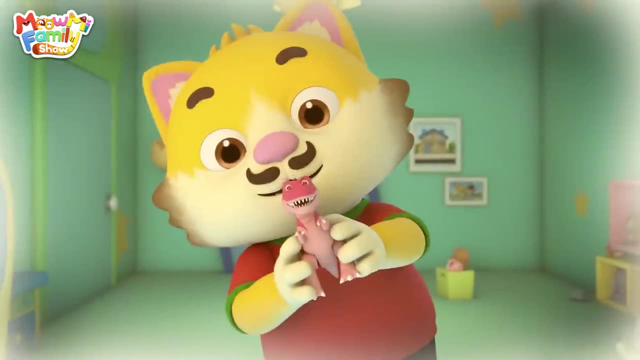 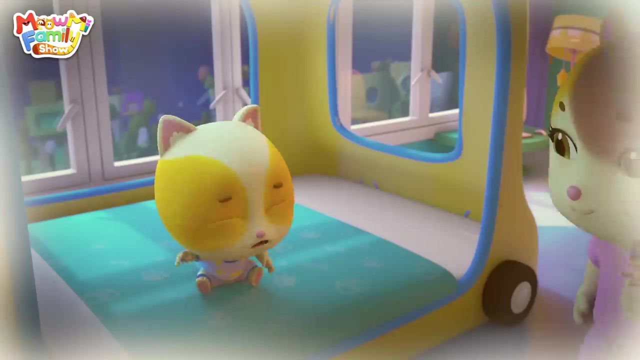 We'll miss you. Uh Goodbye, Uh Uh. Happy birthday, Timmy. This is for you. Wow, It's a T-Rex. Wah, I don't want to sleep alone. Look who's here for you. 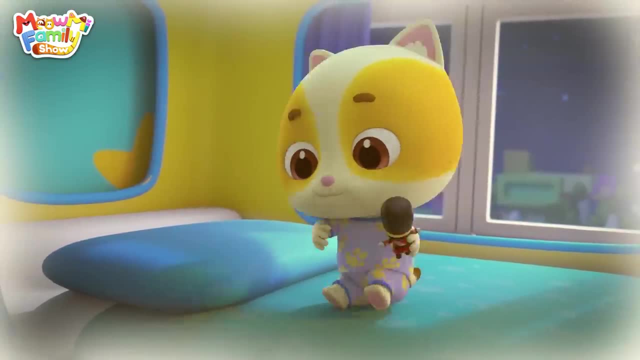 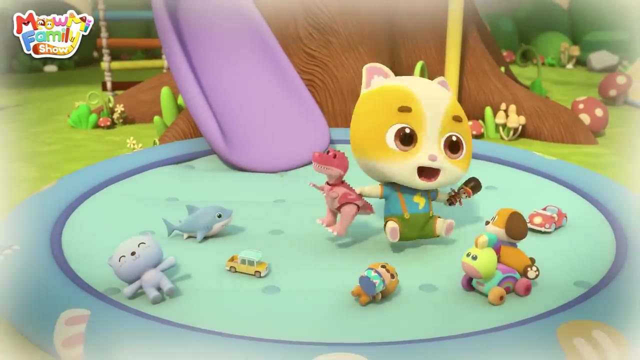 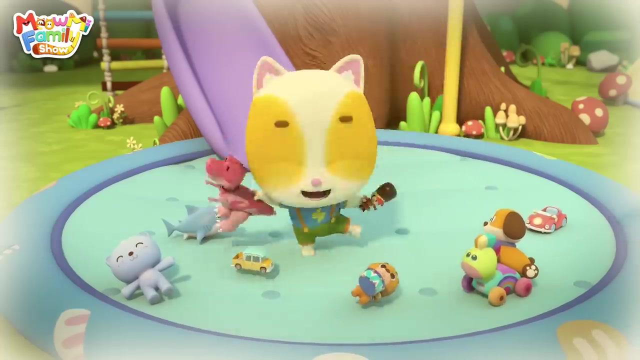 Ah, My little soldier, Time for bed, Good night. Whoa Ha ha ha, Youhoo Ha ha ha, Hey, hey, hey, My big shark and drumming bear. I love you guys so much. 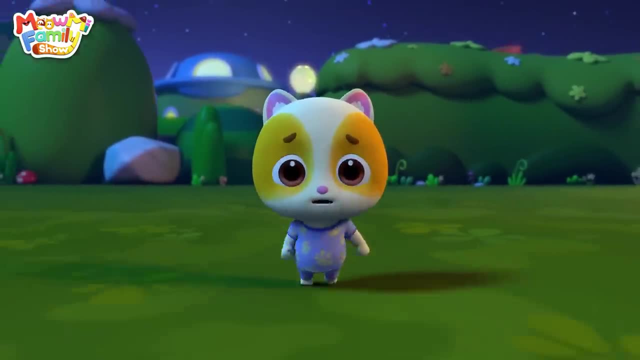 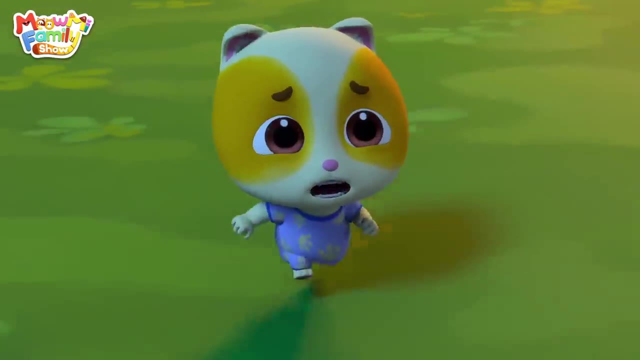 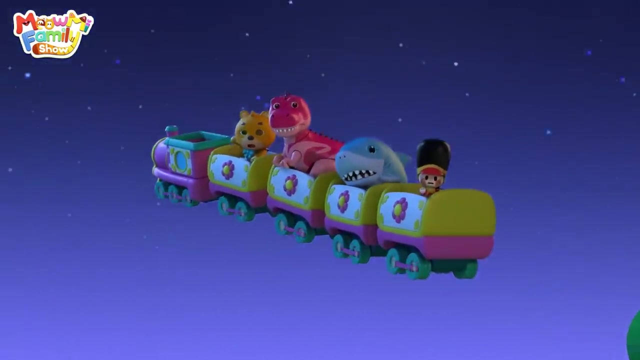 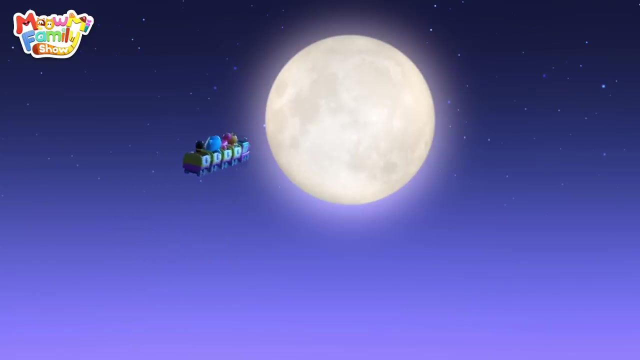 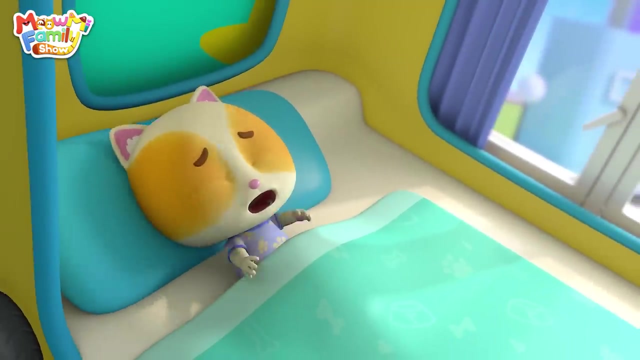 Little soldier, T-Rex, Big shark, Drumming bear, Don't go. Ah Huh, Timmy Timmy, Don't leave me. Ouch, Don't go away. Timmy Timmy, Did you have a bad dream? 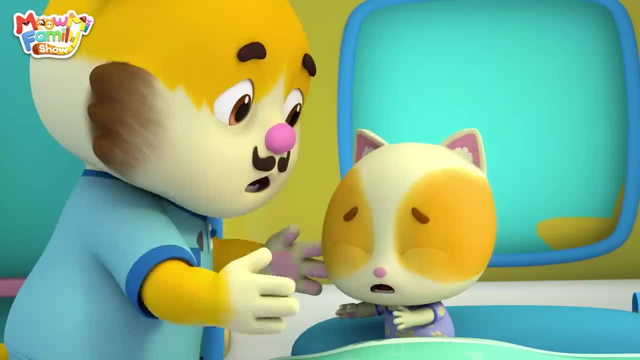 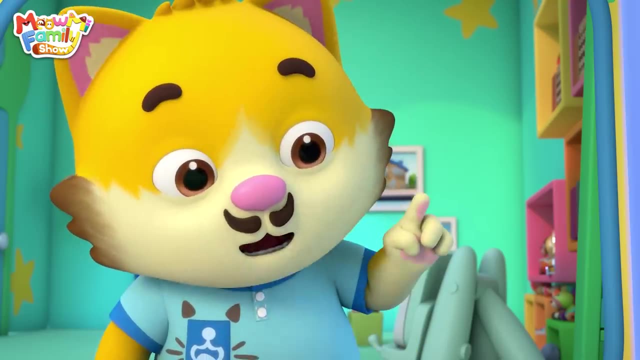 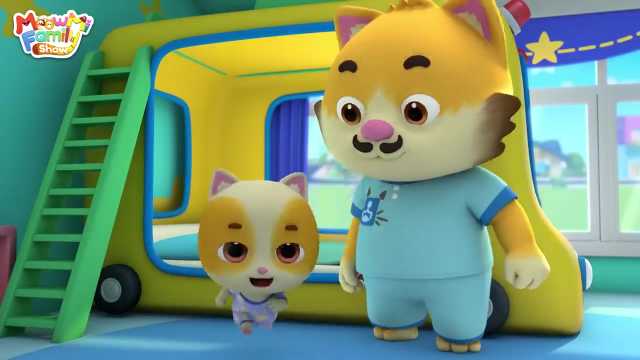 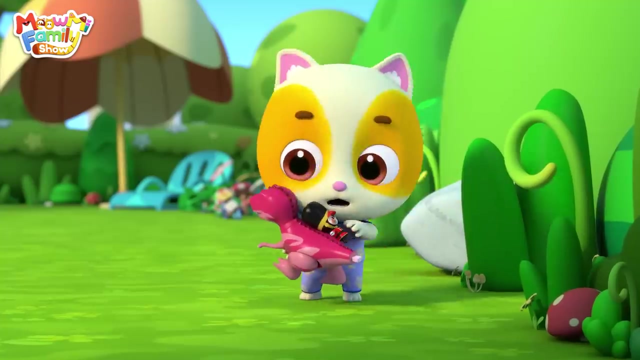 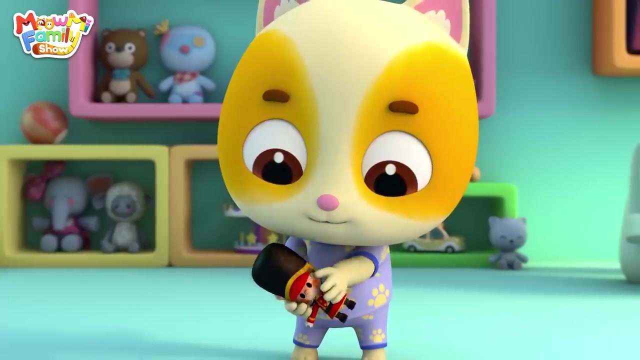 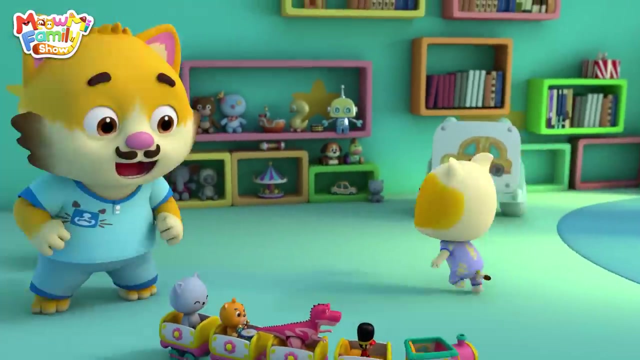 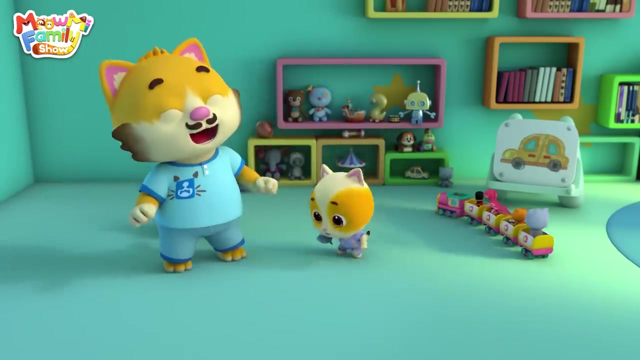 Daddy, my toys all left me because I didn't care for them. Then let's care for them from now on. It's all finished. It's all finished And all clean. Yeah, I'll take care of you all forever, Wow. 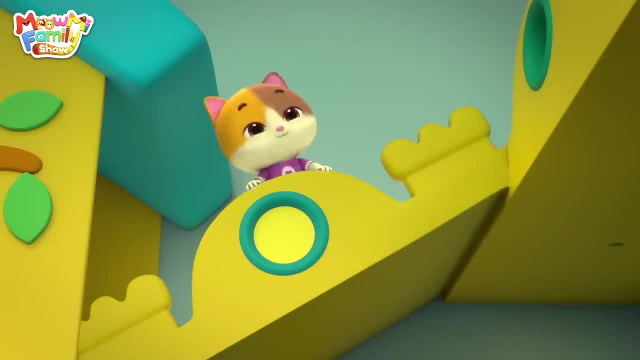 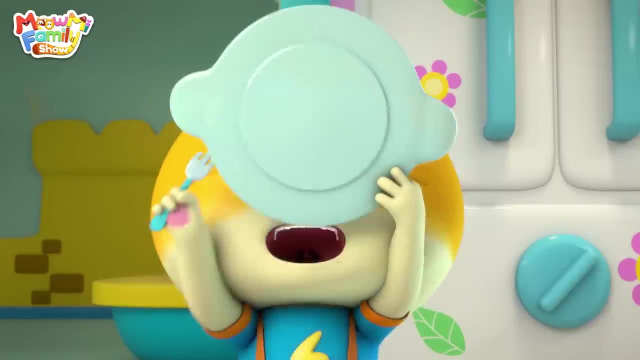 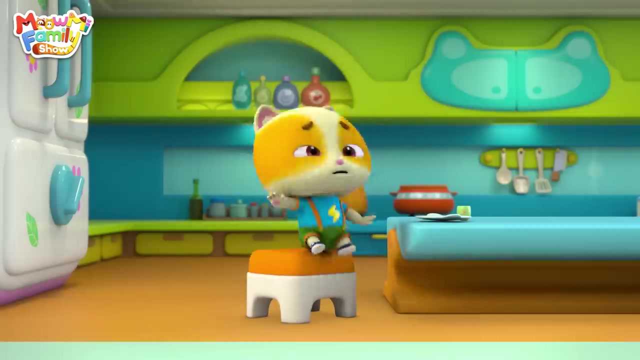 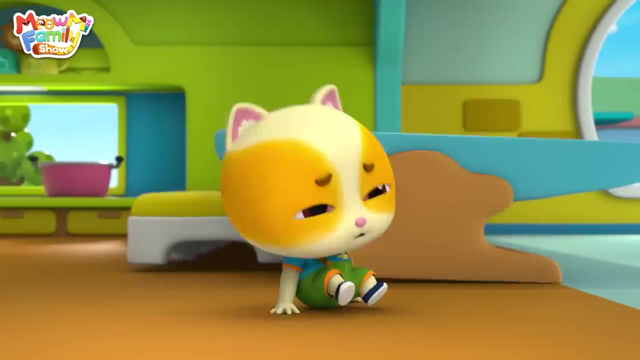 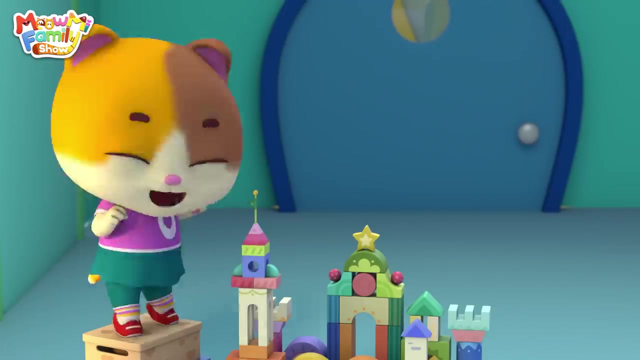 Timmy, Timmy, Come on up, Let's build a castle. Okay, after I'm done eating. Ah, Why am I hiccuping? Stop, It doesn't stop. Wow, My castle looks so awesome, Mimi, Mimi. 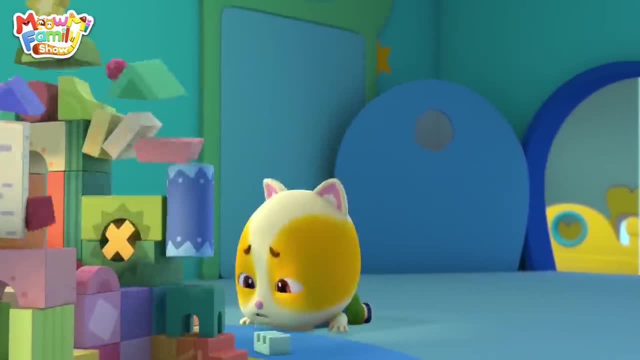 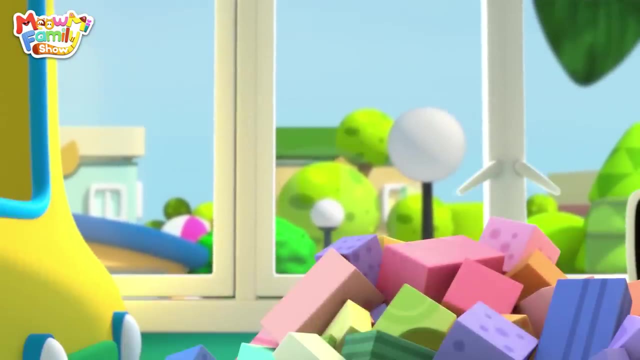 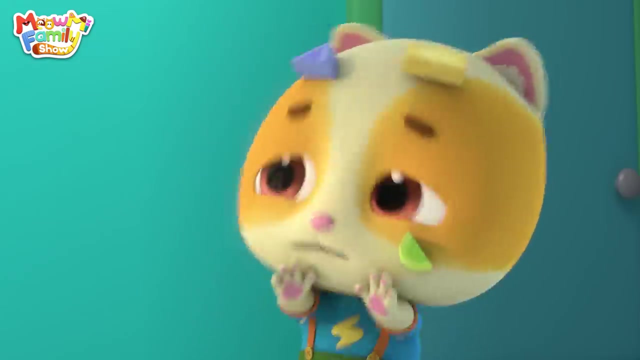 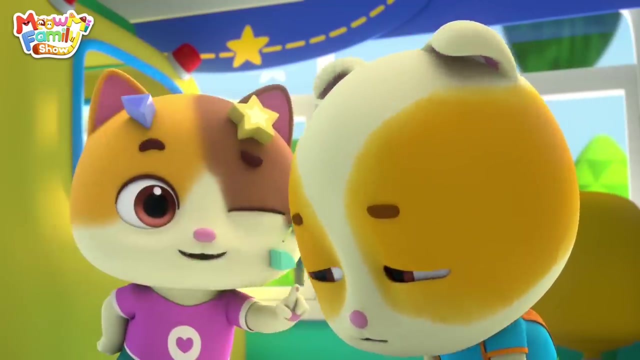 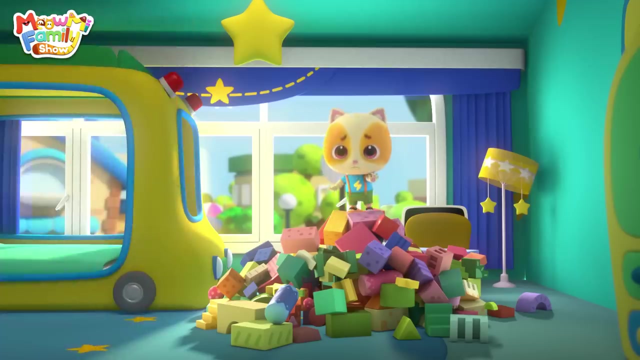 Mimi, Mimi, Mimi, Wow, Ah Ouch. Oh, Timmy, I'm sorry I just hiccuped. I didn't mean to break. it Looks like you need my help now. Mimi, Mimi, Where…? 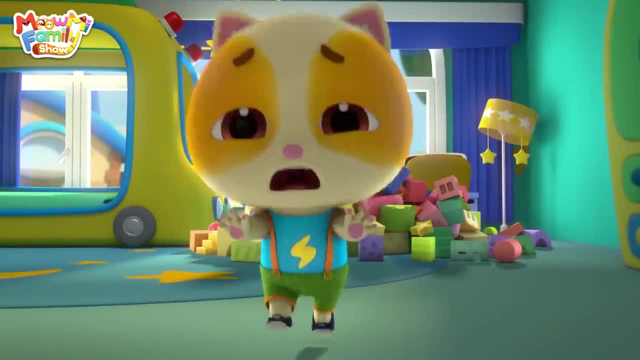 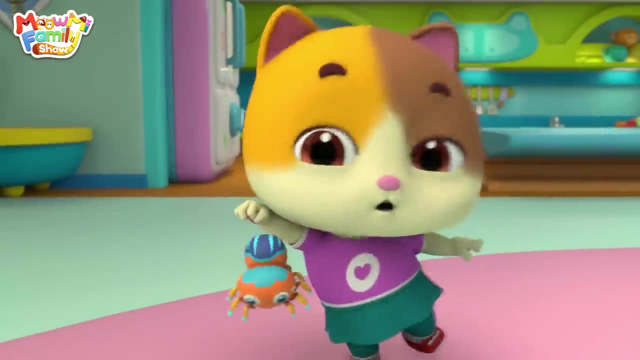 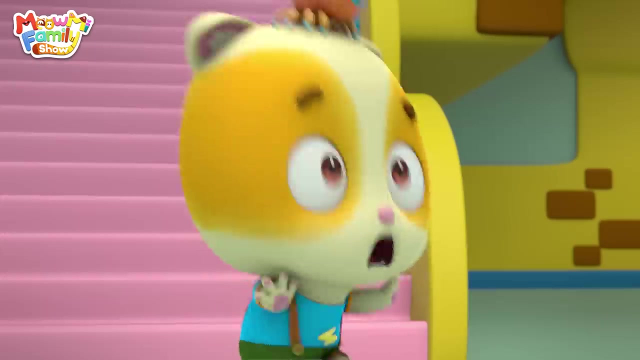 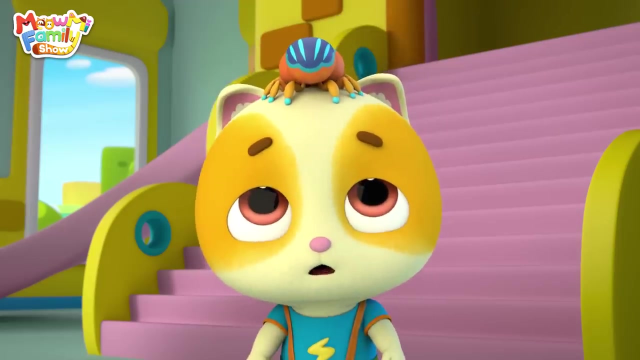 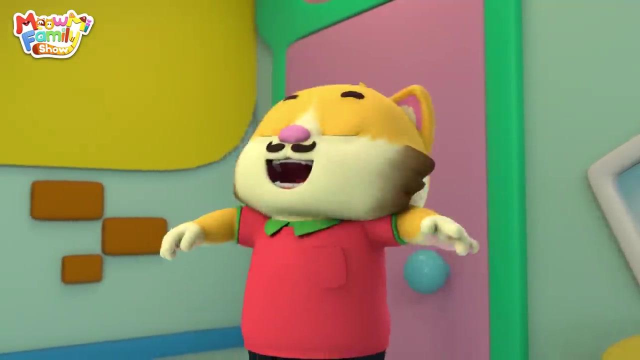 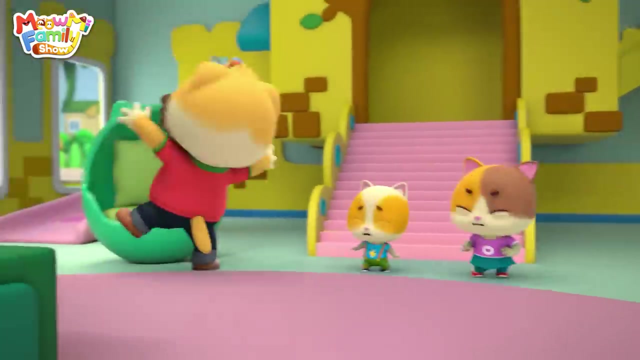 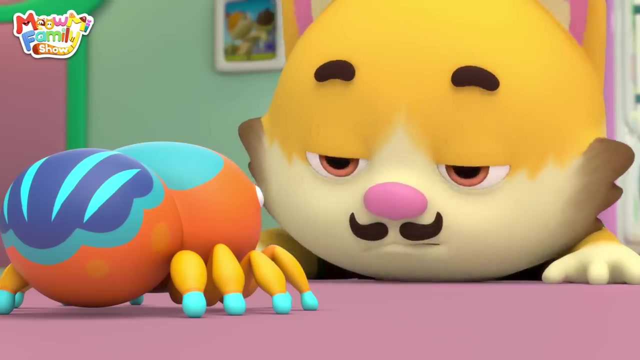 Where are you going? Mimi Timmy, did you stop hiccuping? No, Huh, Isn't it supposed to stop? when you're surprised Spiders, don't surprise me Huh. Spider, Spider, Spider, Huh. 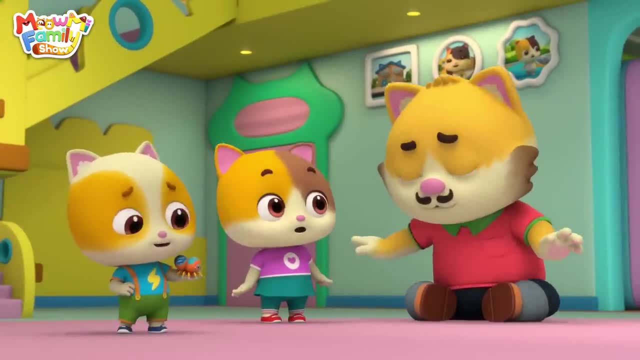 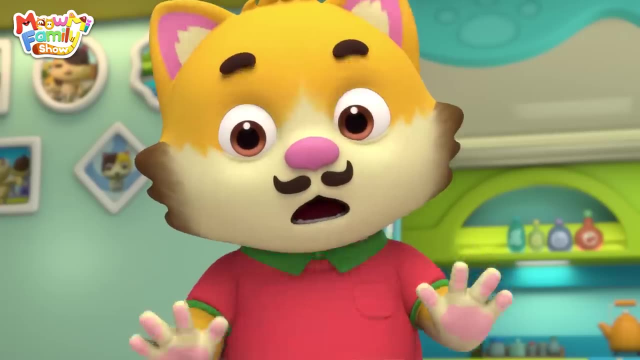 Huh Huh, Is it fake? You scared me. I'm sorry, Daddy, I was just trying to help Timmy stop hiccuping. Huh, Huh, Huh. You know what? I have a good idea. 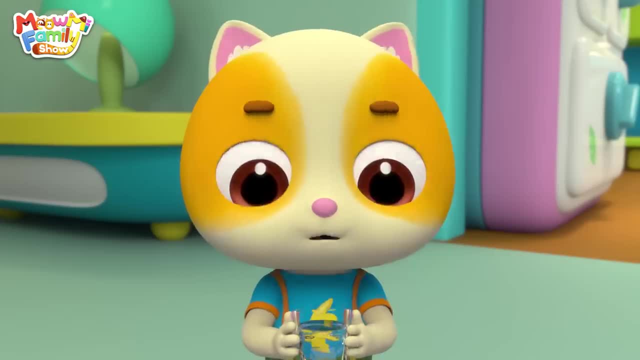 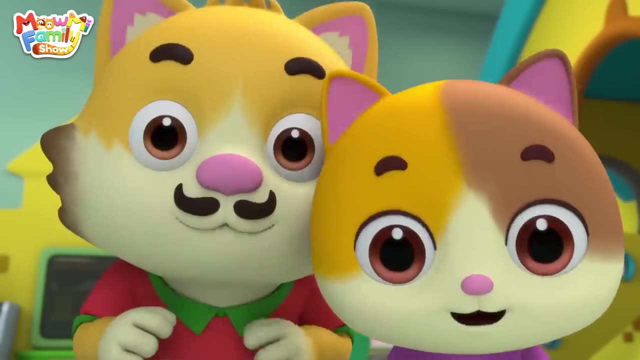 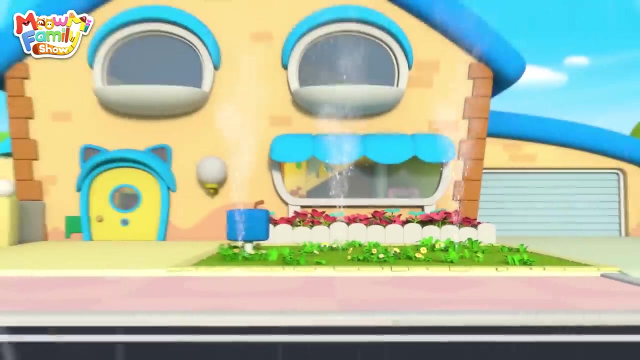 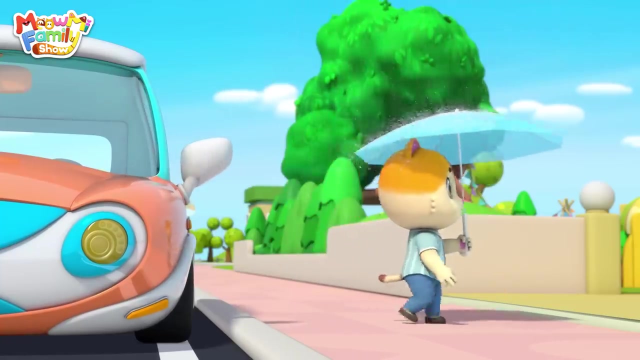 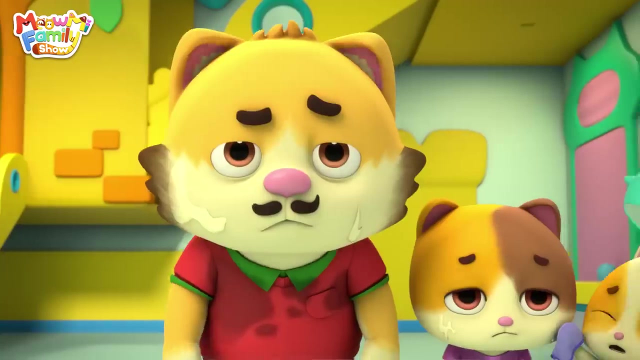 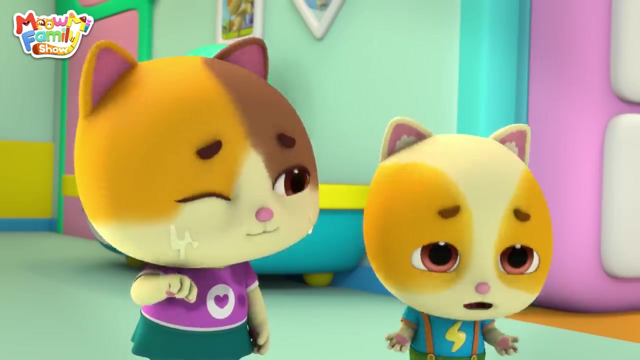 Drinking water can stop the hiccups. Try it. Uh-huh, How do you feel? Did it work? Uh, What's going on? Good thing I brought my umbrella. What strange weather. Why are you all wet? Because I hiccuped. 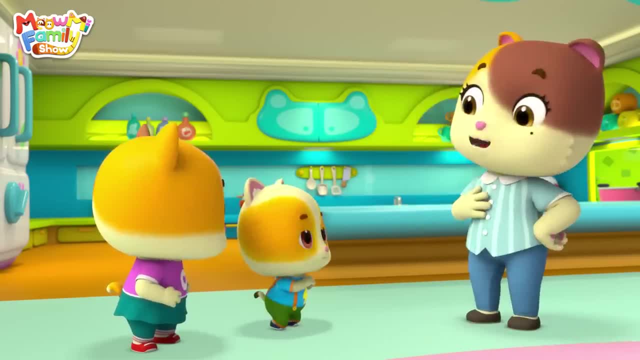 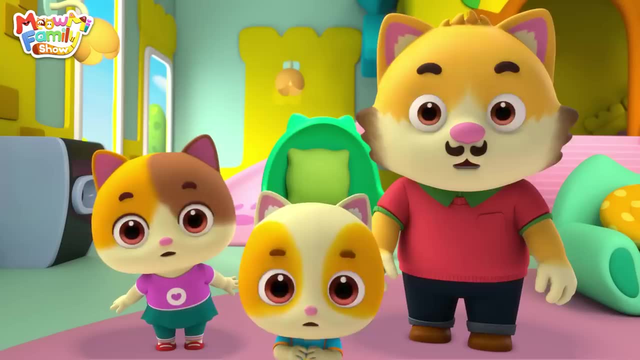 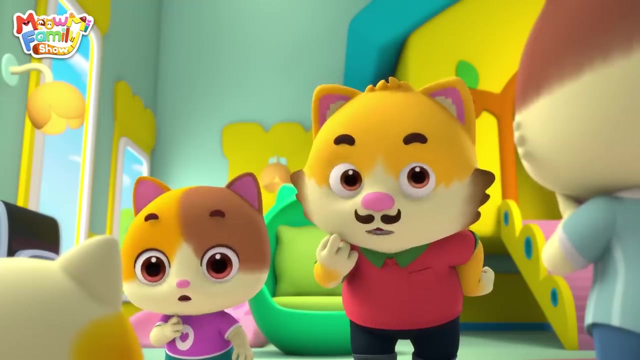 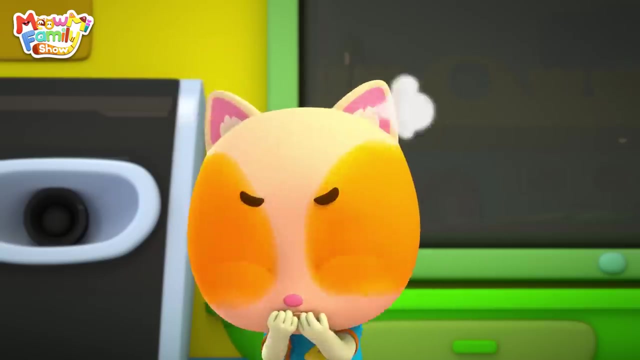 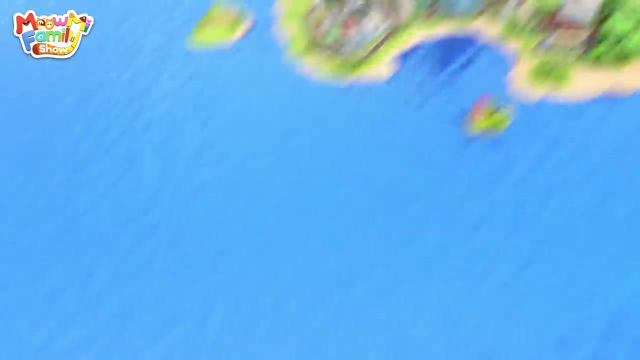 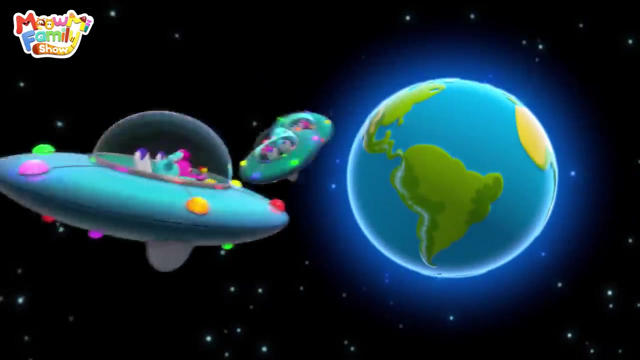 Oh, Hmm, Ah. I have a good idea to stop your hiccups. First take a deep breath, Like I do, Breathe in And then Hold it. Good job, One more second, Ah, Ah. 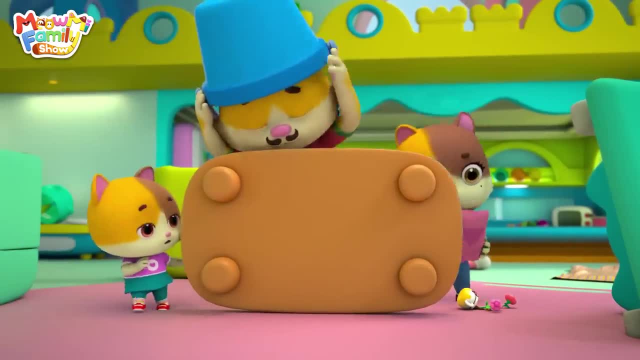 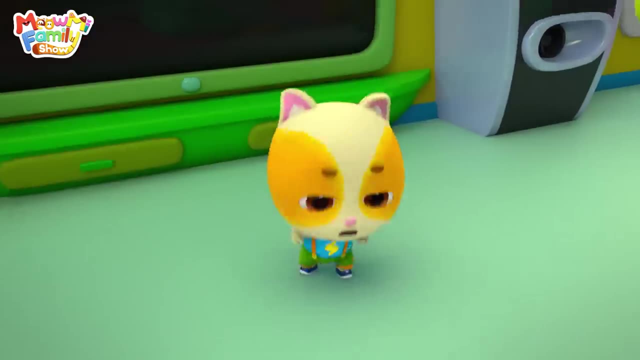 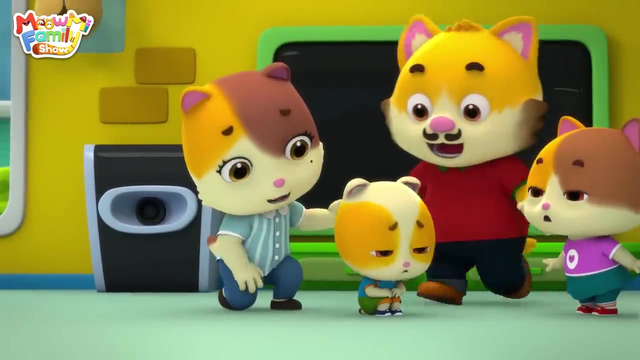 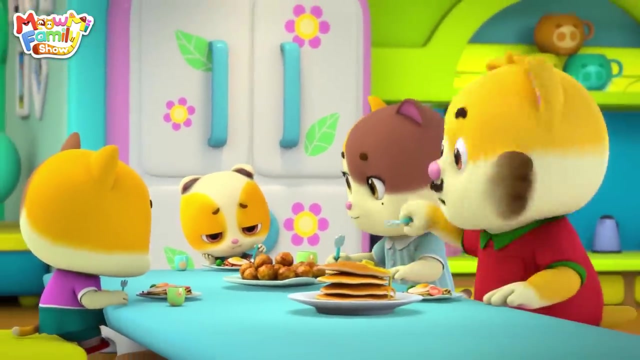 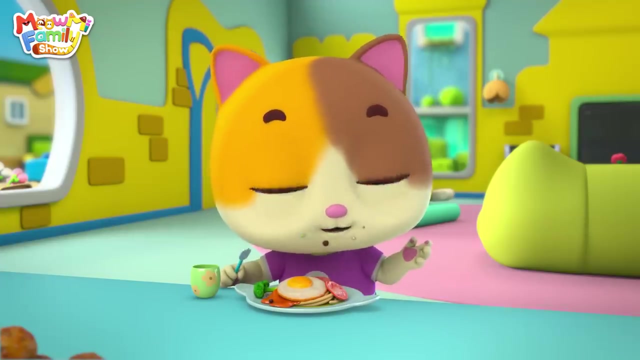 Timmy, did it stop? Let's eat something first And then think of what we can do. That's right, We're all hungry. Oh, come on, Timmy, have some. Yeah, you might feel better. That's right, It's so yummy. 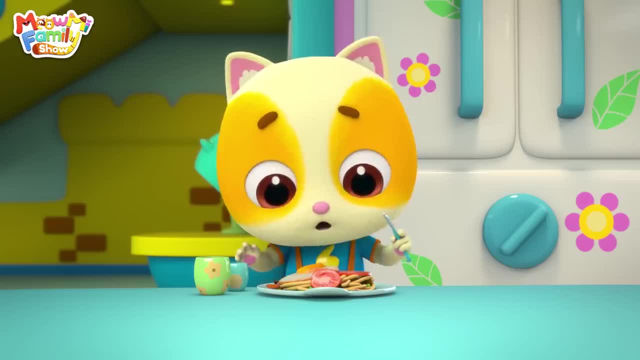 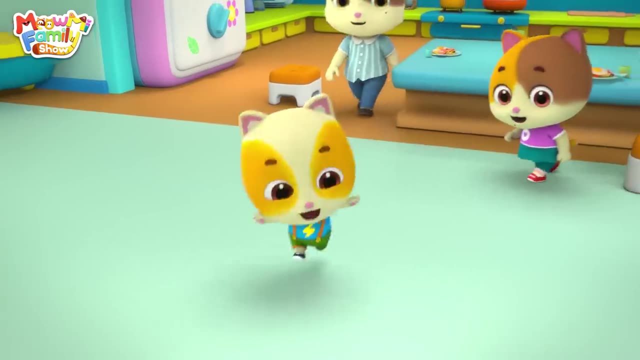 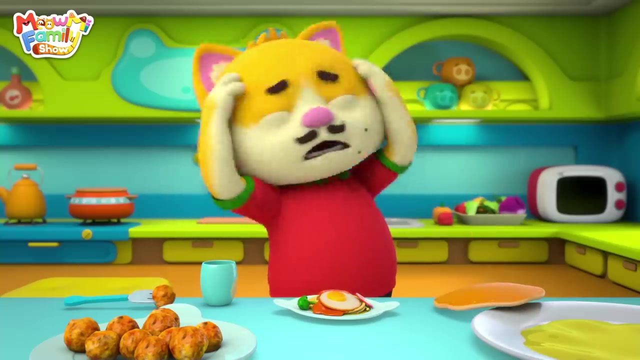 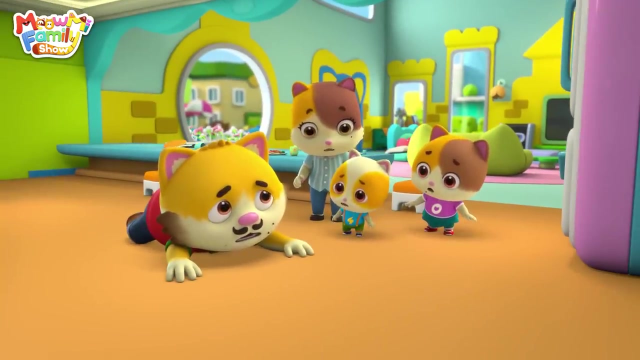 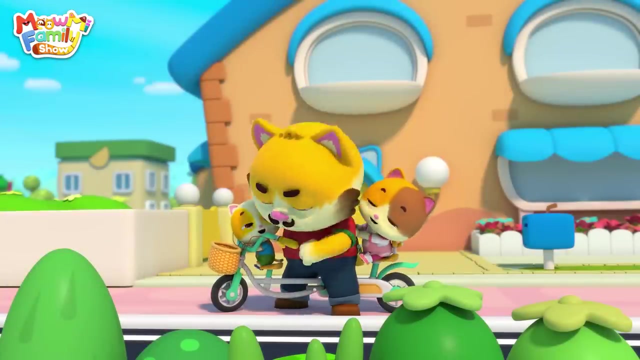 Timmy, you stopped hiccuping. It stopped, It stopped. What's going on Now? Daddy's hiccuping? Daddy, you should eat slowly or you'll hiccup. Mimi Timmy, are you ready? We're ready. 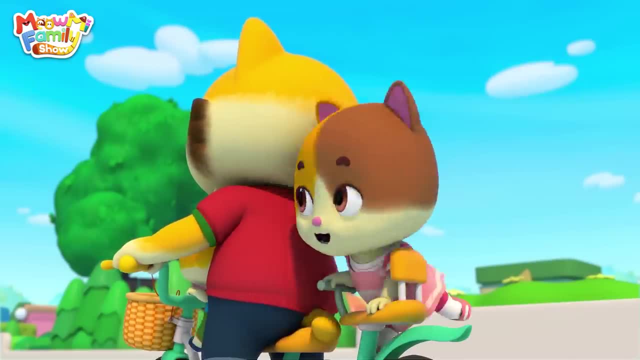 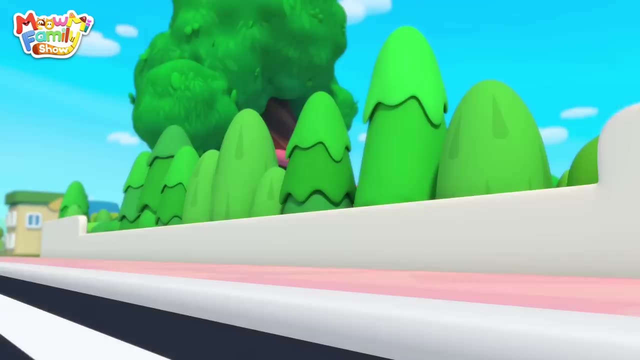 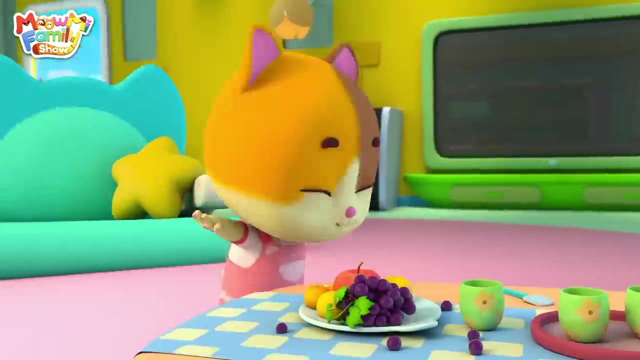 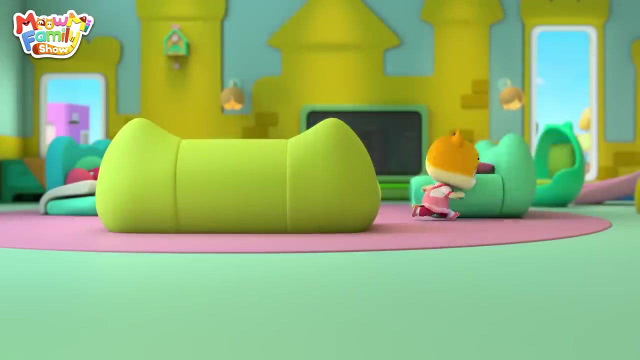 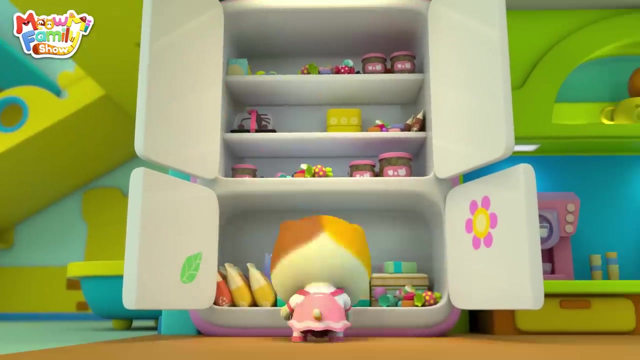 All right, let's go, Go, go, Bye-bye. Yay, Finally I'm home alone, I can do whatever I want. Yoo-hoo, Wow, Wow. Yeah, I can eat snacks while watching TV. 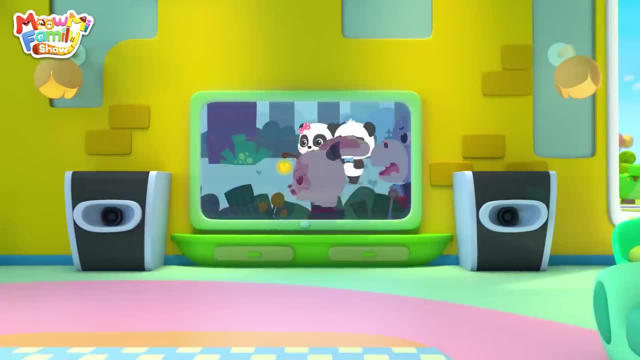 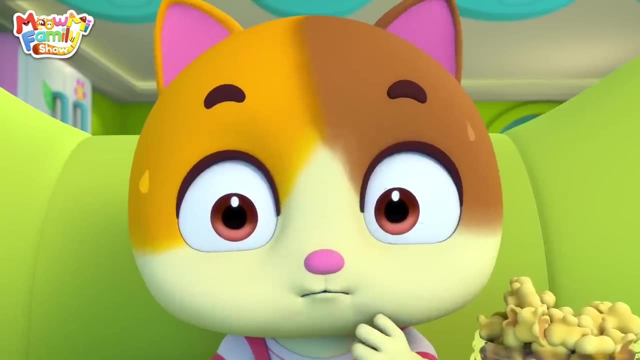 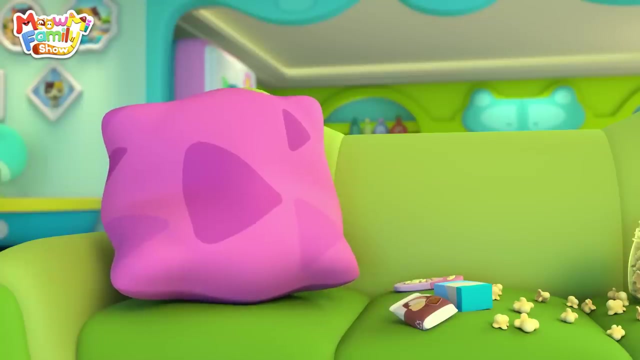 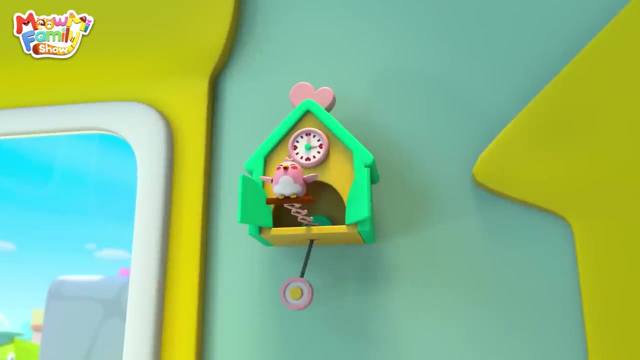 Heh, heh, heh, Hmm, Hmm, Uh, Mmm, Ummmmmm, Huh, Ahhh, Ahh, Uh, Aha, Huh, Huh, Huh, Huh, Ah, Phew. 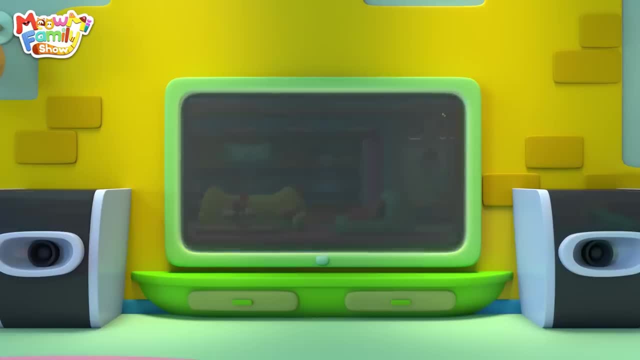 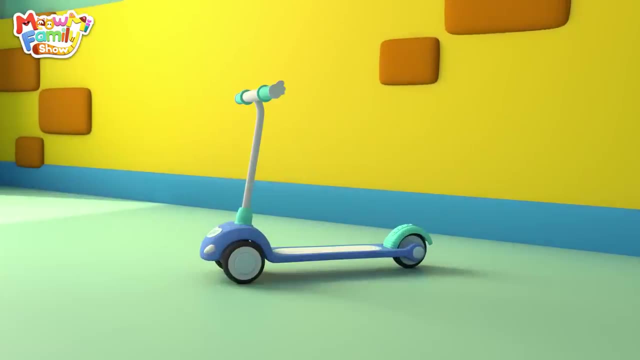 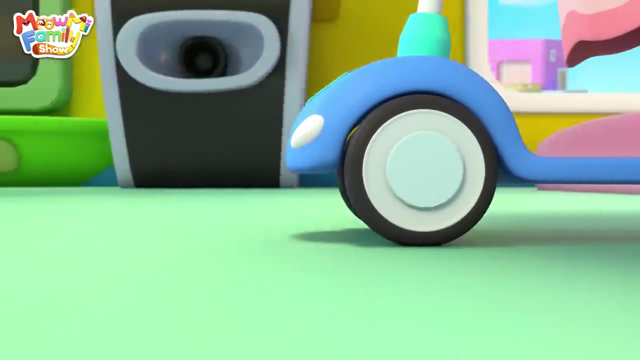 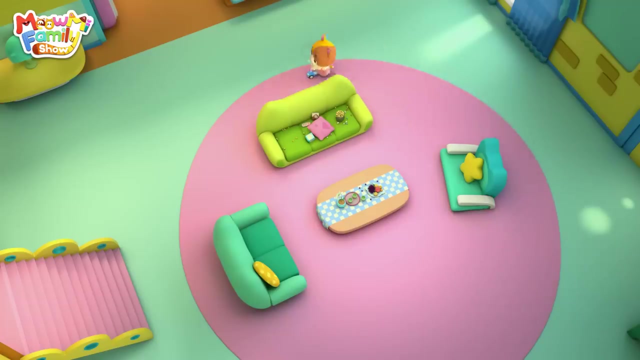 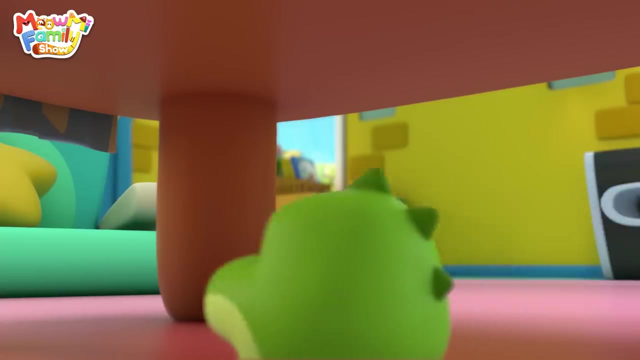 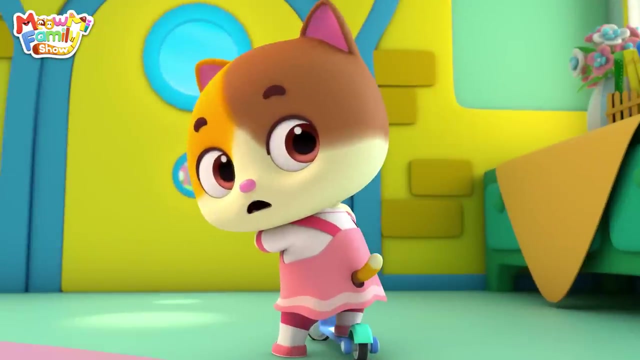 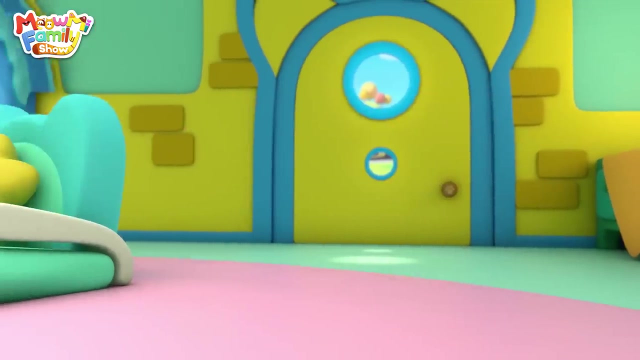 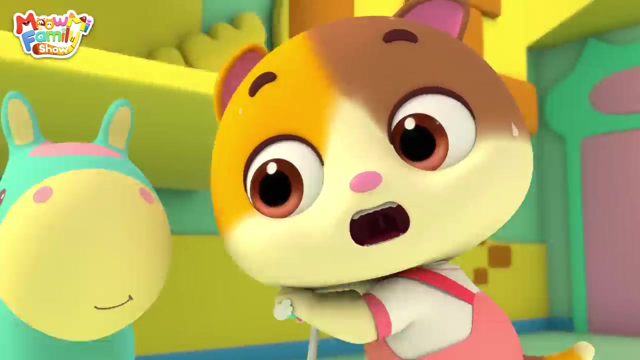 It was just the clock That scared me. Well, I'm gonna ride the scooter. Wow Woohoo, Make a turn. What was that? Uh, uh, uh, Uh, uh, uh. Ah, Ow Huh. 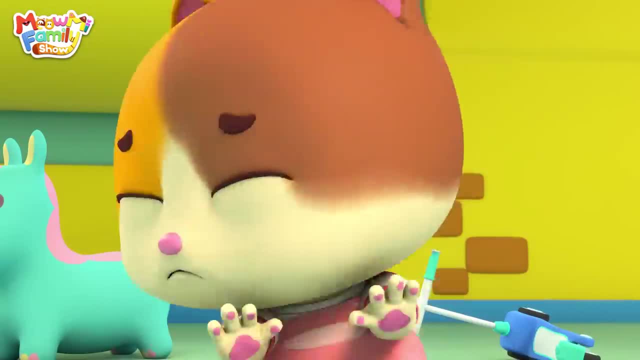 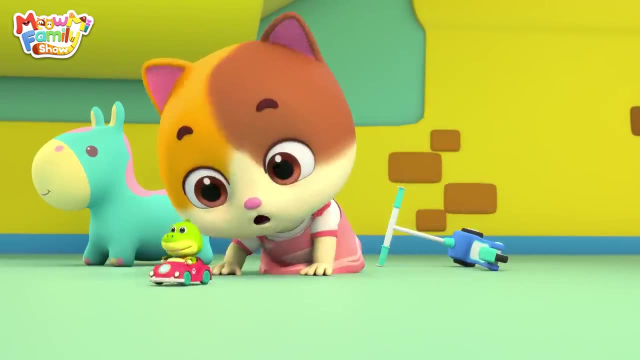 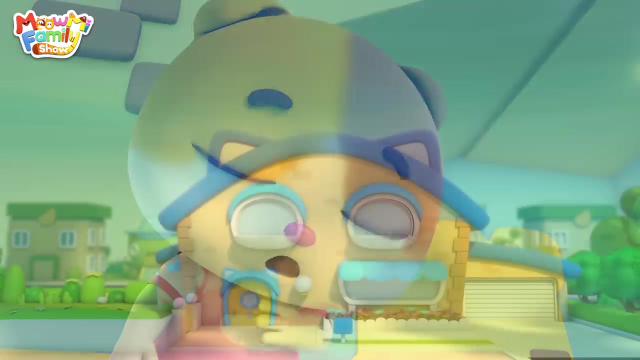 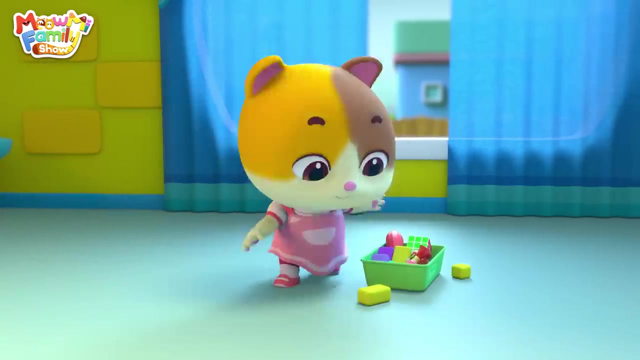 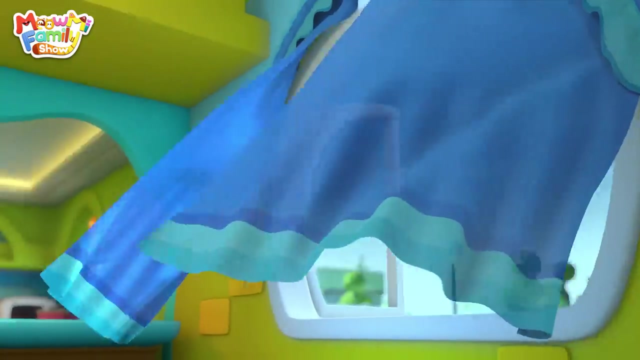 Huh, A monster Go away. Huh, Huh, Huh. Phew, It's just a toy car. Hehe, Let's build a castle. Hehe, Hehe, Hehe, So itchy Timmy stop. 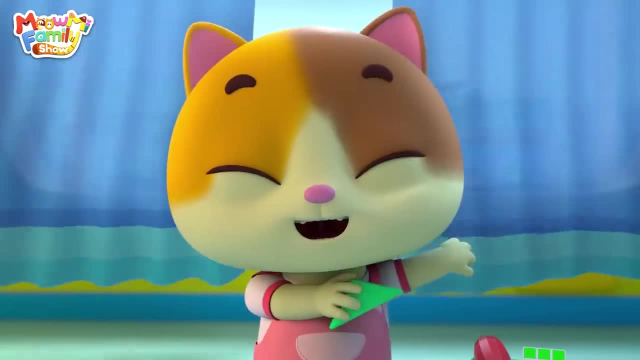 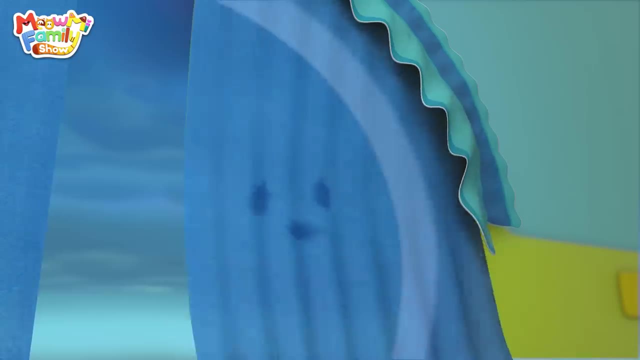 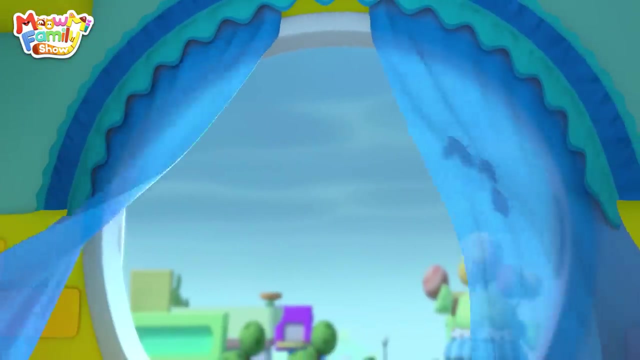 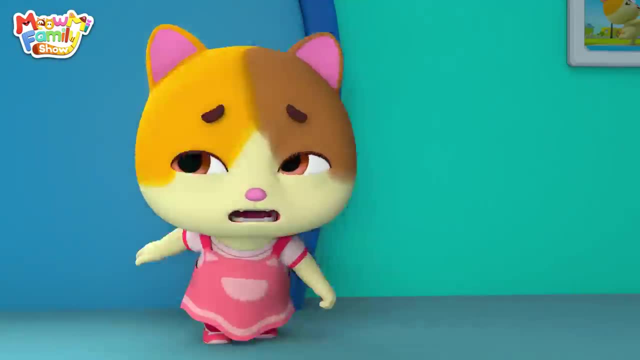 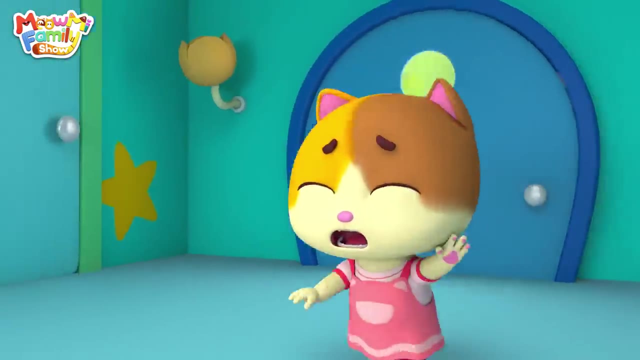 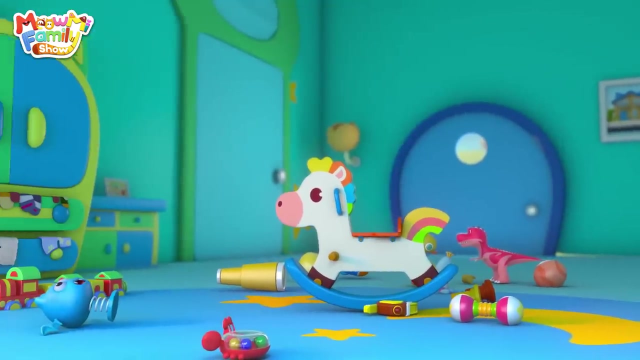 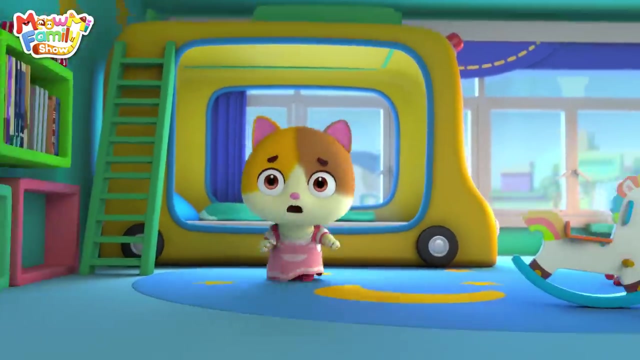 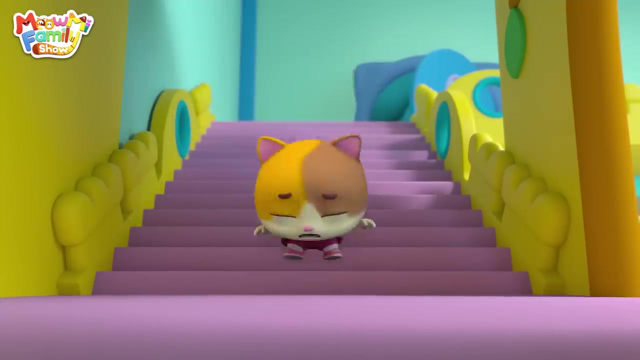 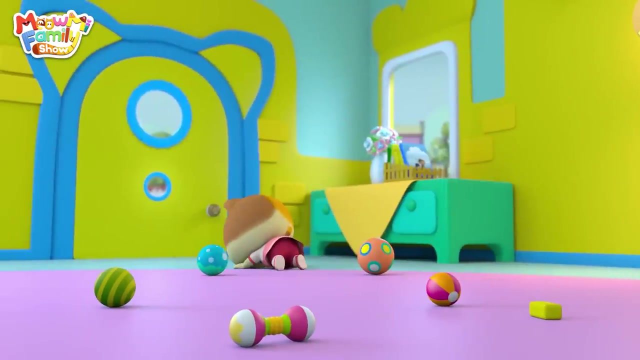 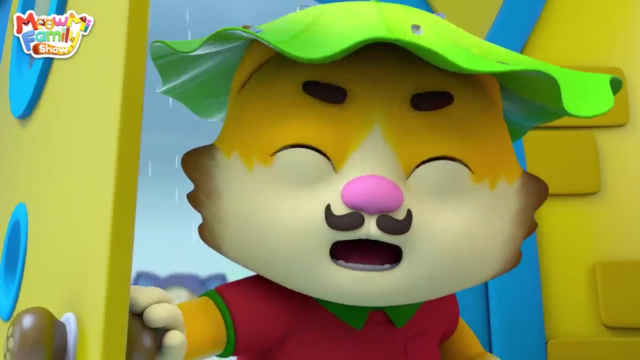 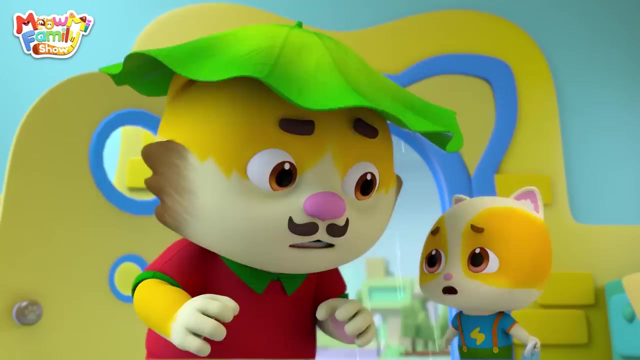 Ah, Ow Ah, Go away. Mommy. Daddy Timmy, come back. I don't like being home alone. Ouch Ah, Go go away. Mimi, You're home. We were so worried. We were worried about you and we're looking for you. 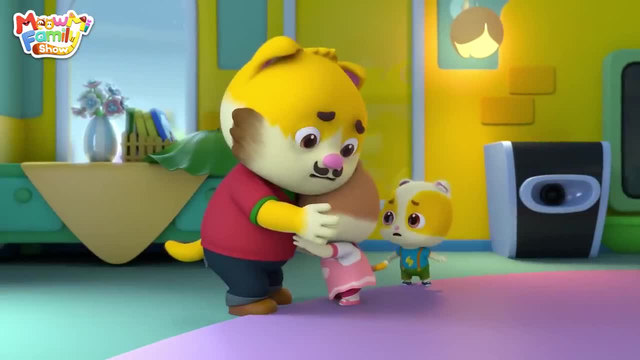 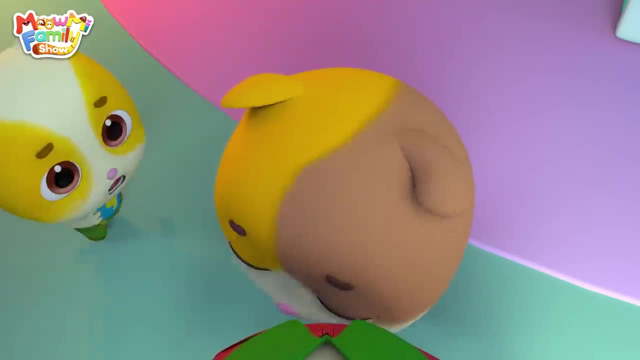 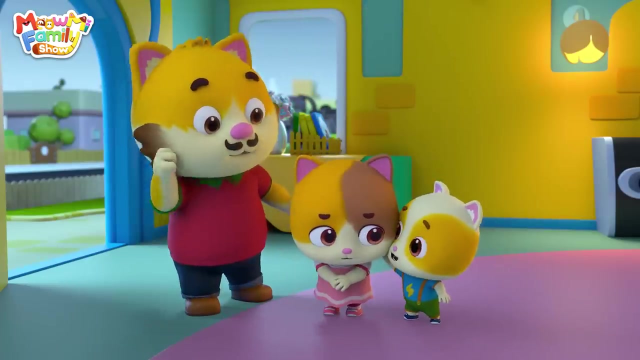 Daddy, Daddy, Timmy, Mimi, It's so scary being home alone. I like being with you guys more, Mm-hmm. So do we From now on, tell Daddy before you go somewhere? It's dangerous for kids to be home alone. 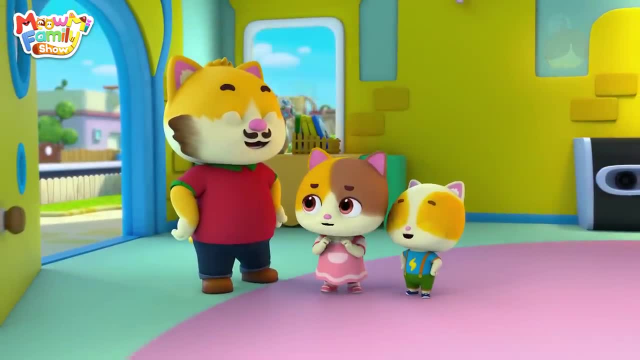 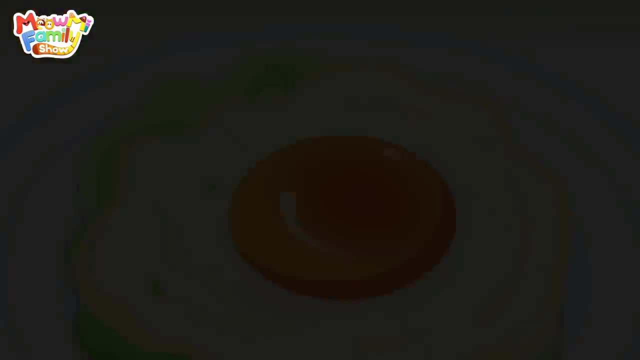 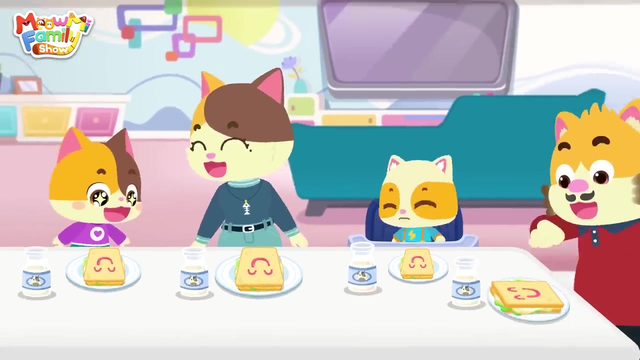 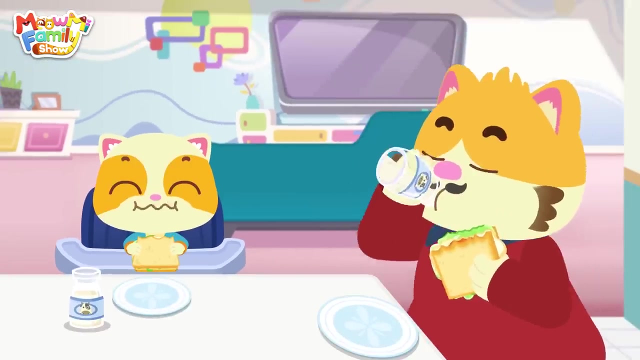 Uh-huh, I'll never do that again. Ha-ha-ha, Mm. Time for breakfast. Wow, Ha-ha-ha. I love mommy's sandwiches, Me too. Oh, Oh, Huh, Huh. 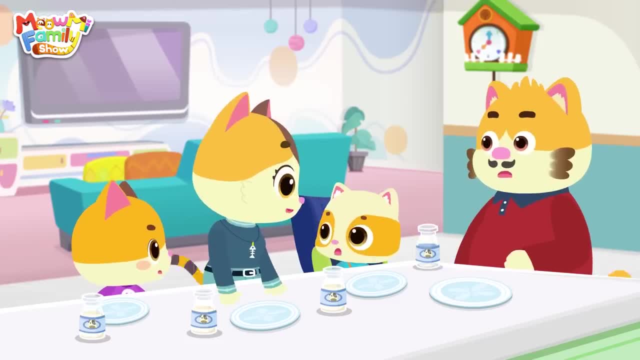 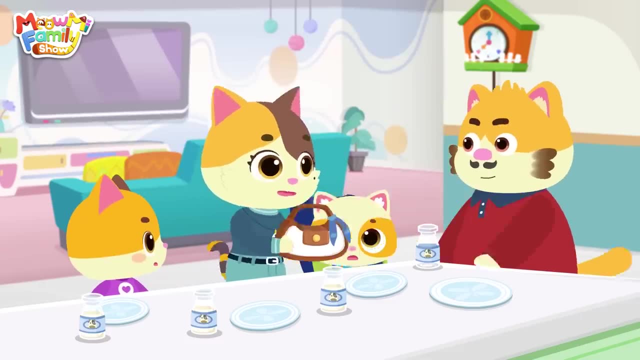 Oh, mommy needs to go now Watch me. Hey, Wow, I'm off to work. Bye, Uh bye, mommy. Daddy, when will mommy be back After she gets off work? What does mommy do at work? Do you want to know? 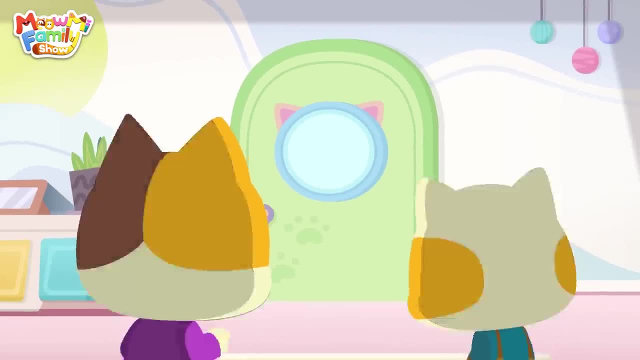 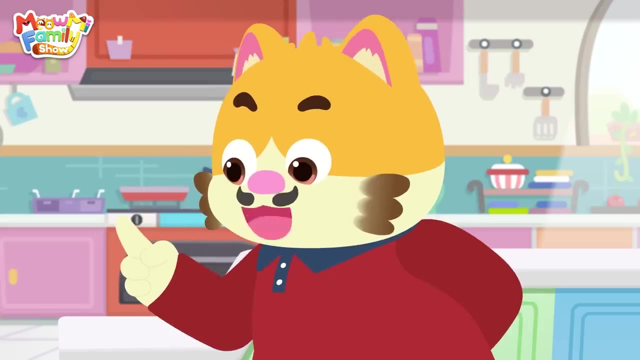 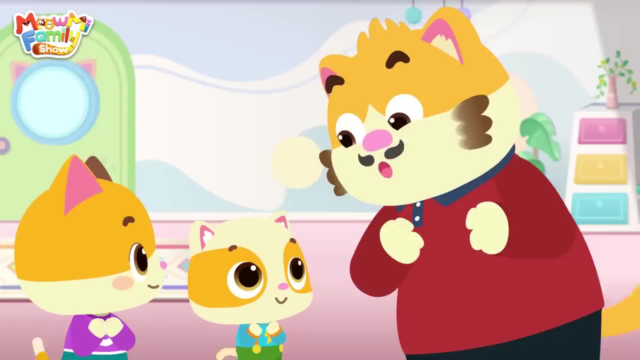 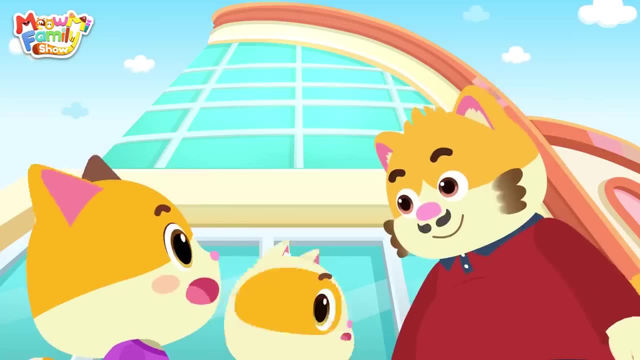 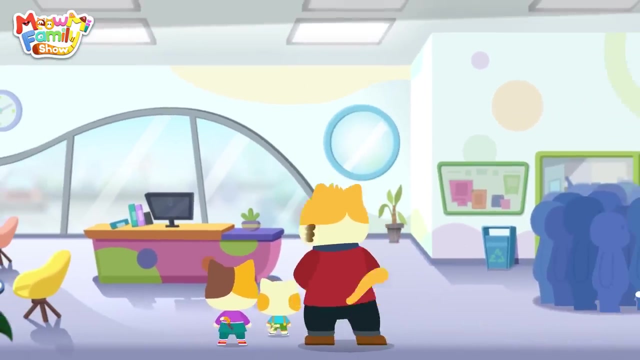 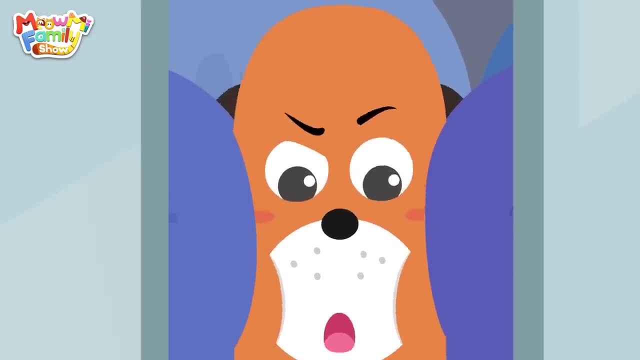 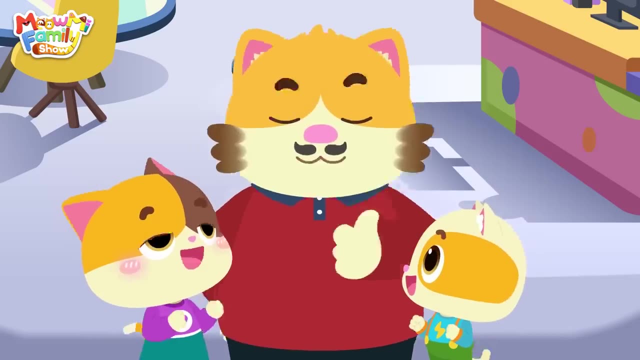 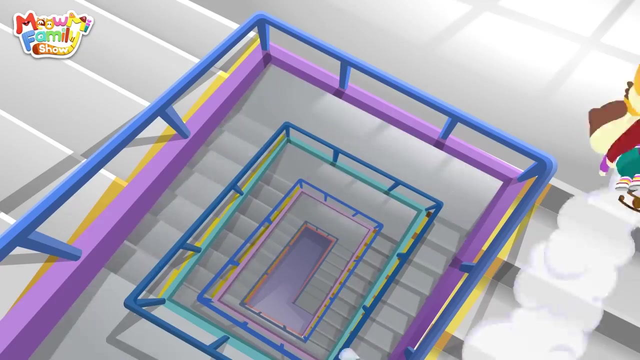 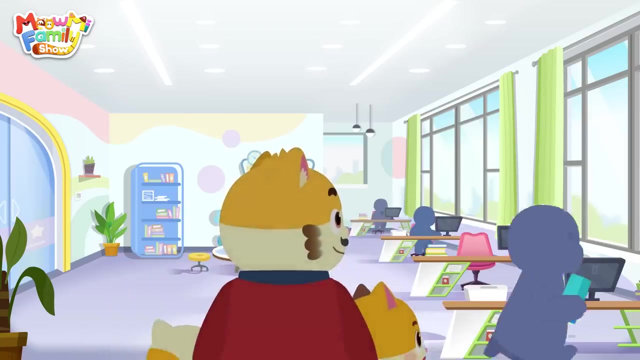 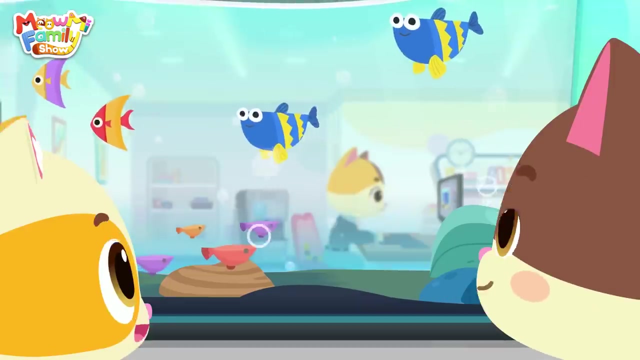 Ah-huh, It's good, it's good. Huh, So many people. It's okay, Let's check the stairs, The stairs, Ha-ha, Ha-ha, Wow, Wow, Mommy, Ha-ha. 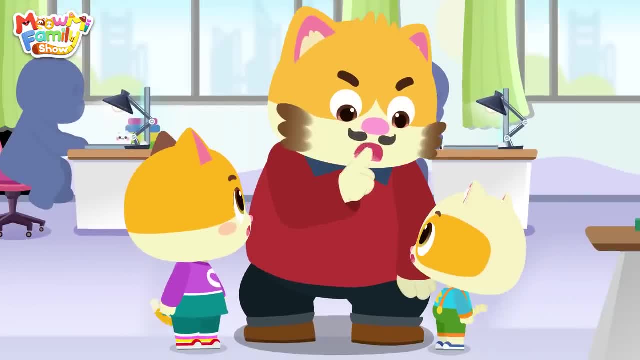 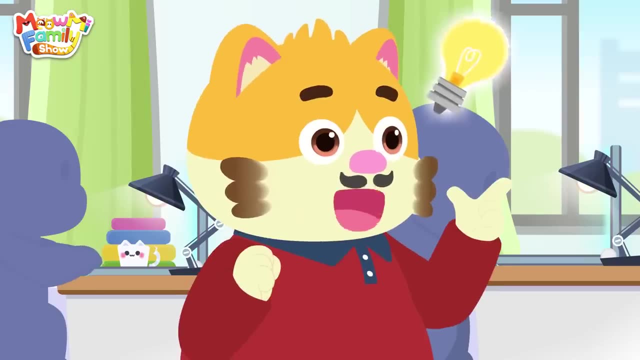 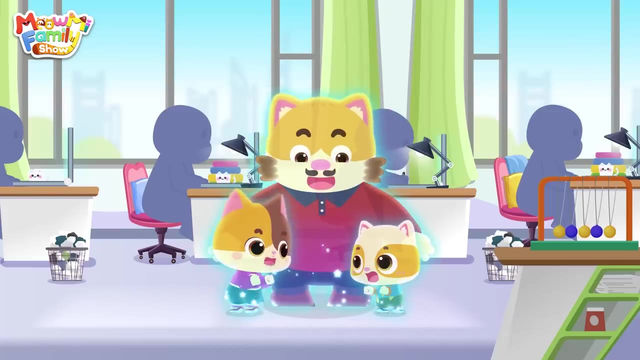 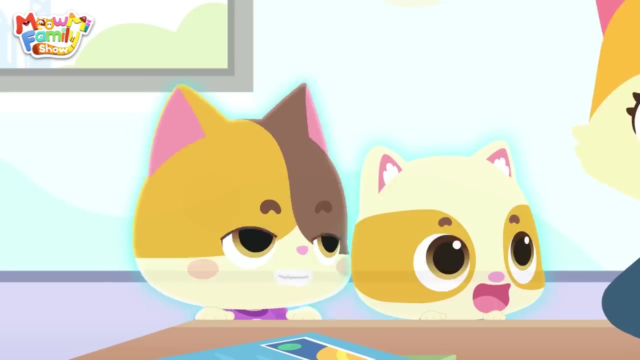 Shh, Mommy's working. Let's not disturb her, But I want to see what she's doing. Me too. I have an idea. Wow, We're invisible. Now we won't disturb Mommy as she works. She really can't see us. 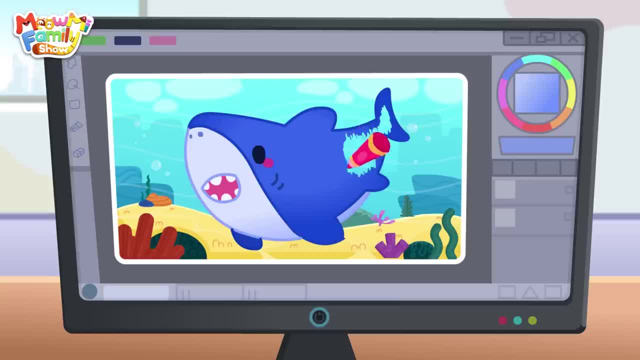 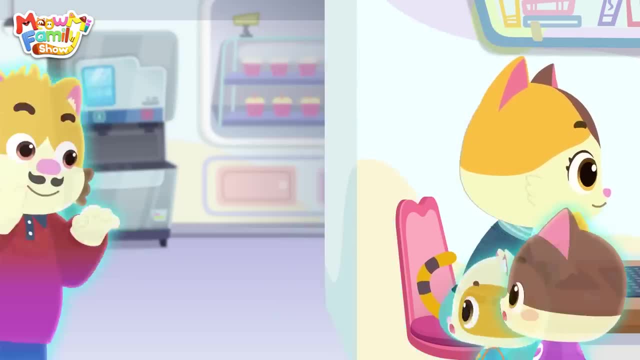 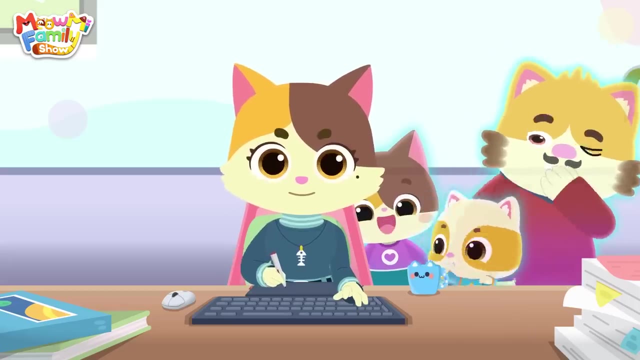 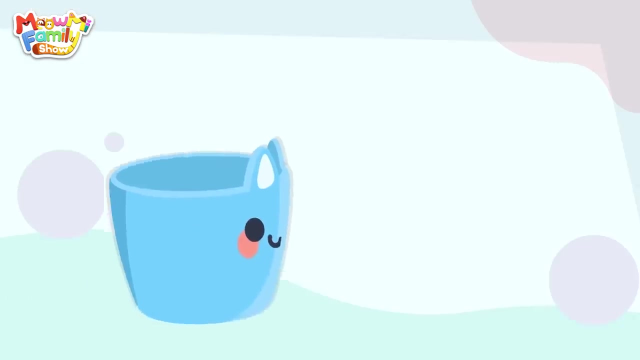 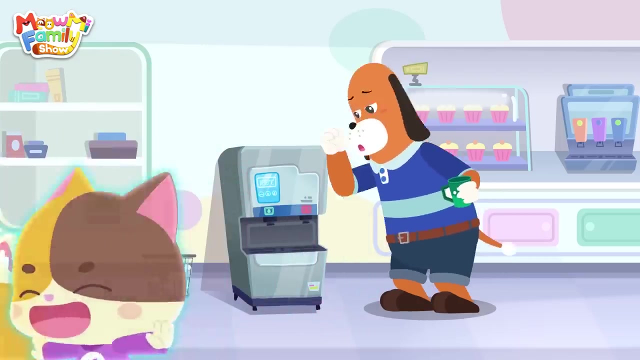 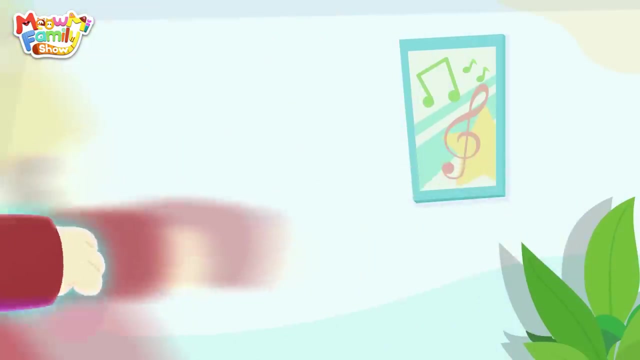 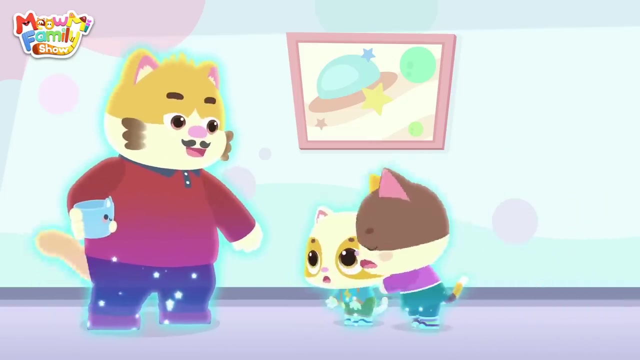 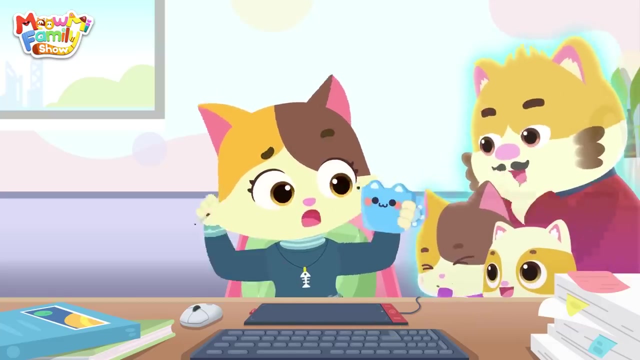 Wow, After I'm done with this, Hey kids, Let's go get some water for Mommy. Uh-huh What? Oh, I must be too tired. That's why, Hey Phew, That was great, Who brought me water? 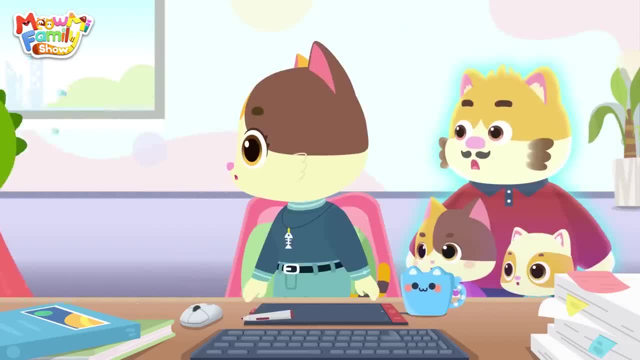 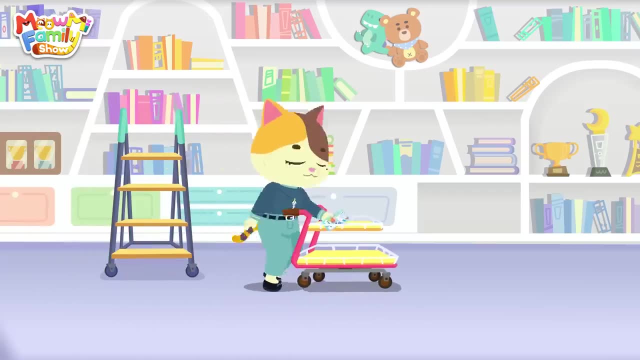 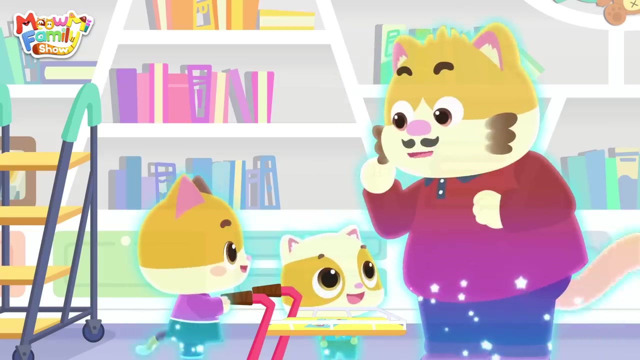 My goodness, Meetings and finding books. I'm so busy. I'll help you with the books. Oh, thank you so much. I think Sharkpedia is somewhere around here. Let us find the rest of the books. Okay, Whoa. 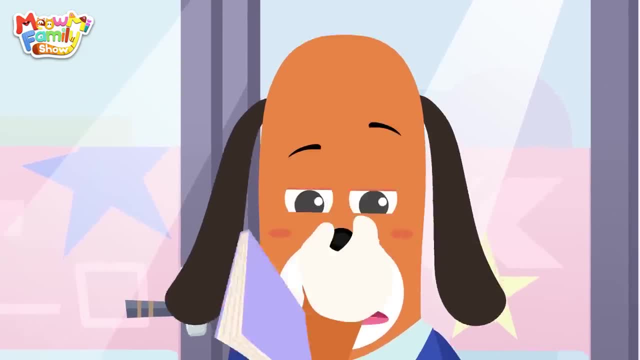 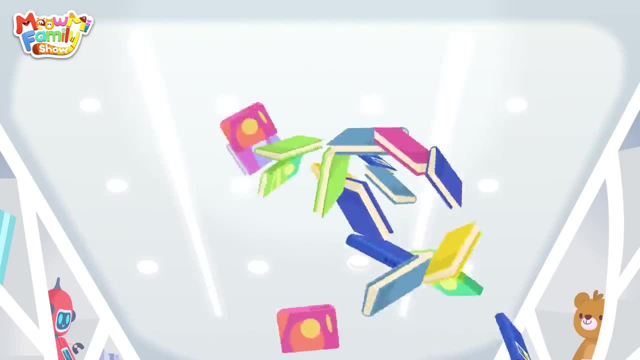 Whoa, Huh Huh, This is so scary. Huh Huh, Ah, Careful, Huh Huh, Wow. Who helped me find all the books? Good job, I need to copy these right now. 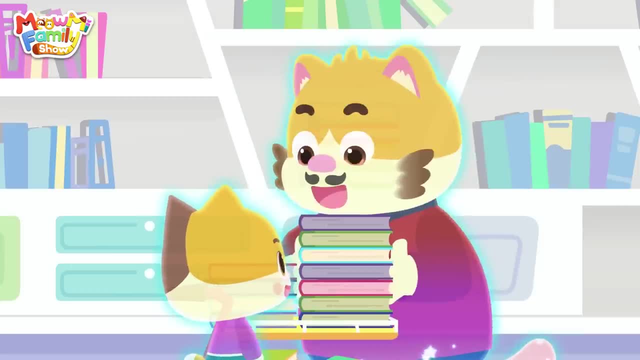 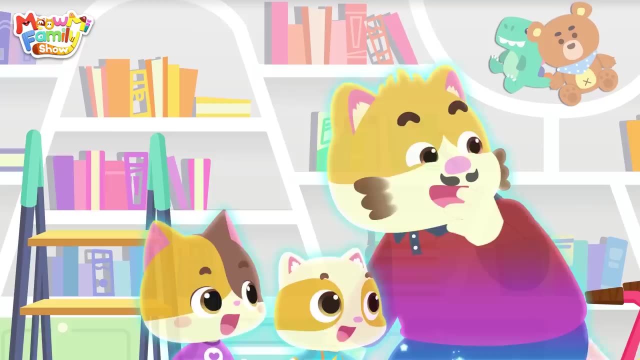 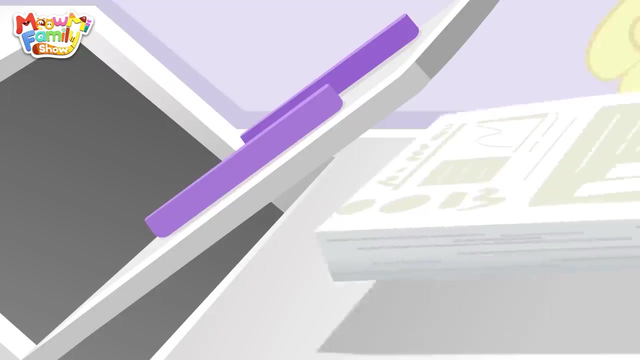 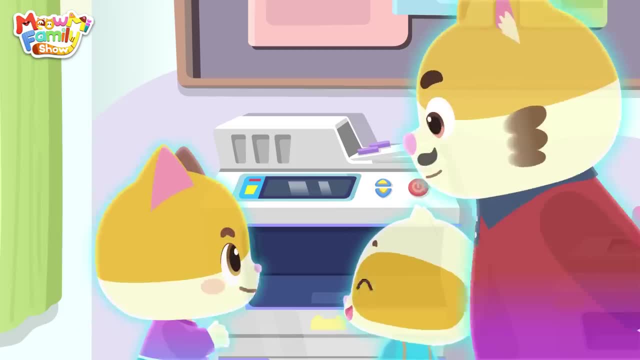 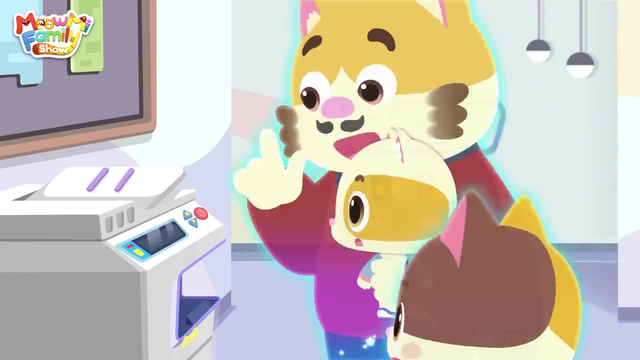 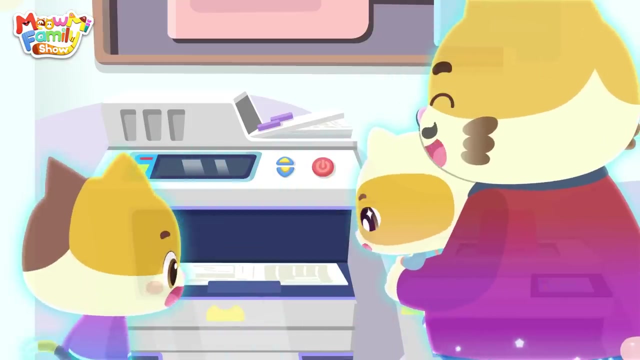 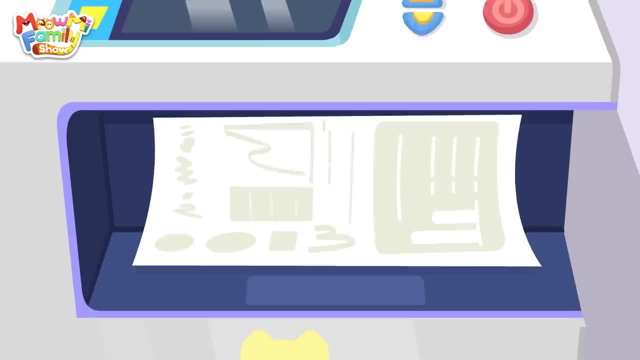 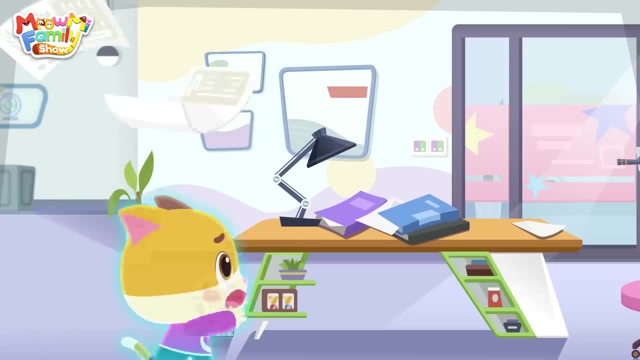 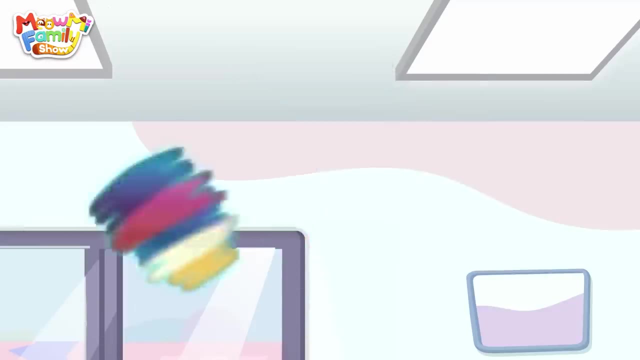 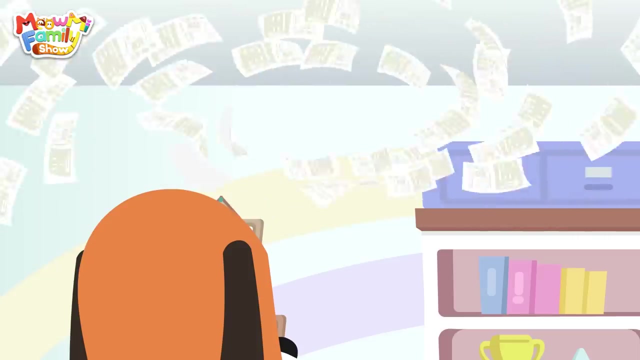 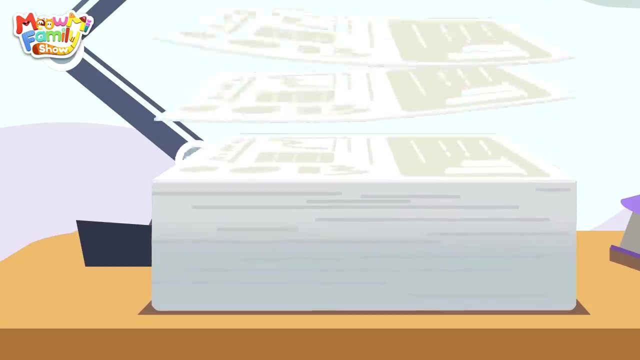 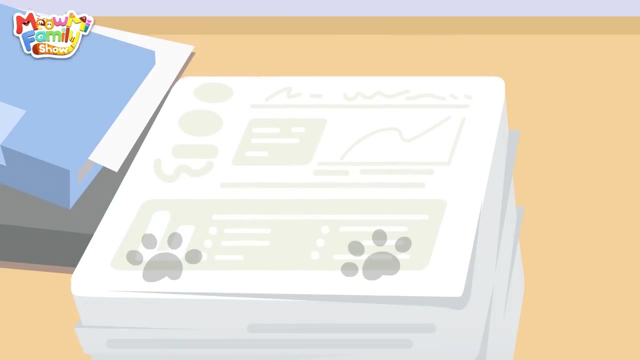 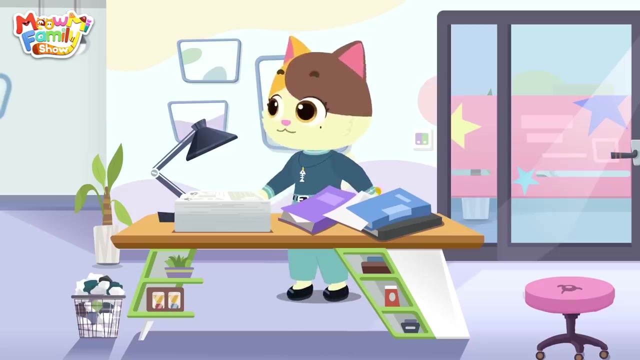 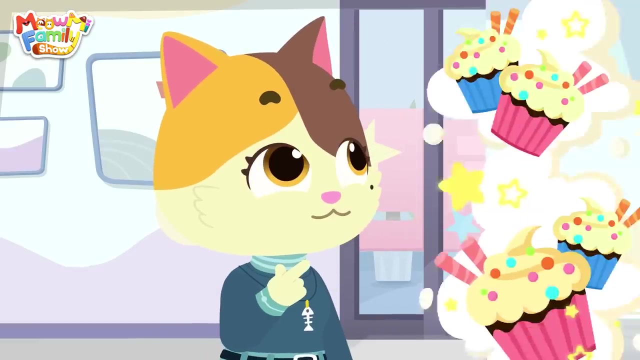 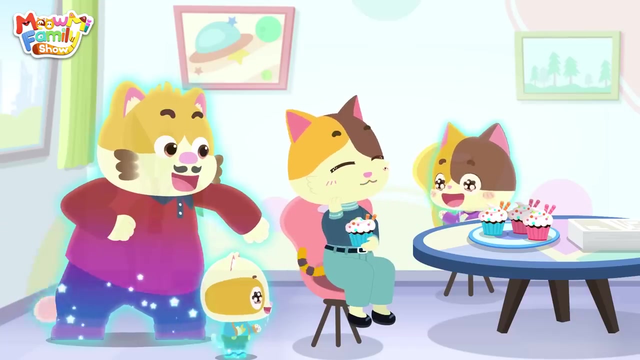 Hahaha, Yay, Yay, All done. They're everywhere. Please, no more strange things. Finally, The copies. Who's been helping me this whole time? Maybe some little angels came to help me. This is so yummy. 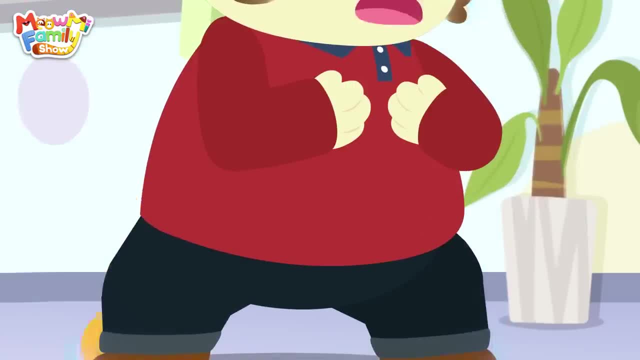 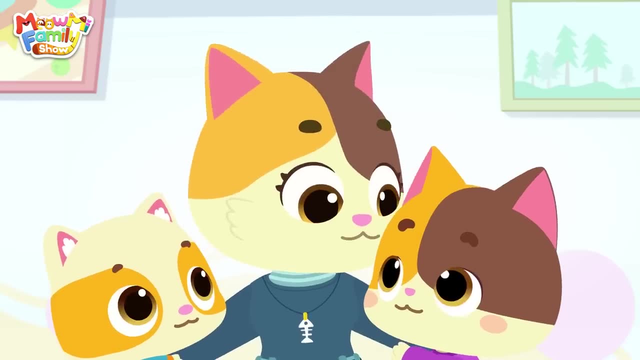 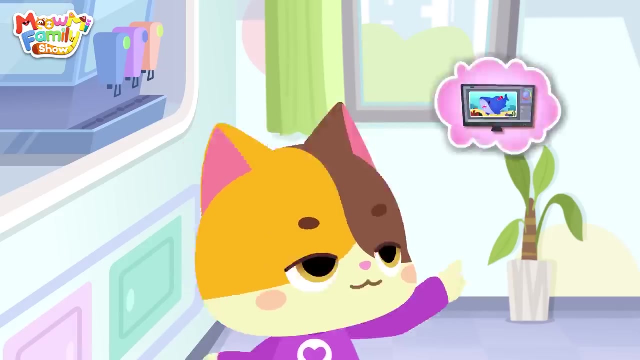 Oh no, I'm hungry. I'm losing my superpower. Sure enough, it was you, Mommy. How come you're here? We wanted to see you working. So what do you think Working is so much fun? We can draw, read and use the copier. 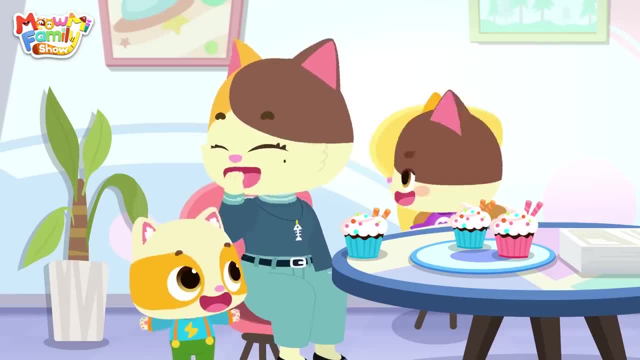 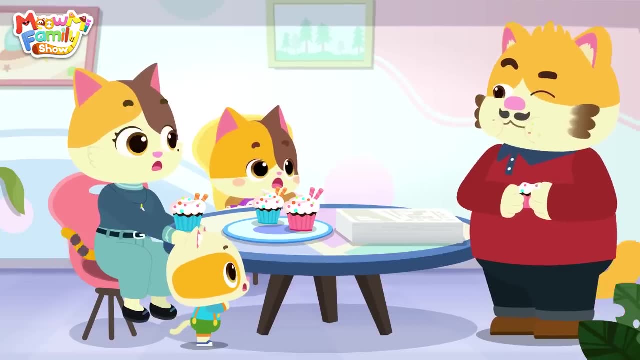 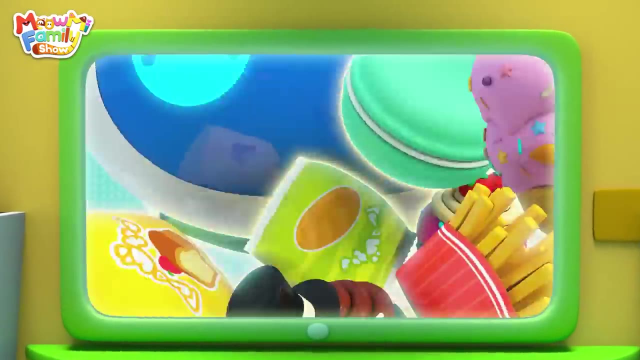 And we can eat yummy snacks. I love this place. Thank you for helping me today. Why don't we have some cupcakes now? Yay, I was really hungry. so What's your favorite snack? Just name it, The Robot Snack Maker will make it for you. 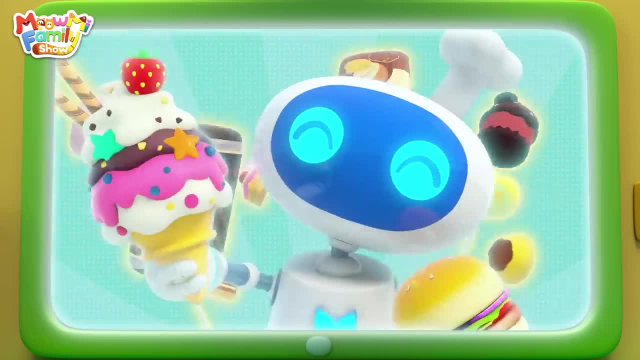 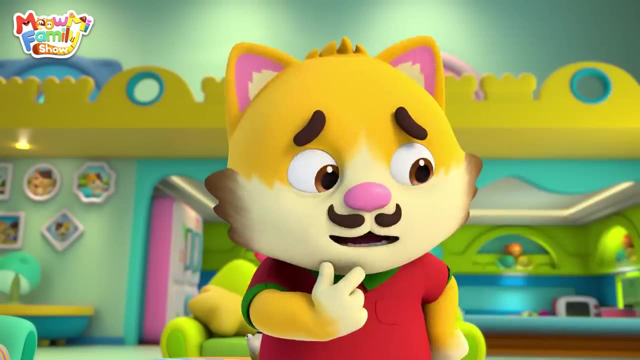 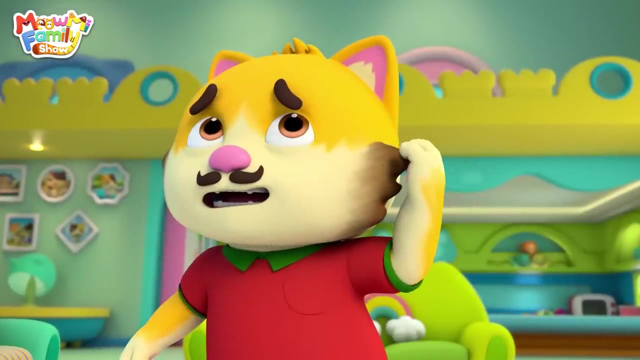 Whoa, Order your Robot Snack Maker now. Whoa, Come on, Daddy, Let's buy one. Well, too many snacks will make our tummies hurt, Daddy, please. Uh, um, All right, Yay, That's great. 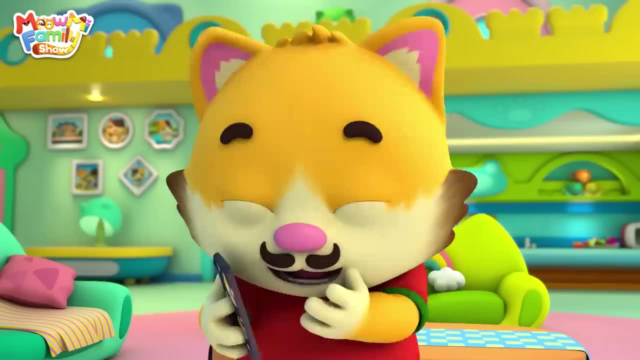 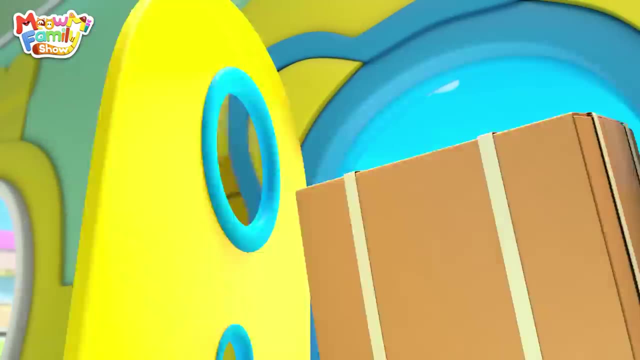 But you have to promise you can't have too many snacks. Uh-huh, Hi. I'd like to order a Robot Snack Maker, Sure, right away. Here's your package. Please sign here. It's here already, Mm-hmm. 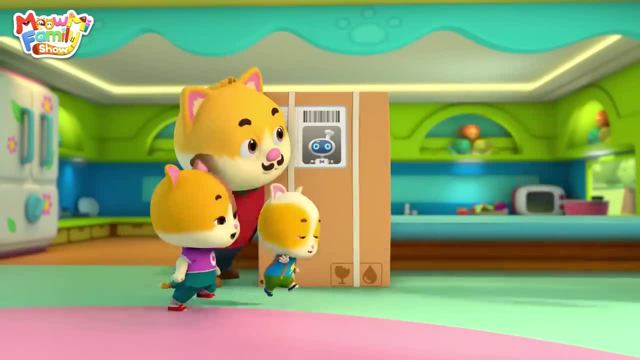 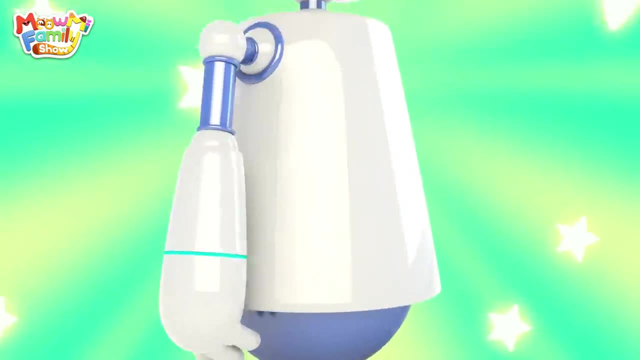 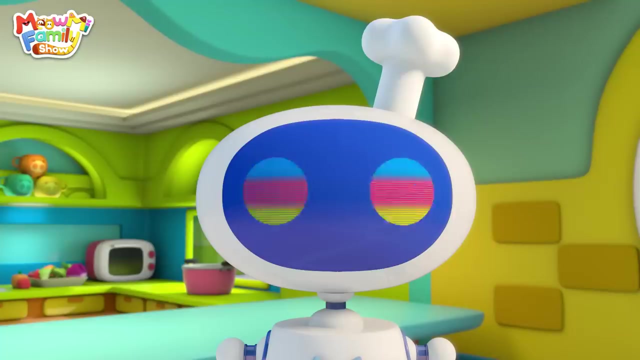 Wow, Thanks, Ha-ha, No problem, Bye-bye, Bye, Come on, Let's open it. Uh, Hee-hee. Oh, Wow, It's so cool. Power on Whoa Yay. Hello, I'm Robot Snack Maker. What would you like? 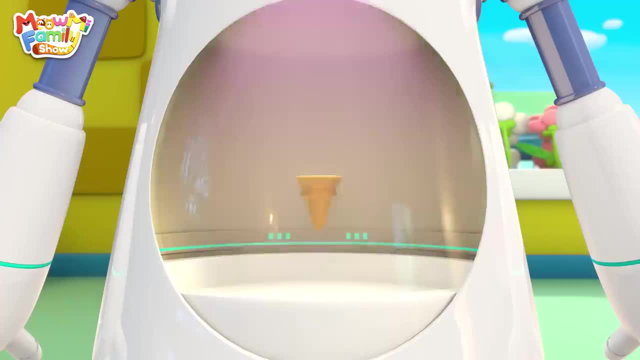 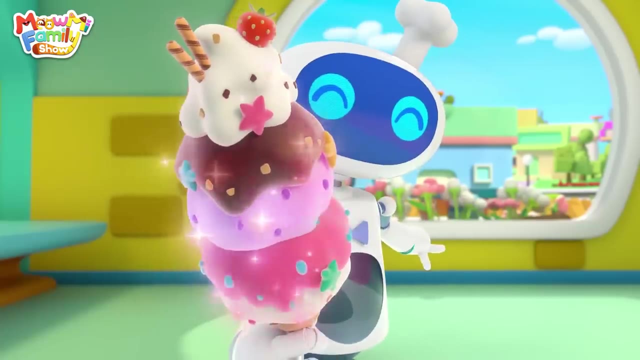 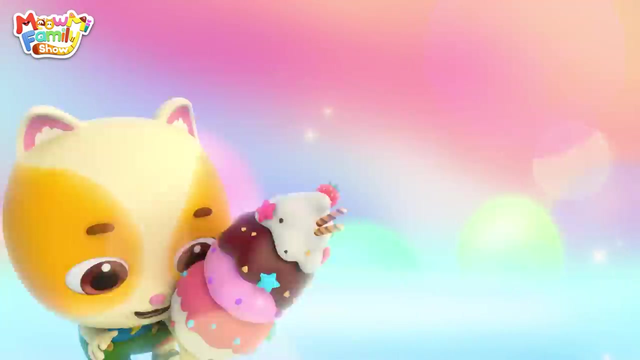 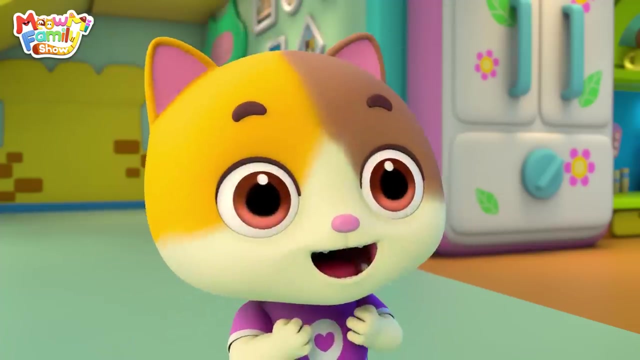 Ice cream, please. Okay, Working on ice cream? Whoa, Here's your ice cream. Whoa, It's so big. Ha-ha, Ha-ha, It's so yummy, Hee-hee, Whoa, Robot Snack Maker, I want cotton candy. 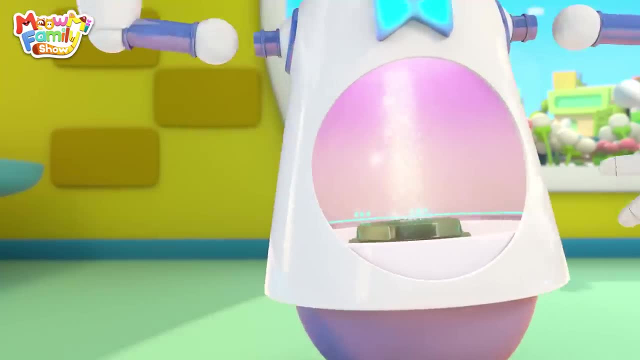 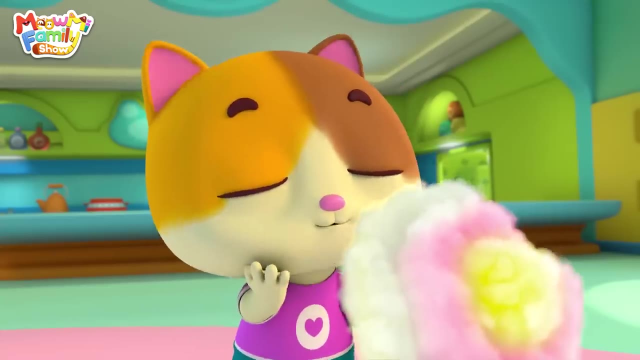 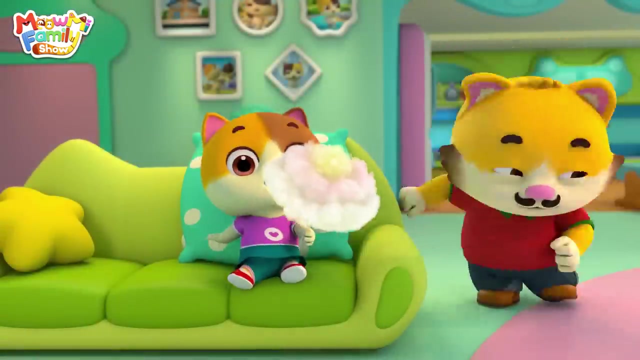 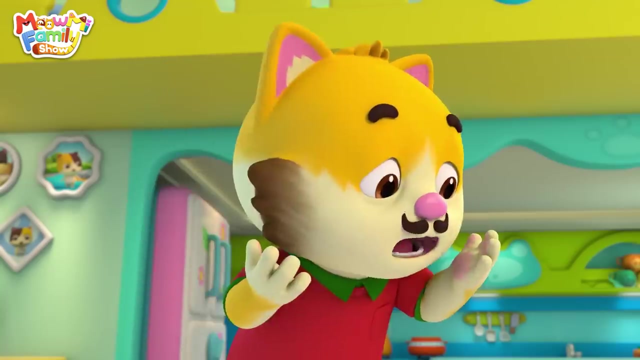 Okay, Wow, Here's your cotton candy. Oh, It's so yummy, My turn, My turn. Ice cream, please. Uh, no, Cotton candy, please, Ice cream, Cotton candy, Ice cream. Okay, Working on cotton candy ice cream. 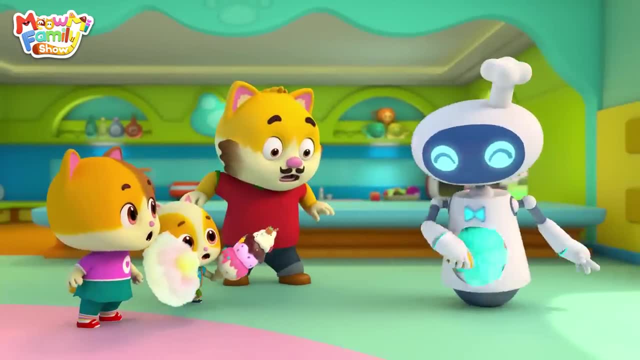 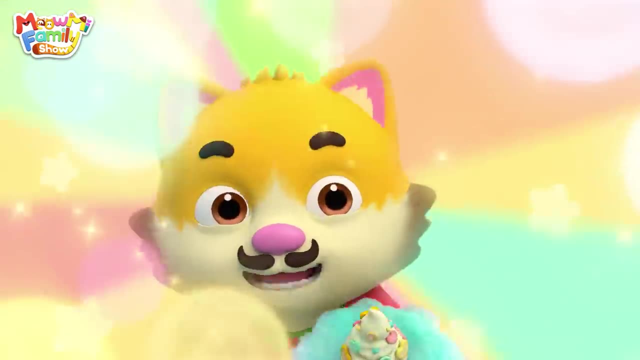 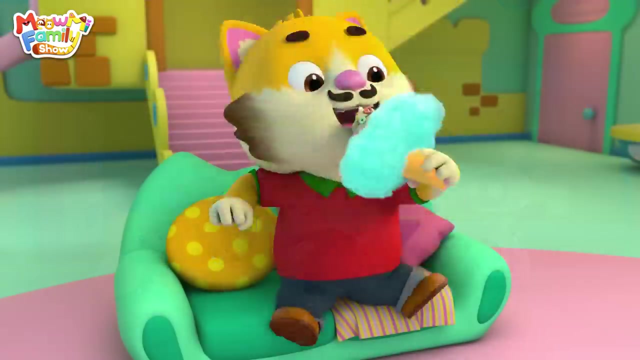 Uh, No, no, no, no, Uh, Uh. Huh, It looks yummy, though. Wow, This is the best ice cream that I've ever had. Yoo-hoo, This is awesome. I'll have another one. 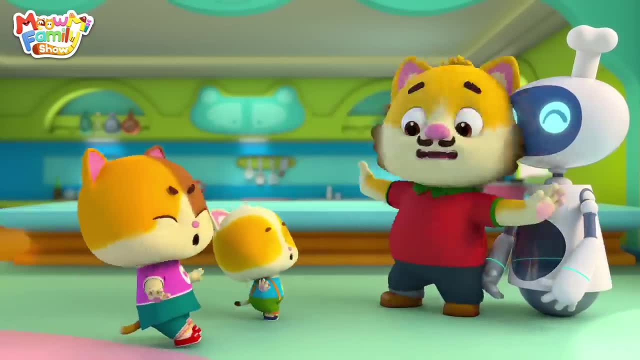 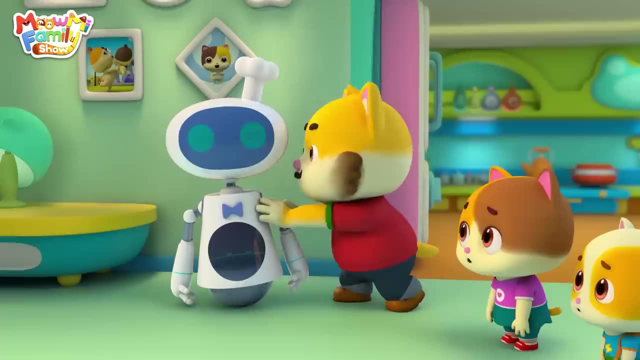 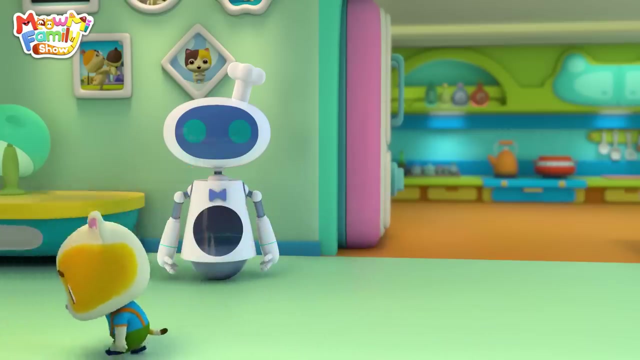 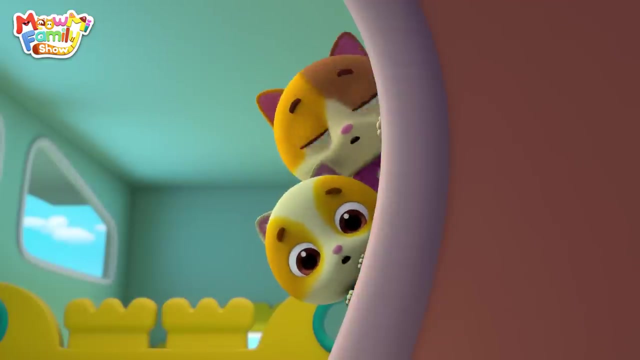 Me too. Uh Uh Uh, No more snacks, kids, Or your tummies will hurt. Uh-huh Huh, Until tomorrow. Okay, See you tomorrow. robot Psh, Psh Hush. 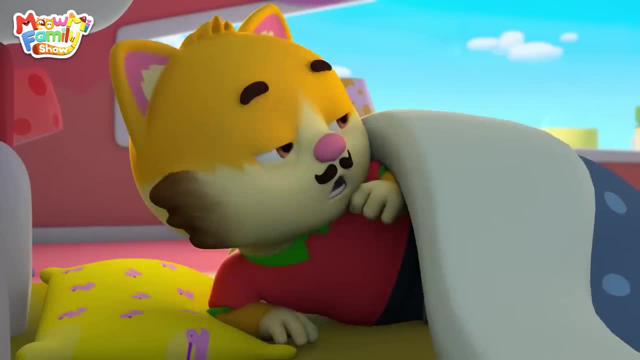 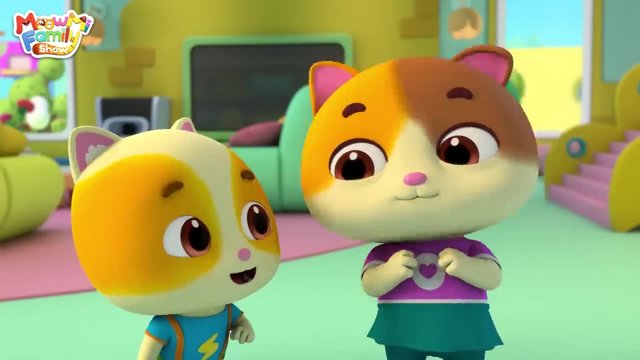 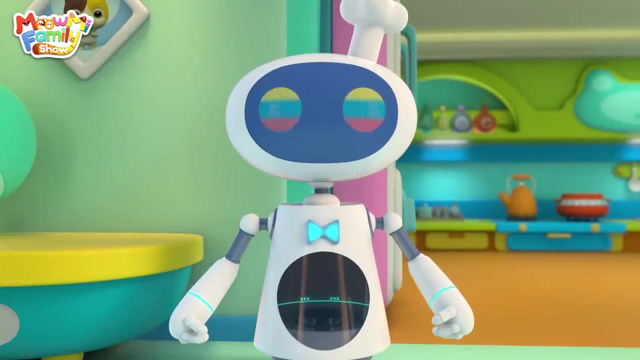 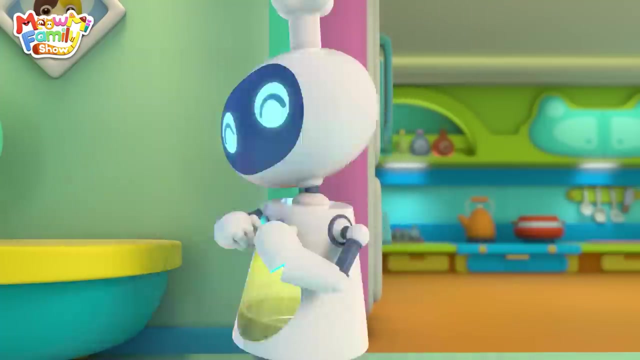 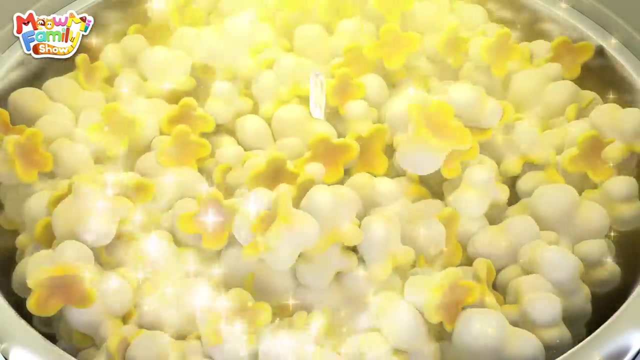 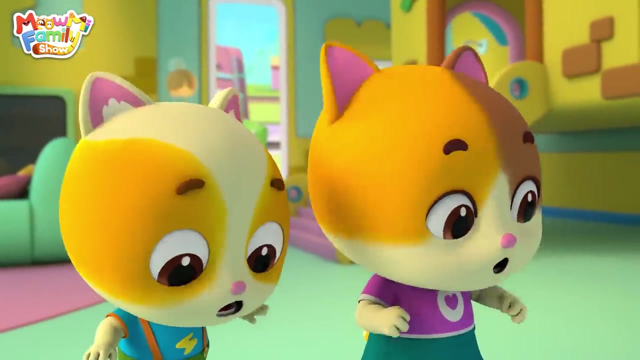 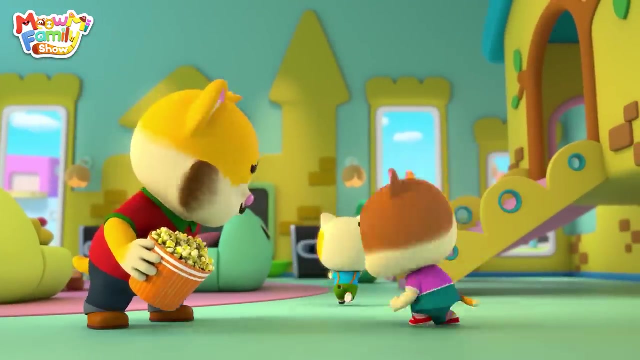 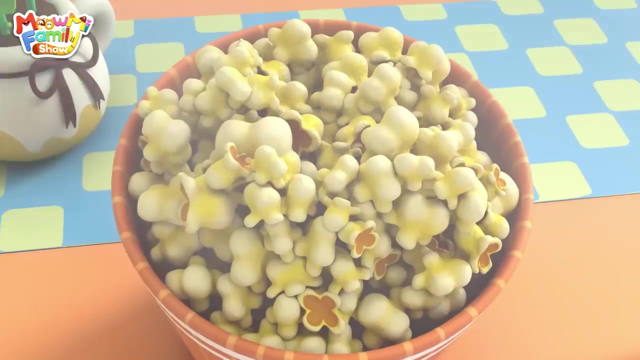 We did it. we got past. daddy, I'm gonna eat everything I want. Yay, Hello, what would you like? I want popcorn. Okay, working on popcorn. Daddy, You sneaky little eaters trying to have more snacks Run Such naughty kids. Oh wow, it smells so good. 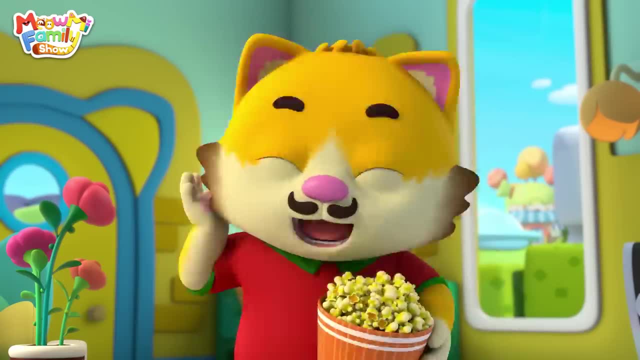 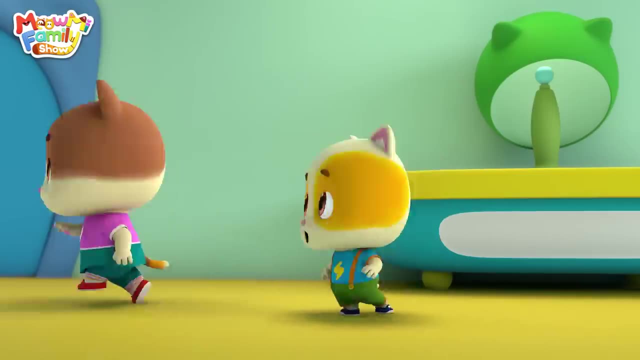 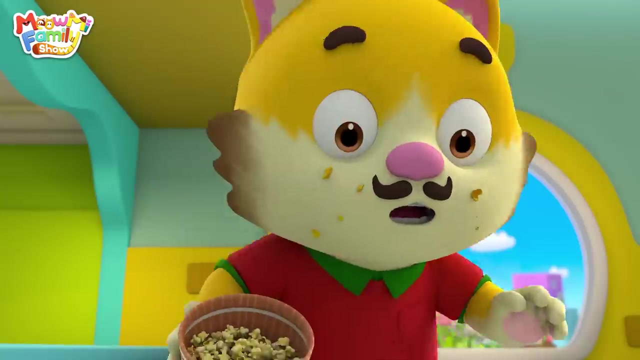 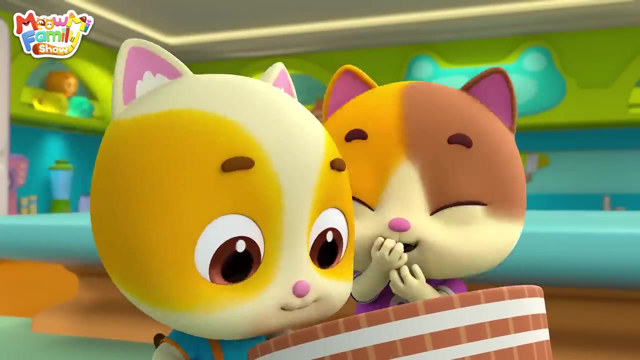 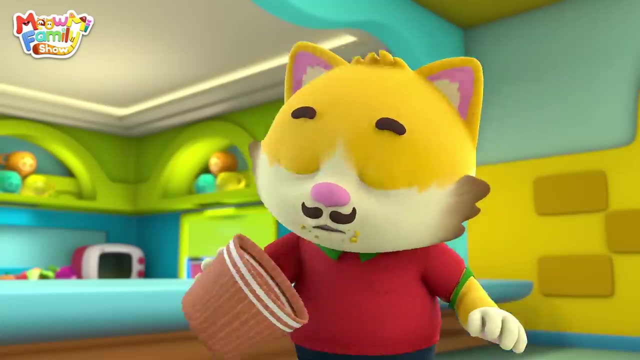 Wow, it's so yummy, Daddy. what are you doing? We've got you, daddy. It looks so yummy, so We want some too. I'm gonna try other snacks, Me too. Me too, Oh wait, Robot snack maker. I want chocolate and pudding. 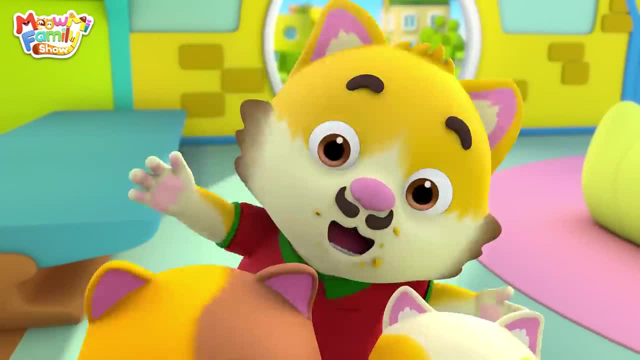 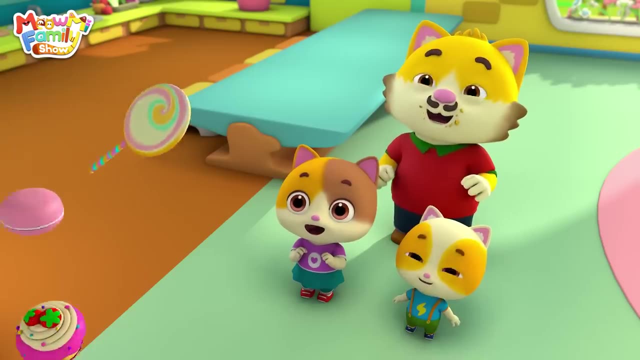 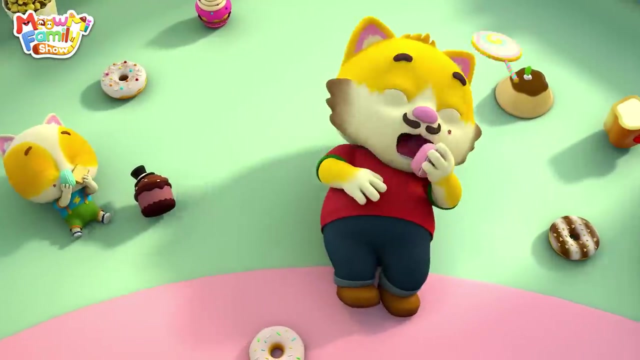 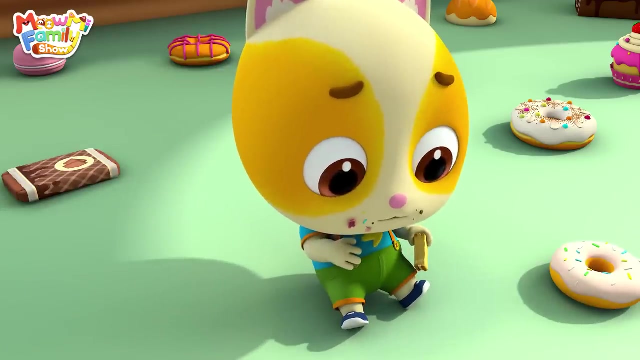 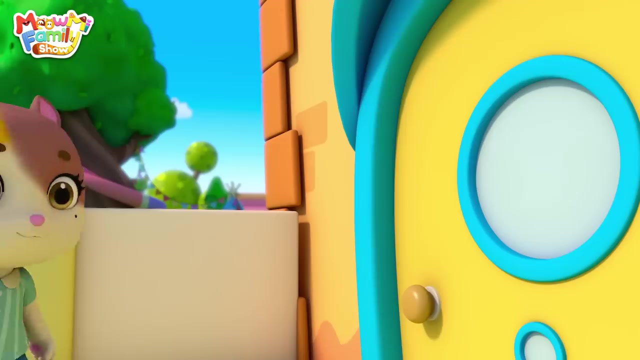 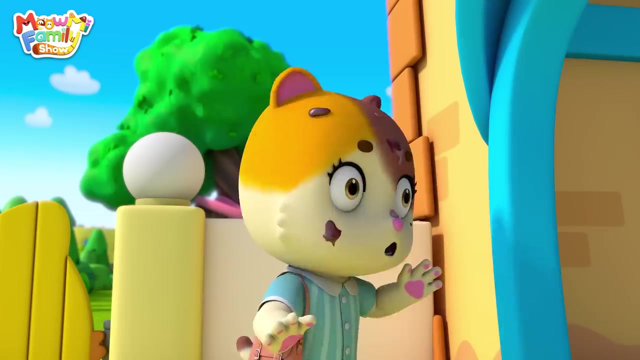 I want lollipops, donuts and cookies. I want vanilla macarons. Okay, working on them. Why is my tummy grumbling? Oh well, not a big deal, I'm back. What's going on? Cupcakes, pudding, macarons, donuts. 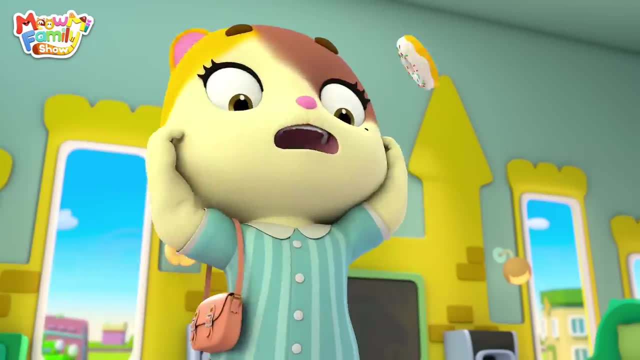 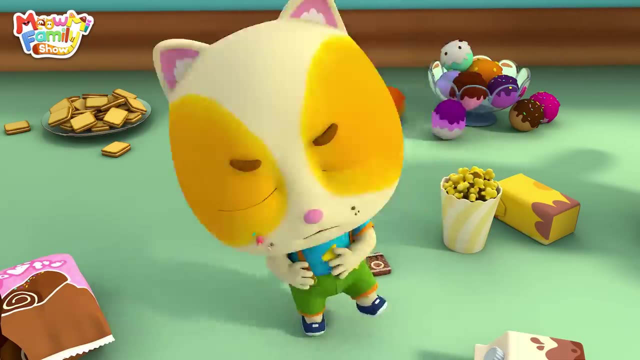 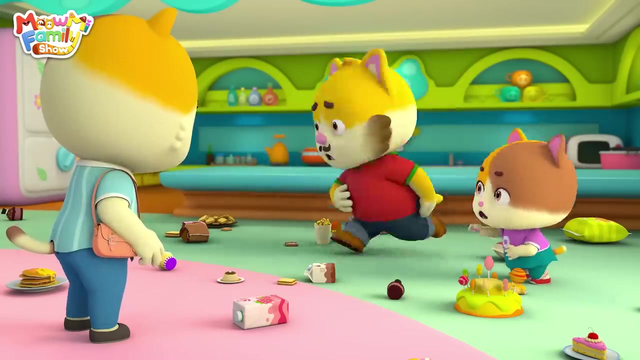 Oh no, Did you eat all of these snacks, Are you alright? Sure Ow, my tummy hurts. Huh, My tummy hurts. Mine hurts too. Oh no, mine too. Ow ow. I need to go to the bathroom. I'll go first. 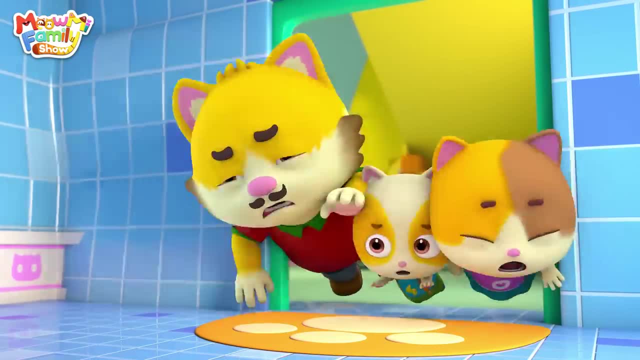 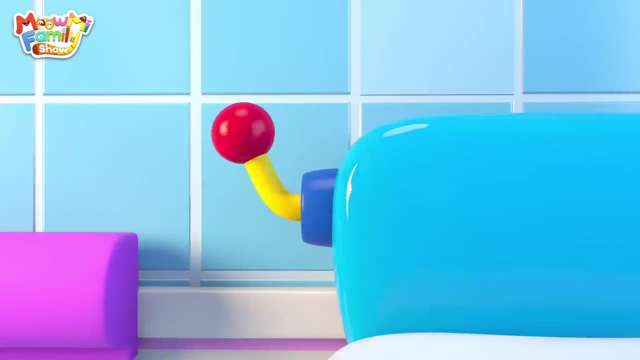 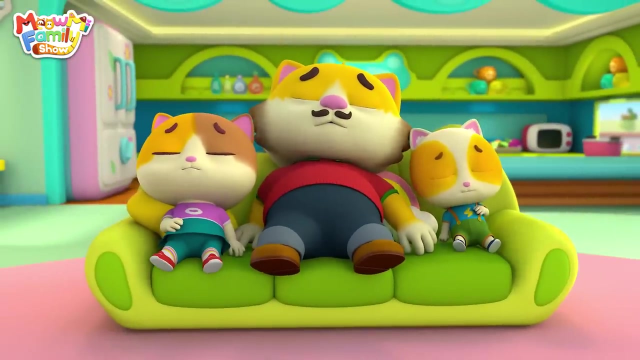 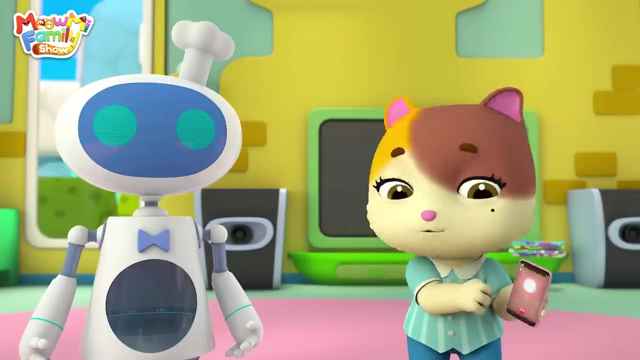 Oh, ouch, I can't hold it. I'll go first. Ouch, I'll never eat this many snacks. Huh, I can't hold it. I can't hold it. Ugh, I'm hungry. Then let's send the robot back. Got it? Feel free to order again. 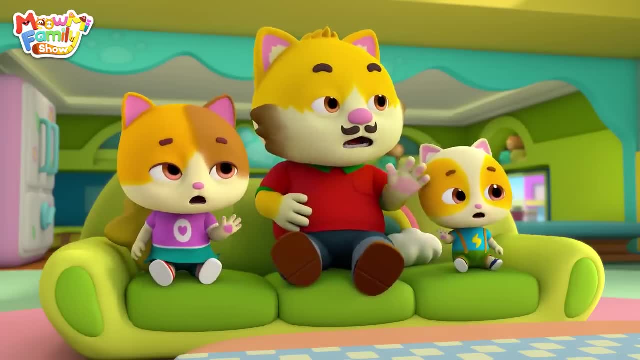 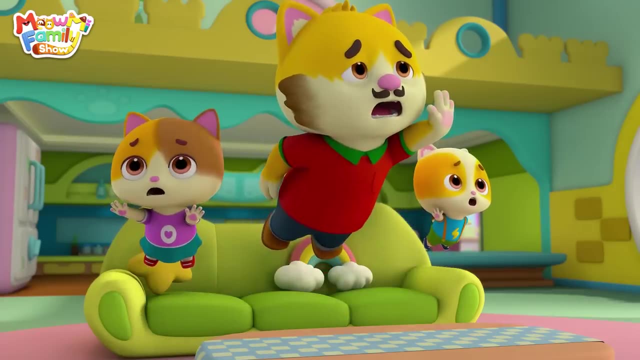 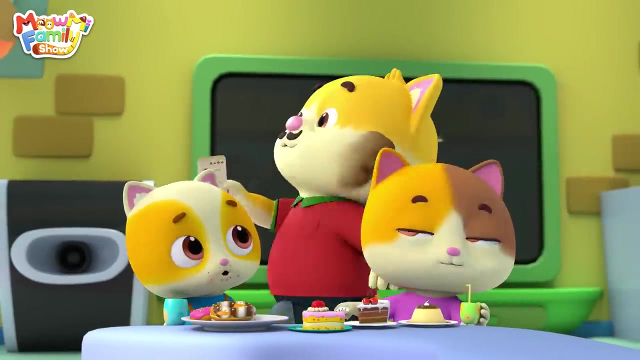 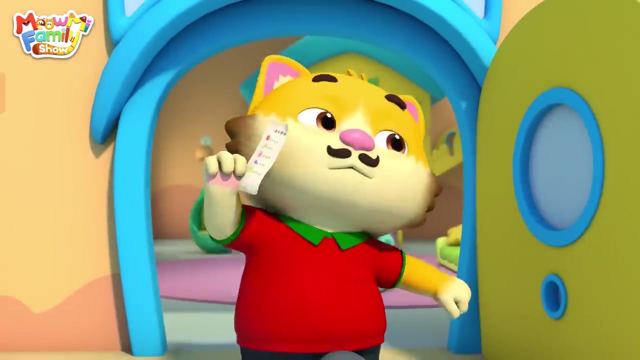 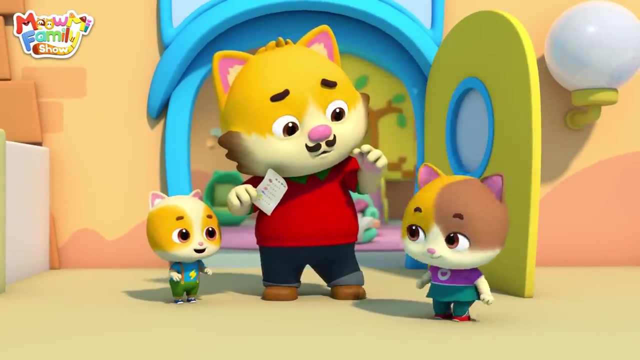 Bye, Bye, Bye-bye. Ugh, I need to go again. Ugh, I need to go again. Time to go shopping Tonight. I'm going to the supermarket. I'm going to buy a nice-looking car. Daddy, we'll go shopping for you. We're all grown up now. 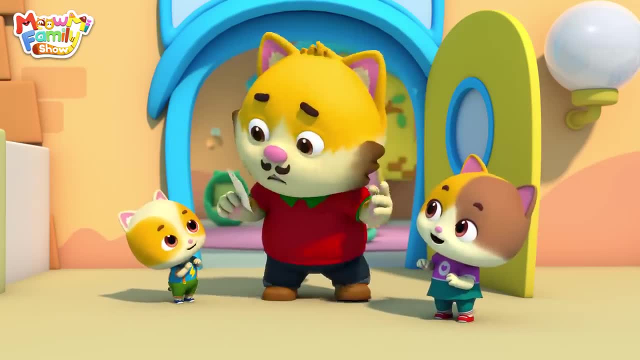 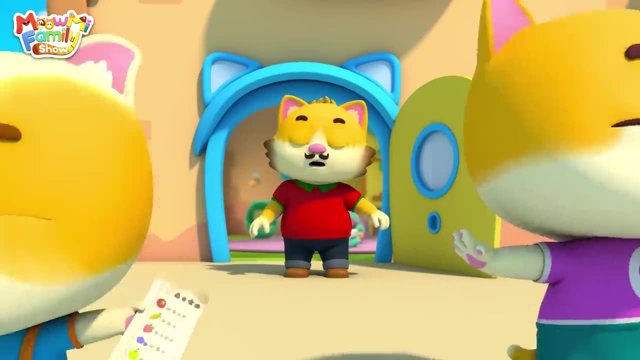 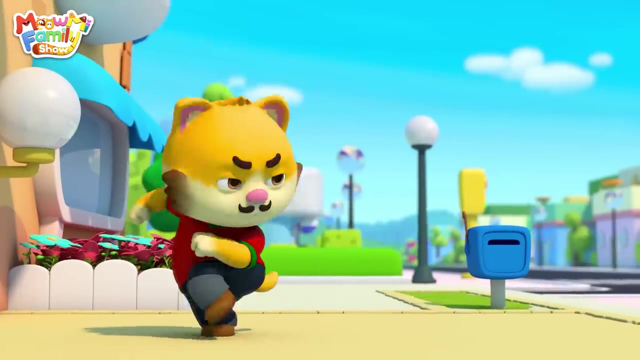 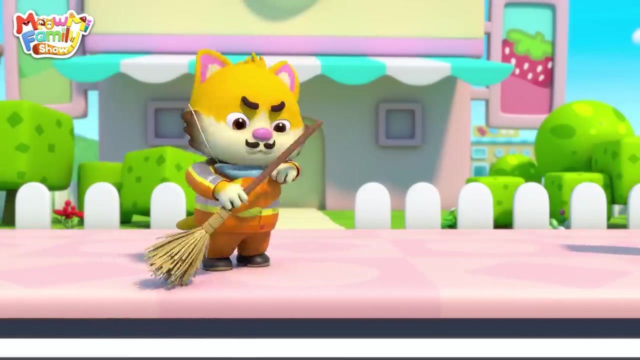 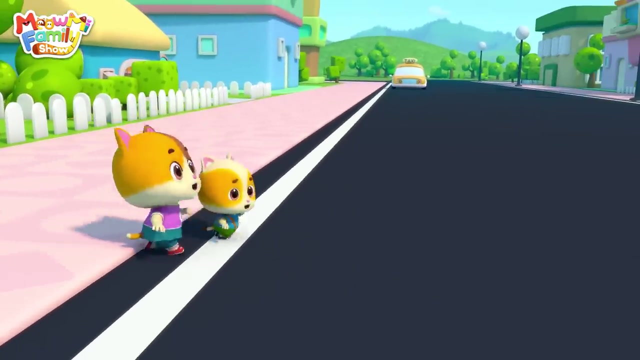 We can run errands for you, But it's dangerous outside. We'll be careful, Don't worry. you don't have to follow us. Can they protect themselves? I don't think, so I need to follow them. Let's cross the street. Okay, Watch out. 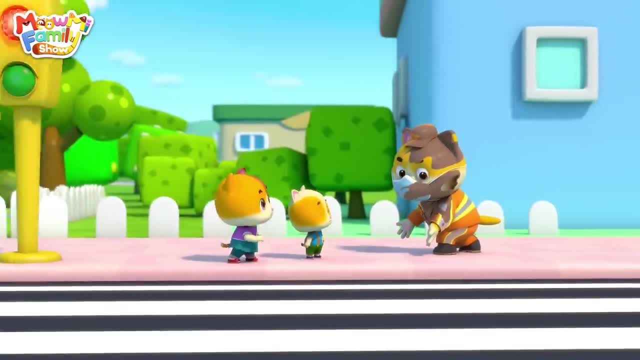 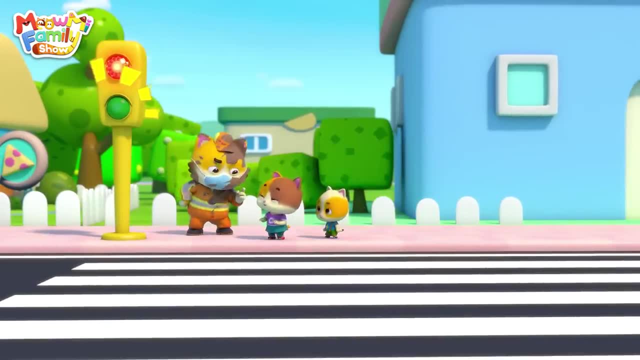 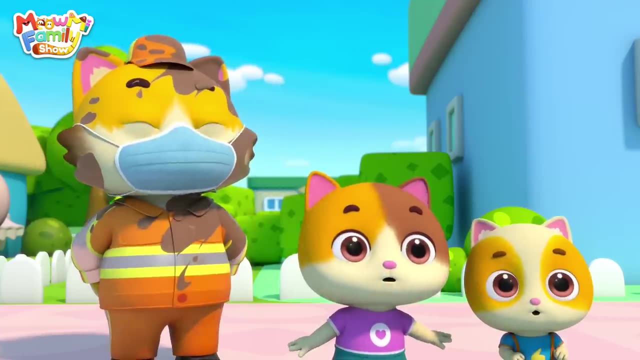 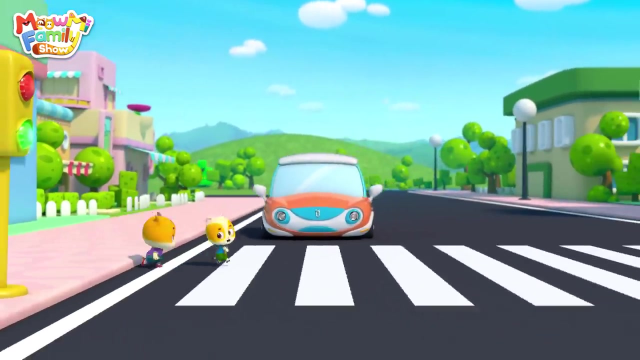 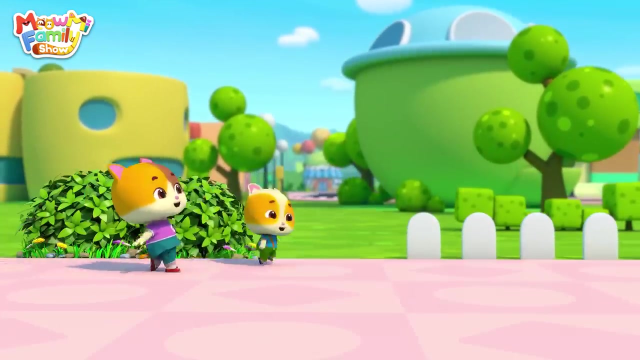 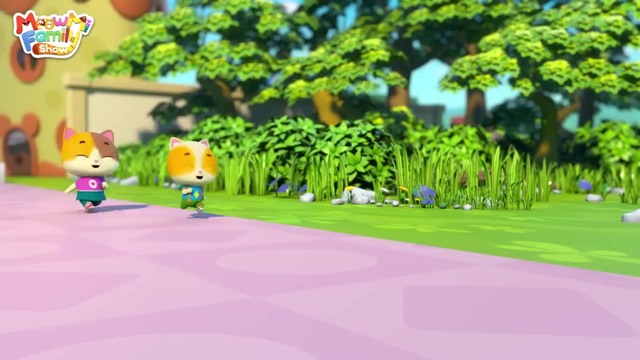 Kids. that was so close. Always use crosswalks when you cross the street. Also, stop at the red light And go at the green light, okay, Okay, Mr Street Cleaner, It's green, Let's go, Hi, Mimi. 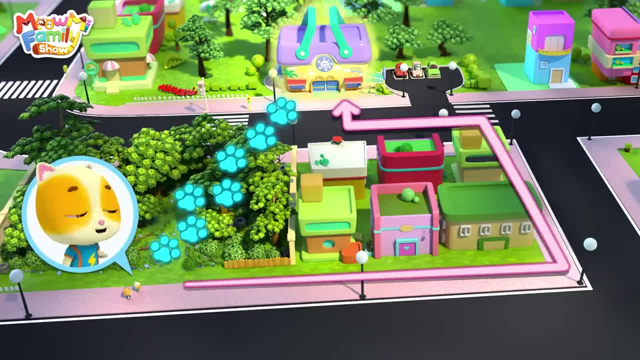 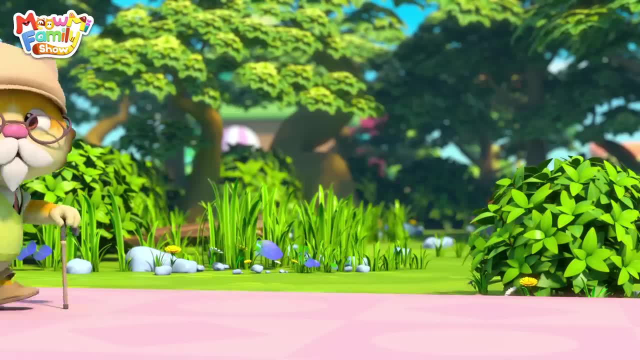 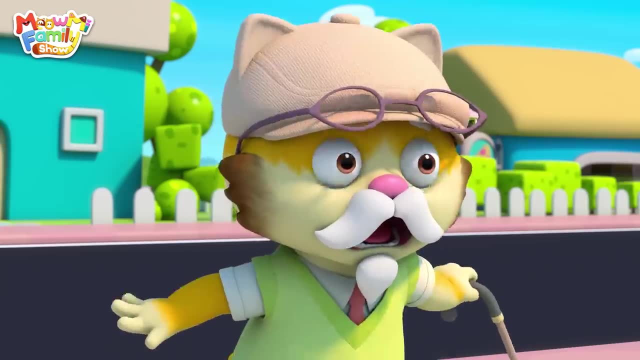 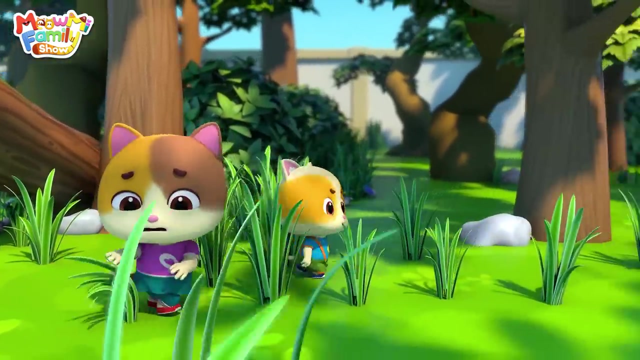 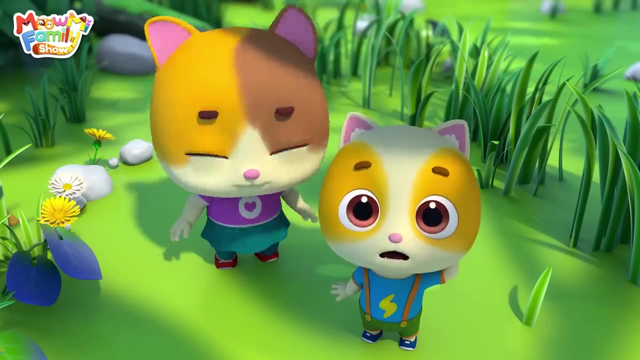 I think this is a short cut. Let's go this way. Timmy, you're so smart, Let's go. Oh no, You shouldn't go that way, Kid. you shouldn't take narrow roads. You might come across something dangerous, Like what. 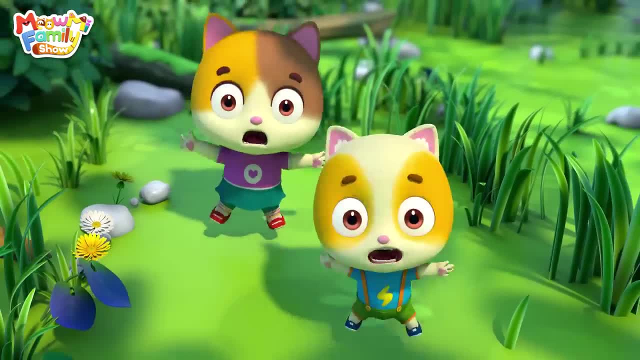 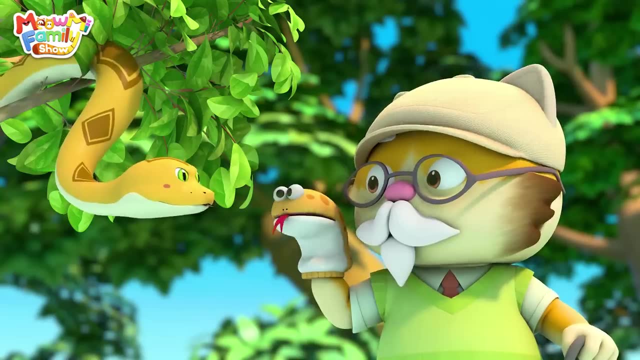 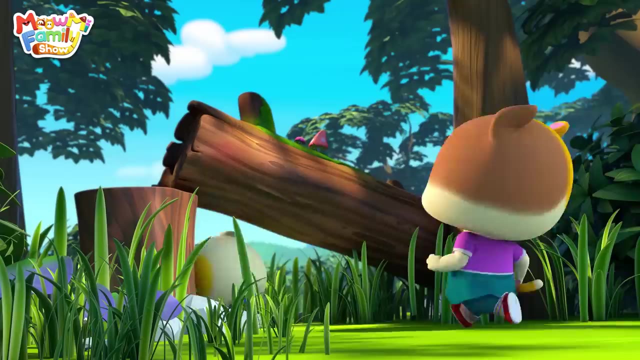 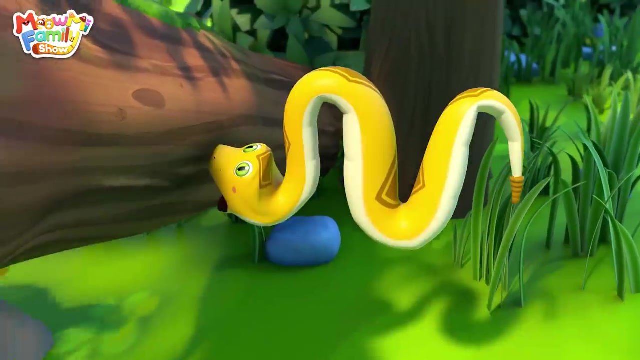 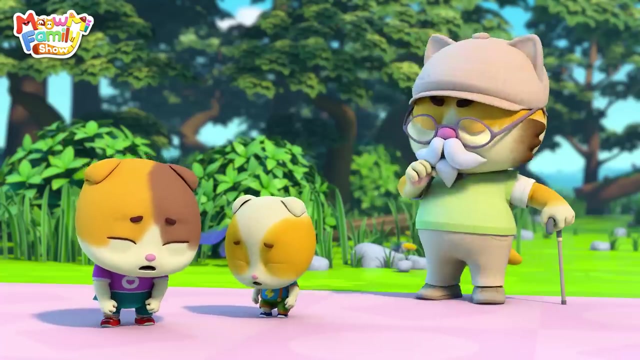 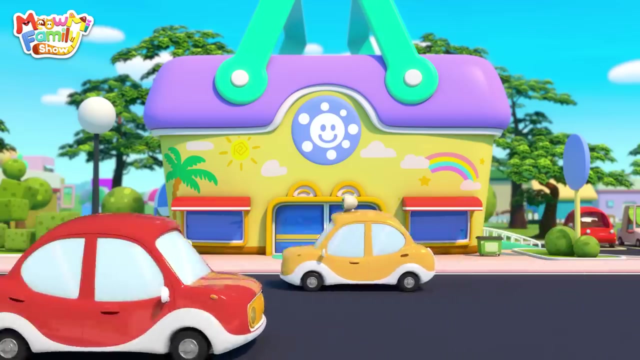 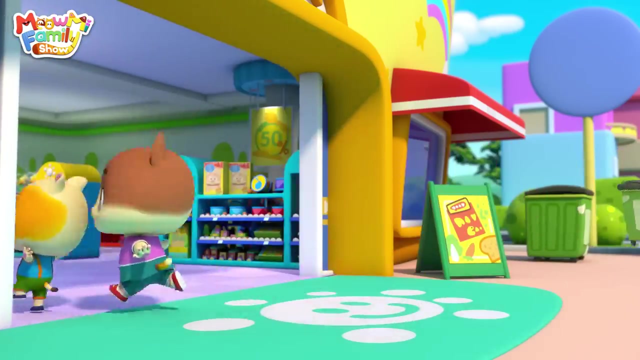 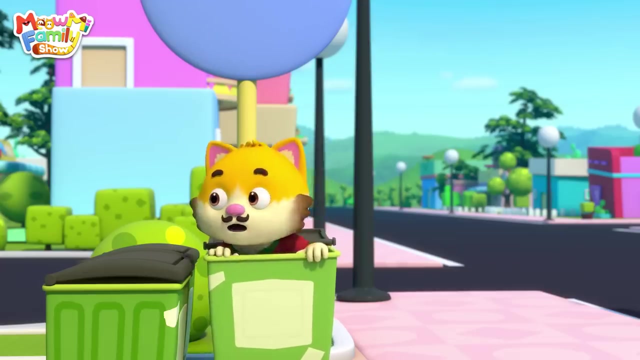 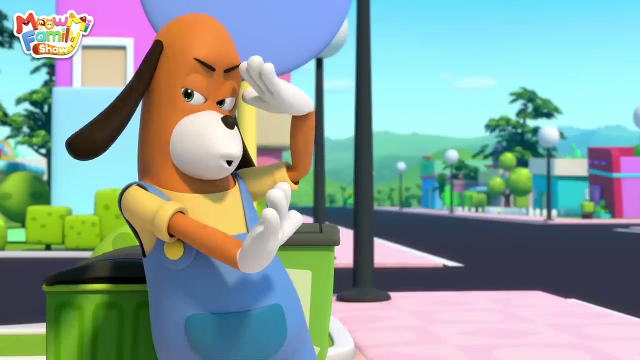 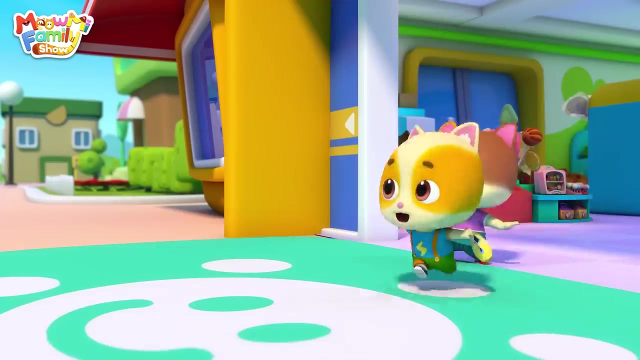 Like a snake, Oh snake, This is just a toy. Run, Run, That was close. kids Never take narrow roads again. Okay, sir, Yay, We're here, We're here, Yay, We're here, Oh no. 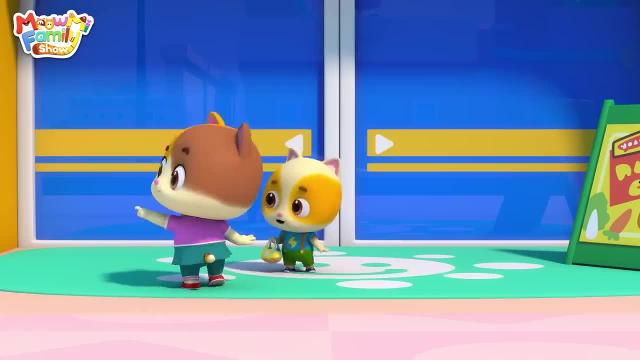 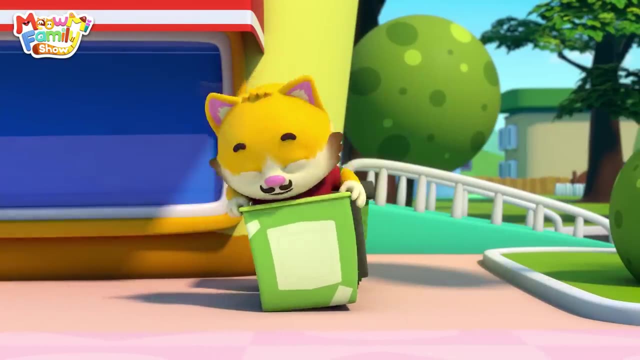 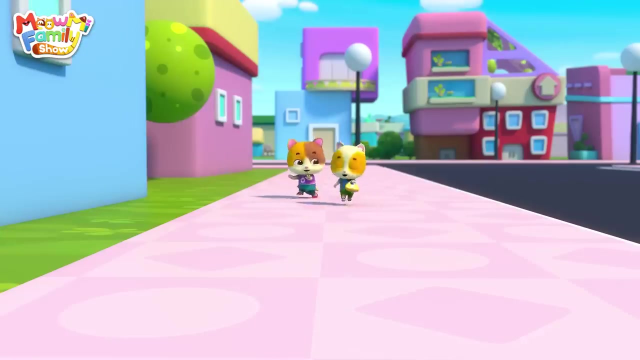 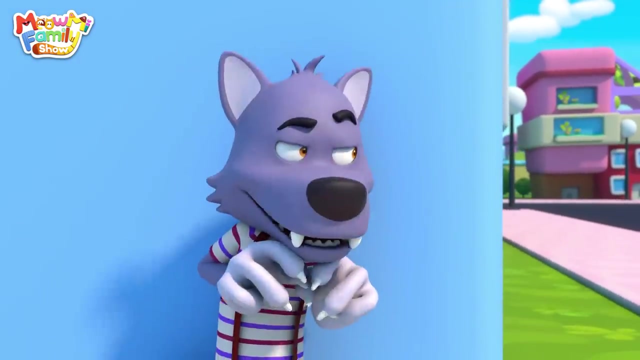 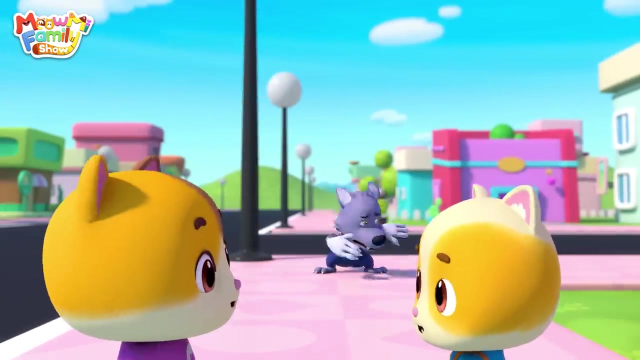 That's so scary. Oh no, We're here. We're here, We're all done. Now let's go home. Yay, Ha-ha, They did it so quickly. Good job, Sir. what's going on? 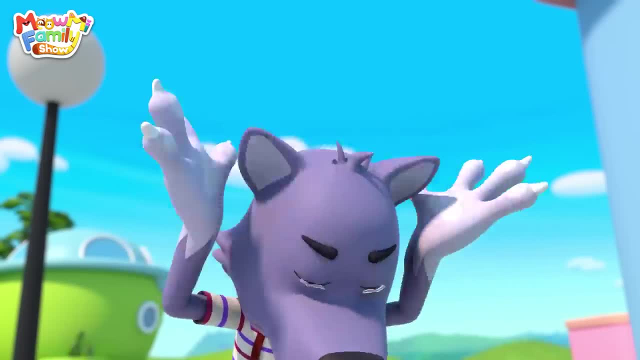 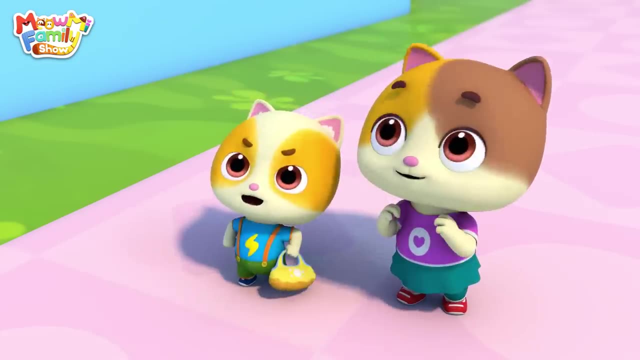 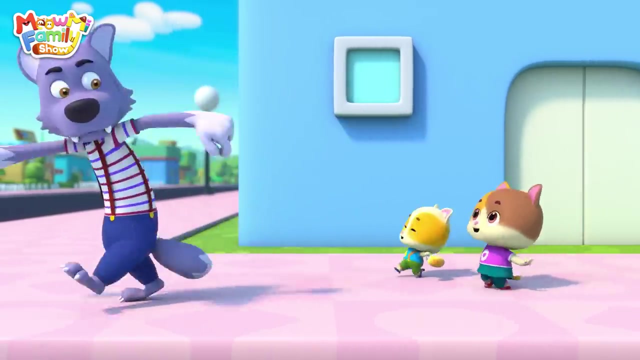 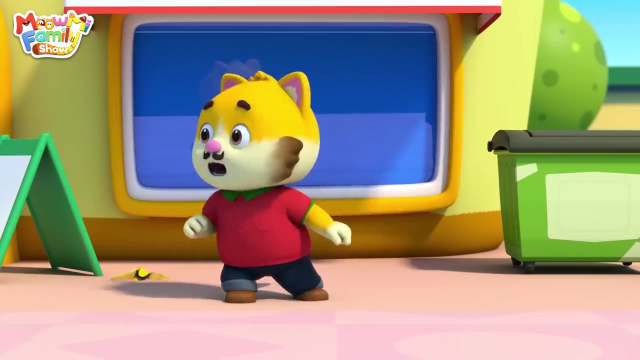 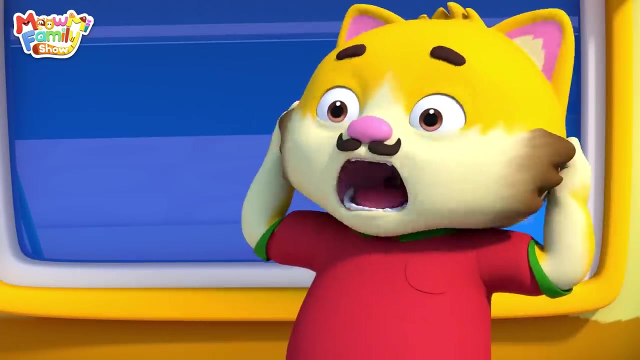 I lost my wallet in the alley. I won't be able to have lunch without it. Don't worry, We'll help you find it. Yay, Thanks, It's not far from here. Follow me, He-he-he, Oh no. 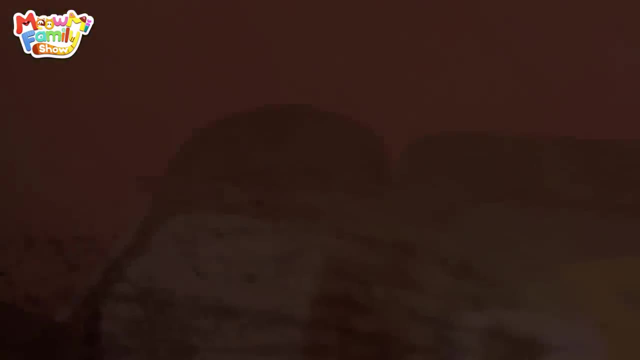 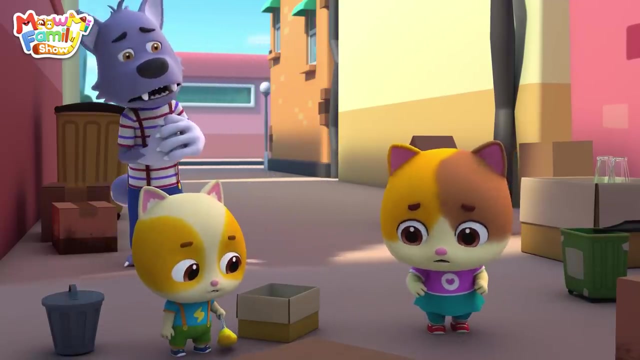 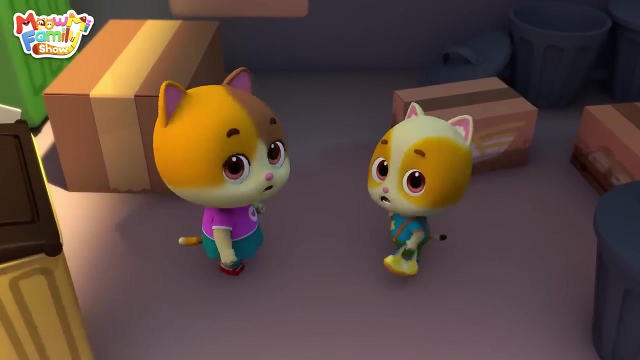 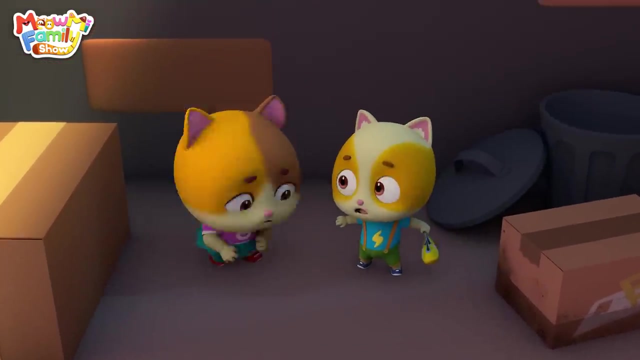 Hey, Hey, kids, You shouldn't go with strangers. It's not here. It's not here either, He-he-he. Of course there's no wallet. What do you want? I'm gonna get you Somebody help, Help. 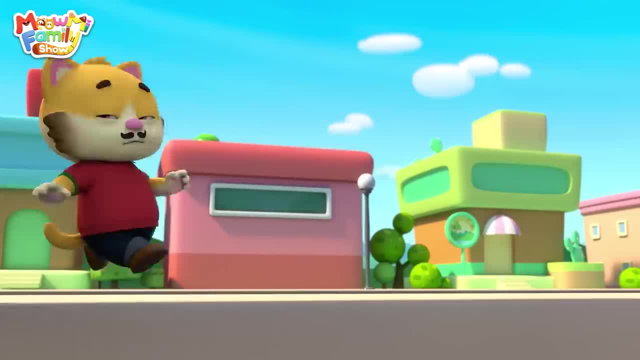 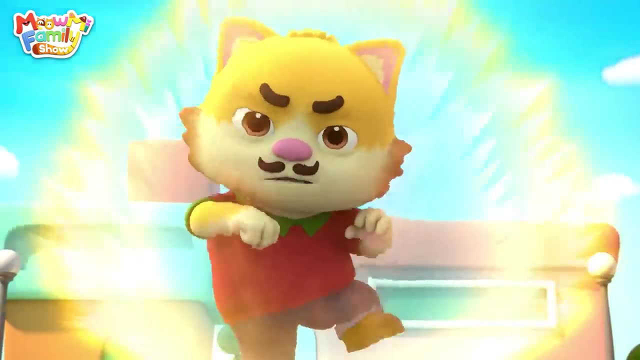 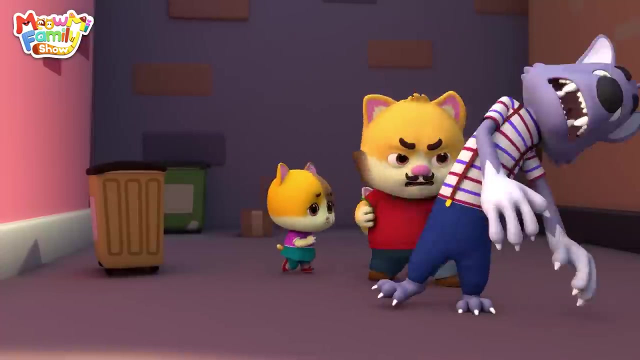 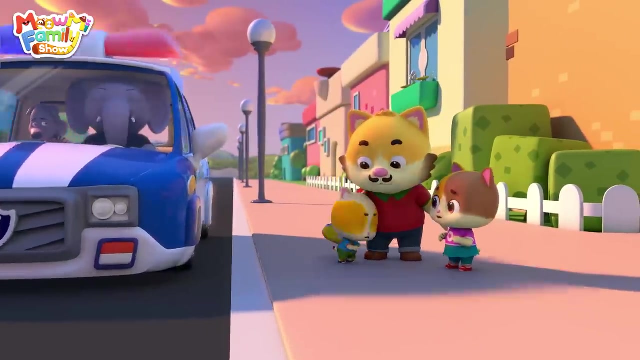 He-he-he, You can't run away. Stop, Don't ever touch my kids. Grrrr Daddy, We were so scared. It's okay now, But remember: adults never end. It's okay now, But remember, adults never end. 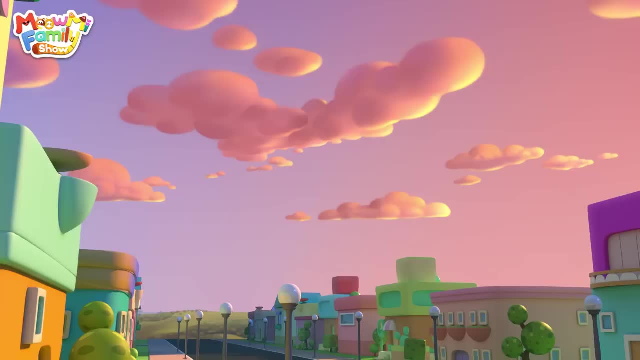 It's okay now, But remember: adults never end. The best way to help kids is to ask for help from children who are weaker than themselves. The best way to help kids is to ask for help from children who are weaker than themselves. Okay, We got it. 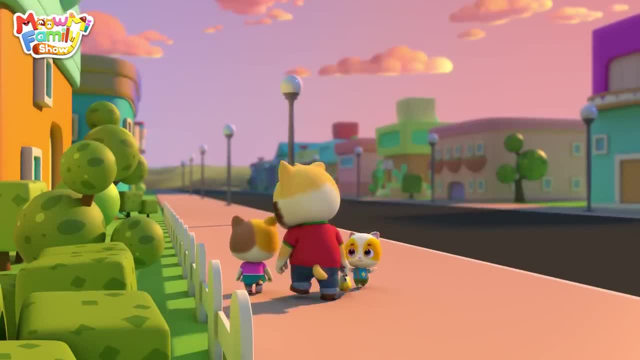 Great, Now let's go home. Daddy, You were awesome. Of course, Daddy was once the weightlifting champion. Wow, He-he-he, Ha-ha-ha, He-he-he, Ha-ha-ha, He-he-he. 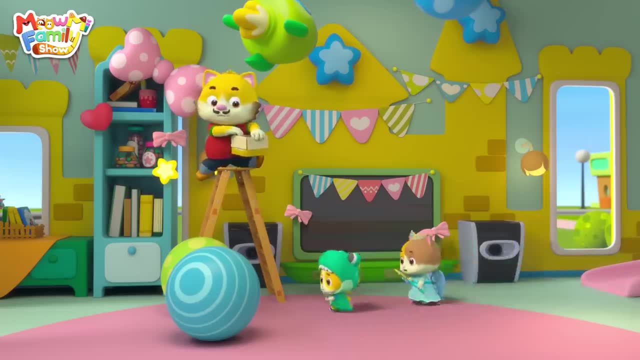 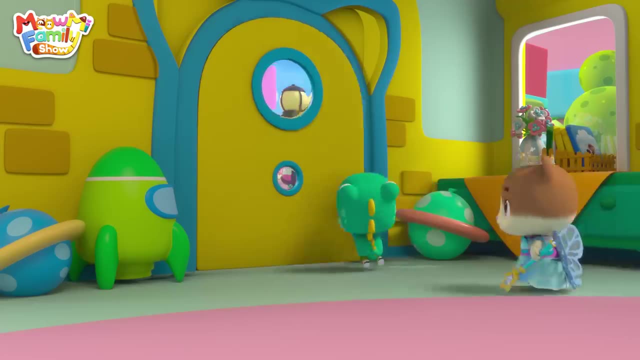 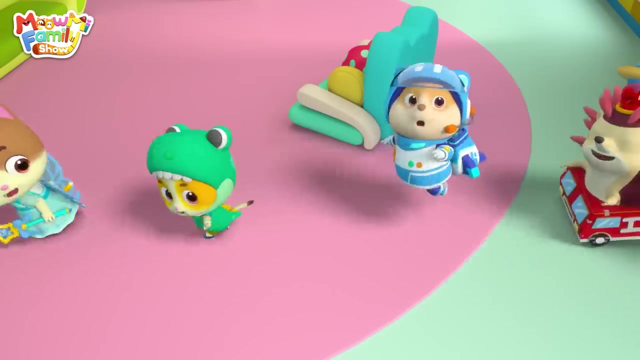 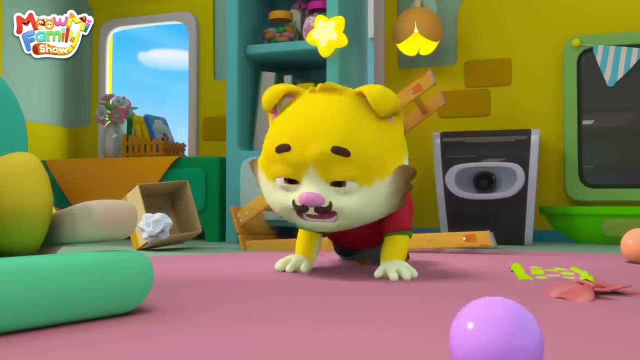 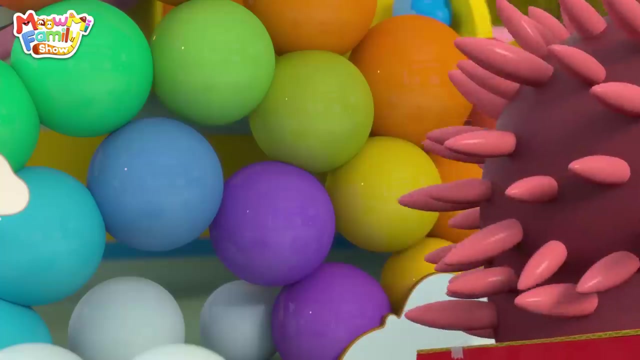 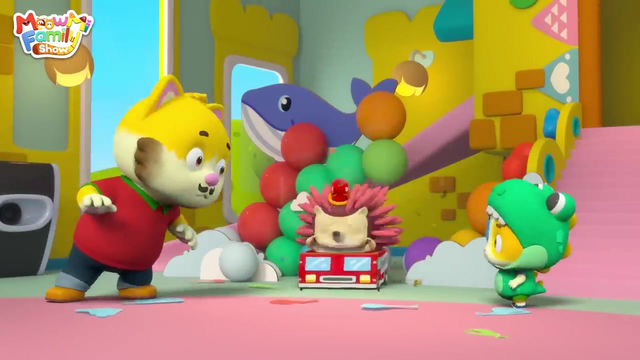 Hmm, We'll open the door. Phew, Hey, we're here to join our party. Come on in. Hi Daddy Cat, Hi everyone. What's going on? I'm sorry, I didn't mean to do that. 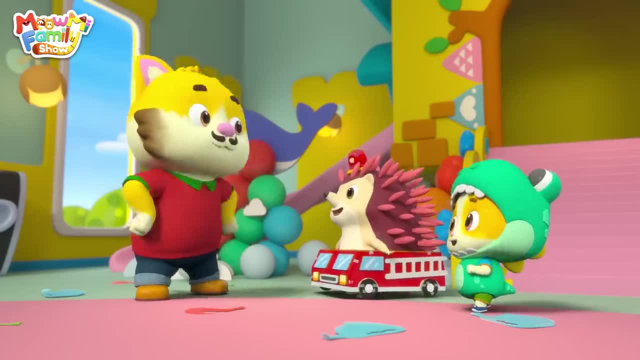 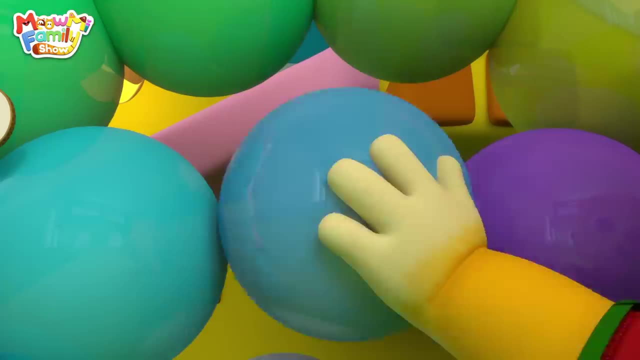 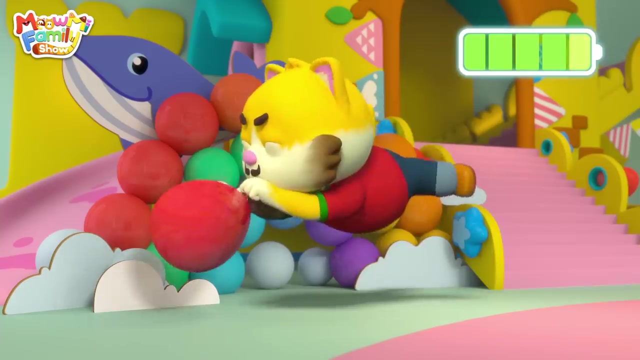 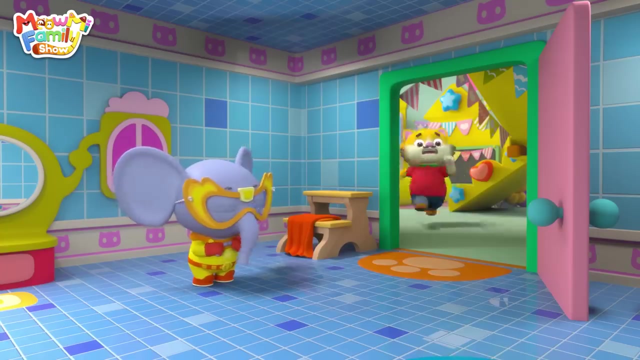 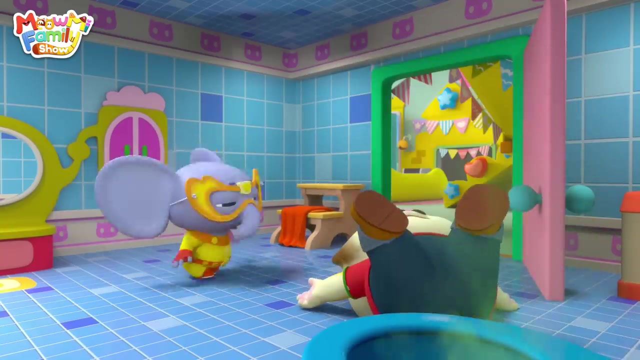 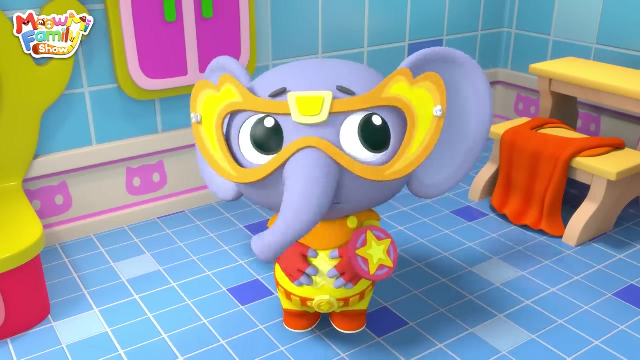 It's okay, Leave it to me. You can go and play. Thanks, Daddy Cat. It's all done. Daddy Cat, I'm coming. Daddy Cat, The toilet is clogged. I'm sorry, I had so much for breakfast. 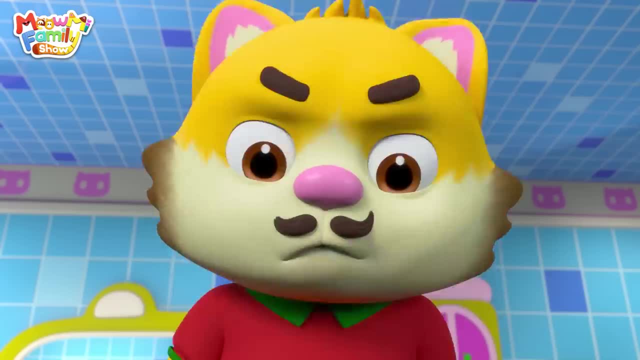 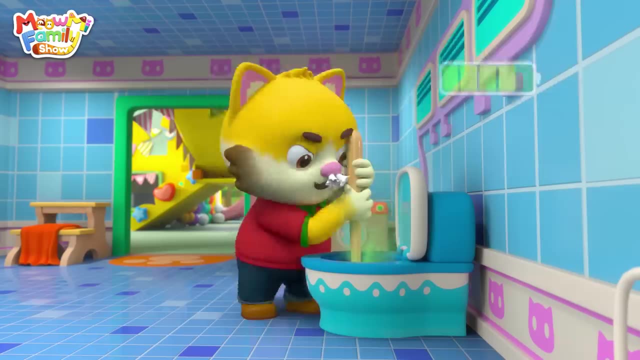 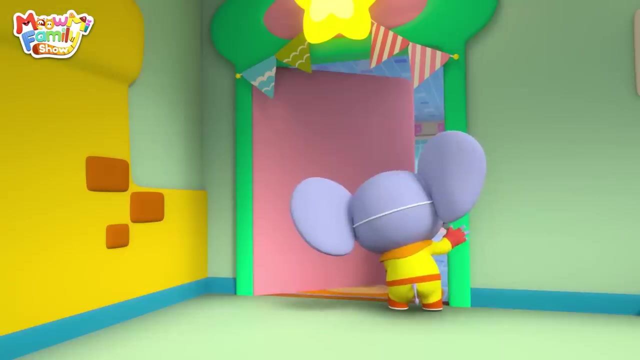 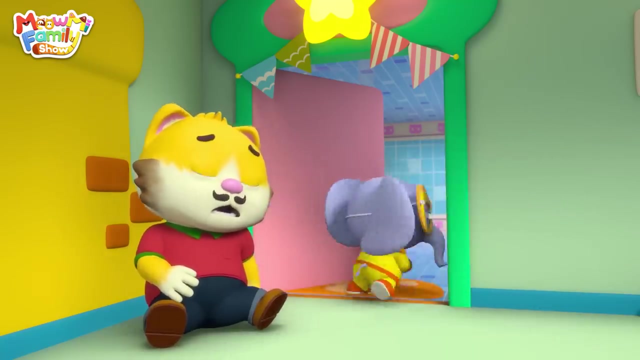 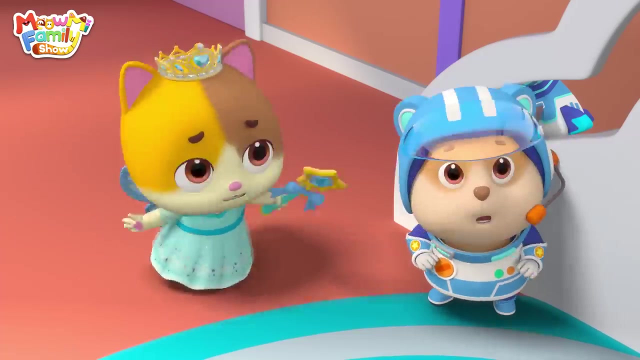 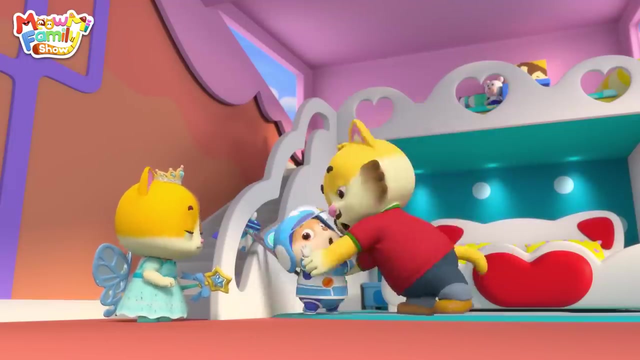 I'll handle it, Daddy Cat. I did it. I need to go again, Daddy, What's going on? Little hamster is stuck. Look, Let me see first. Don't worry, I'll help you out, Hey, Wow. 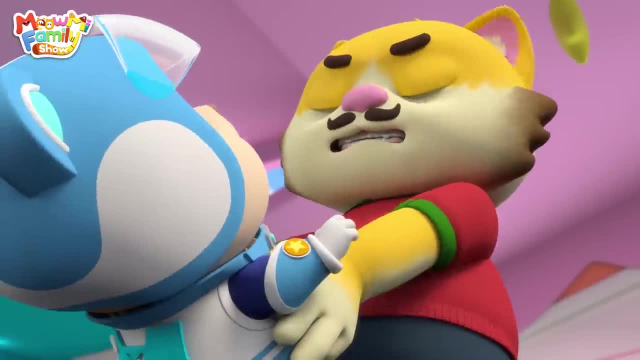 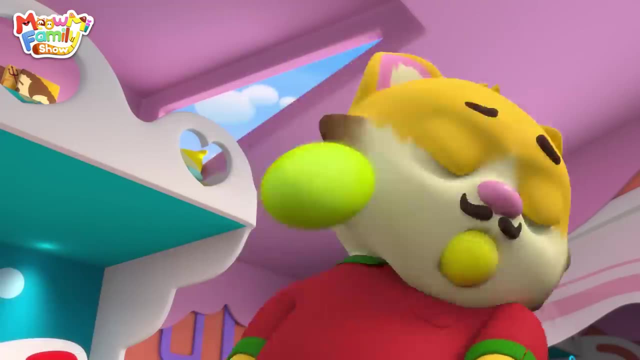 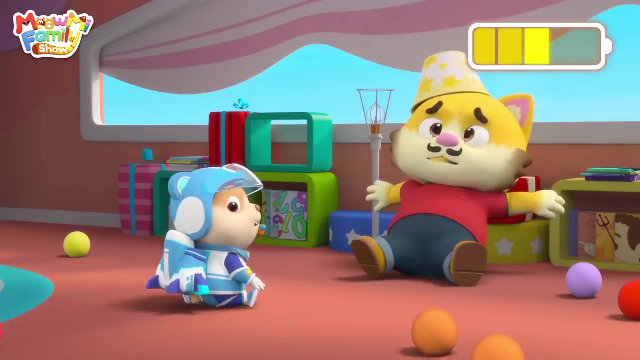 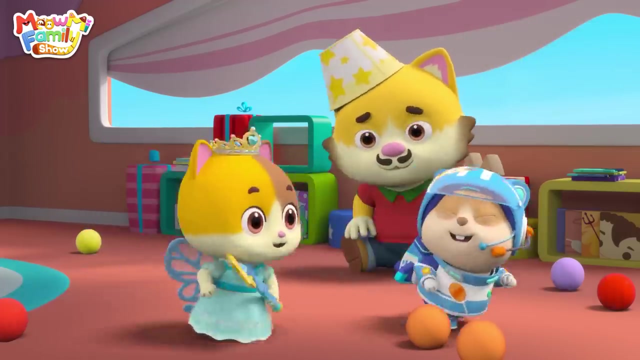 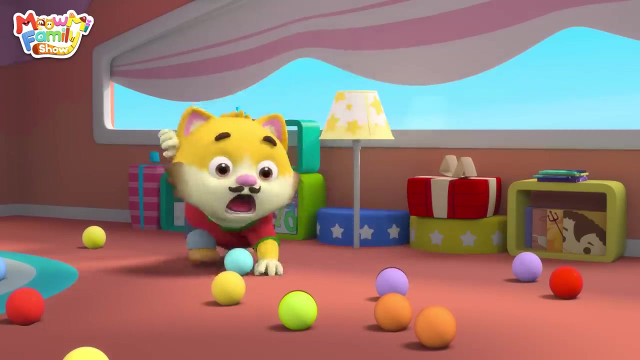 Wow, It's so tight. Nick Almost done. Wow, Wow, I got out. Yay, Hey, No problem. Happy birthday, Daddy. Happy birthday. Happy birthday. Happy birthday to you, Daddy. What, What is it? 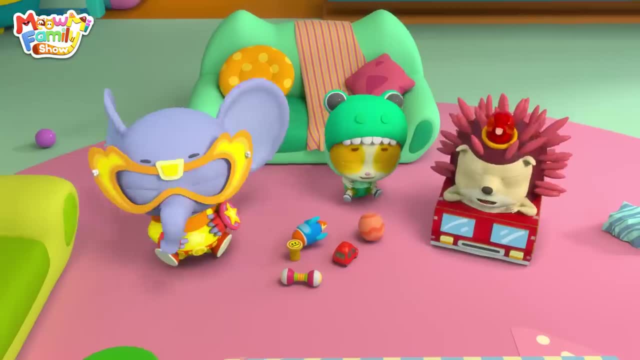 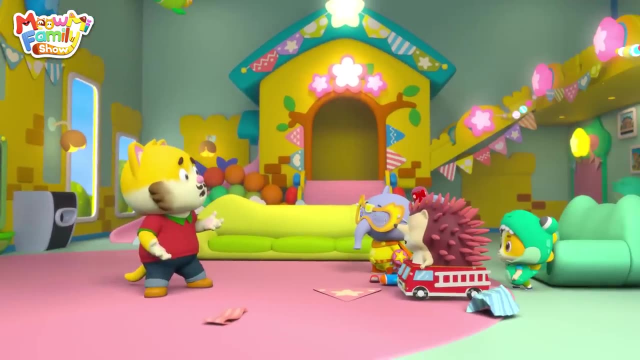 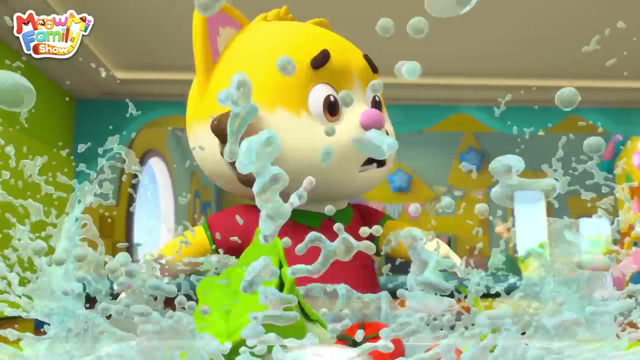 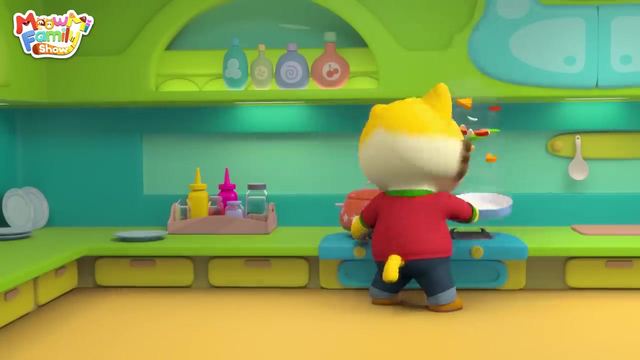 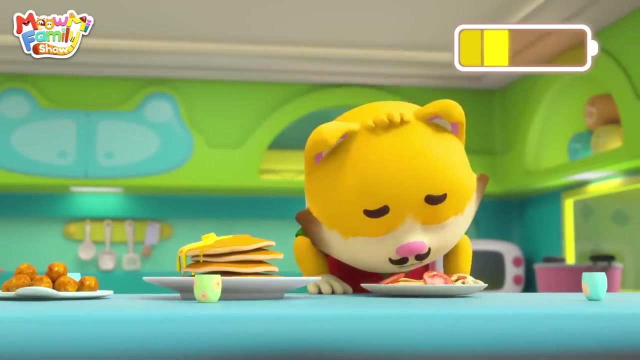 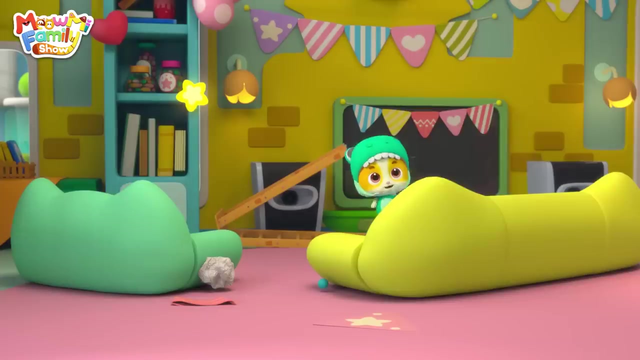 What's going on? kids? We're hungry. Oh Oh, Oh no, I forgot to prepare the food. Oh no, It's all done. Time to eat, kids. Yay Whoa, They look so yummy. 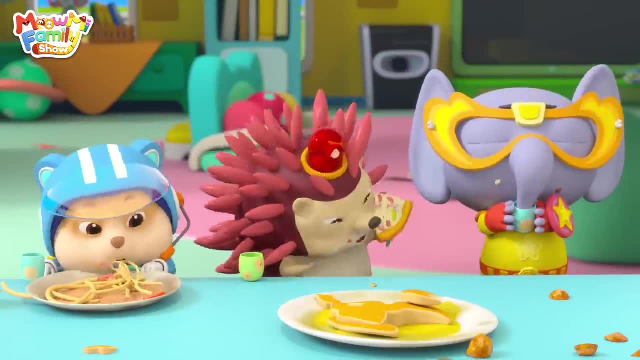 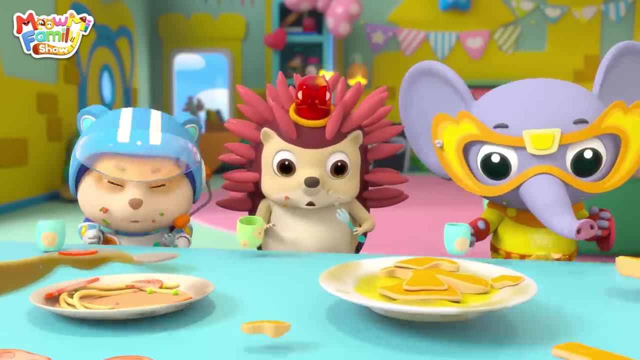 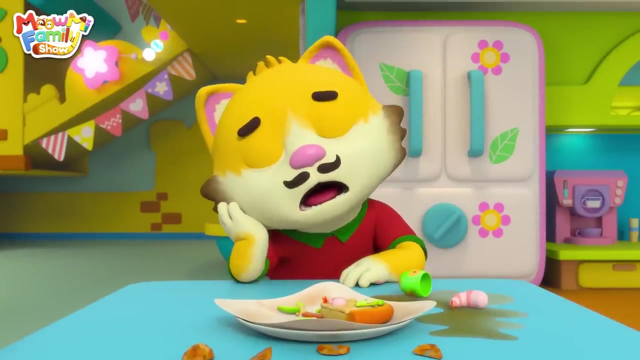 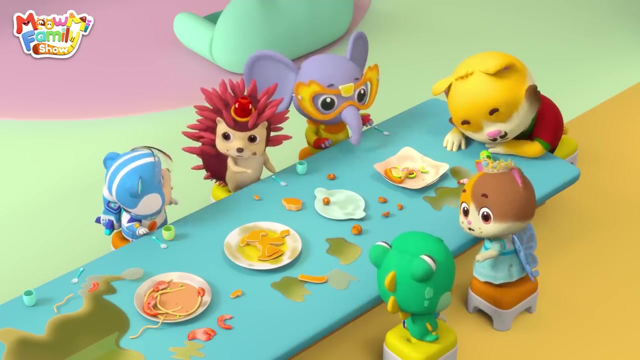 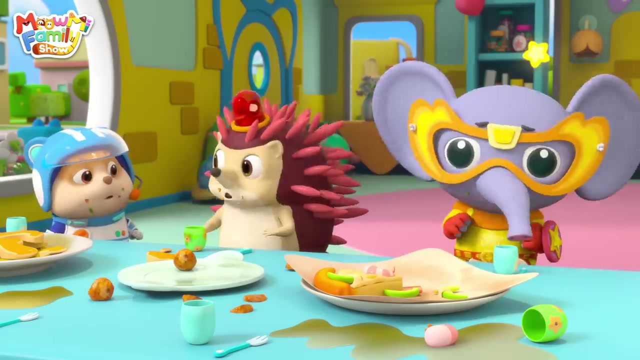 Wow, So yummy. My daddy made them Awesome. Daddy, can't Daddy, Daddy, Daddy fell asleep. He looks so tired. He did many things for us. That's why he's so tired. Then what can we do for him? 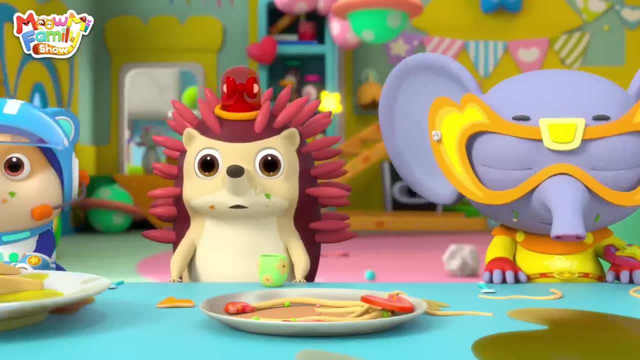 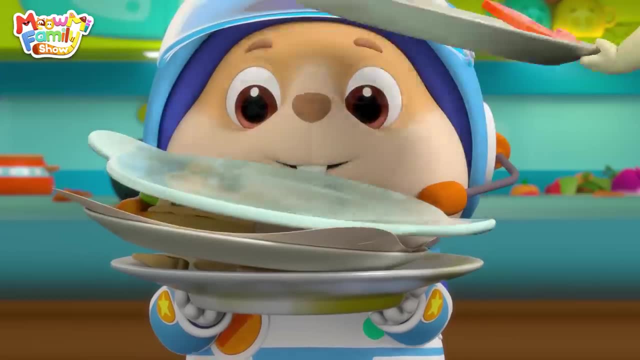 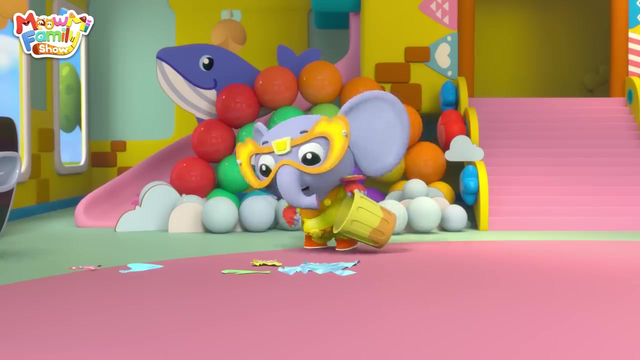 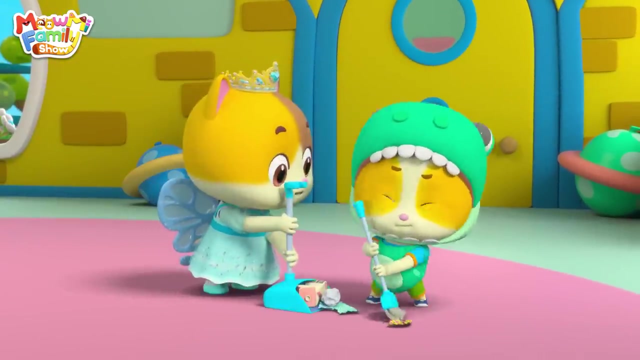 Let's clean the house together, Okay, Shh, Oh, Wow, You're so cool. Hehehe, Wow, What a Hahaha. Hehehe, Hello, How are you? Hehehe, Wow, Hehehe. 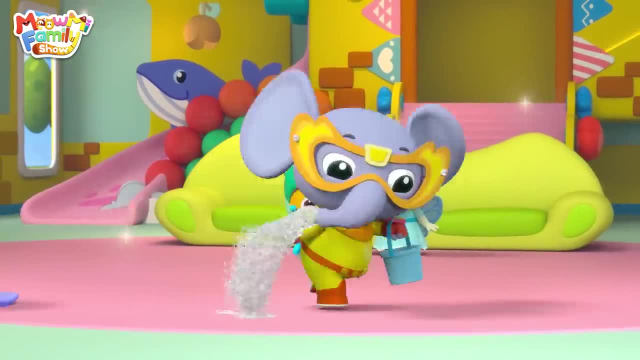 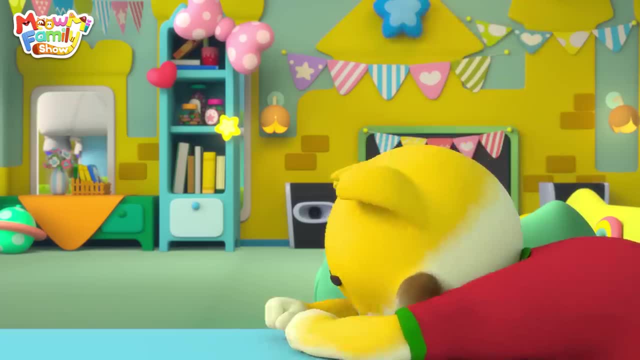 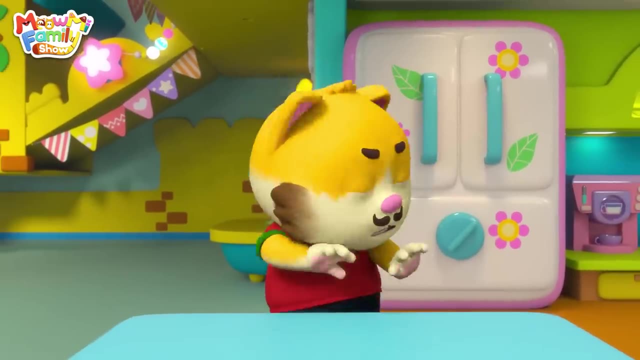 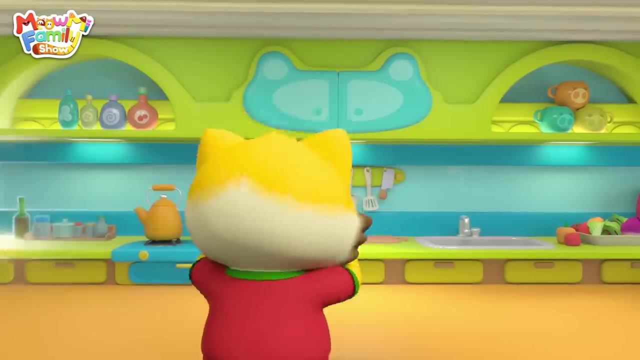 Yummm, Yummm, Yummm, Yummm, Yummm. Huh, Did I fall asleep? I still have a lot of things to do. Wow, It's so clean. Wow, What happened? Who did this? 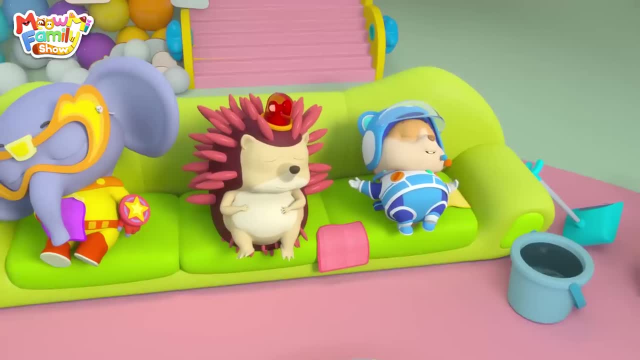 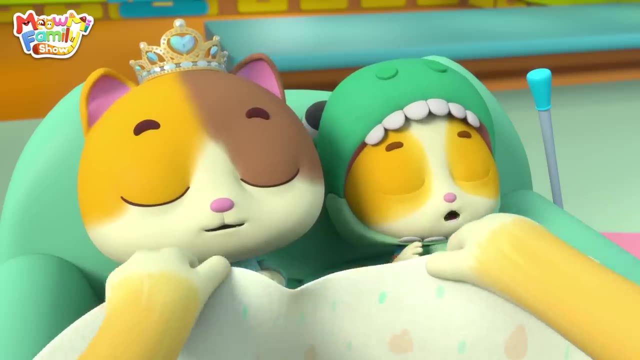 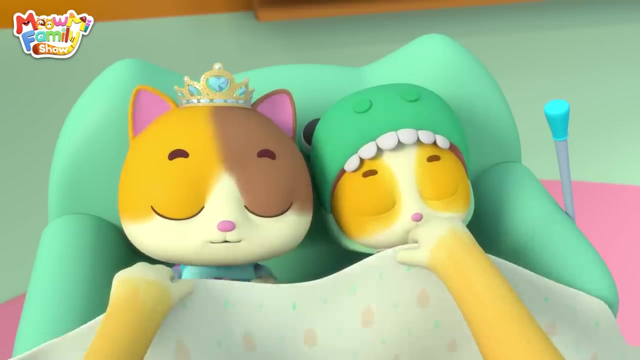 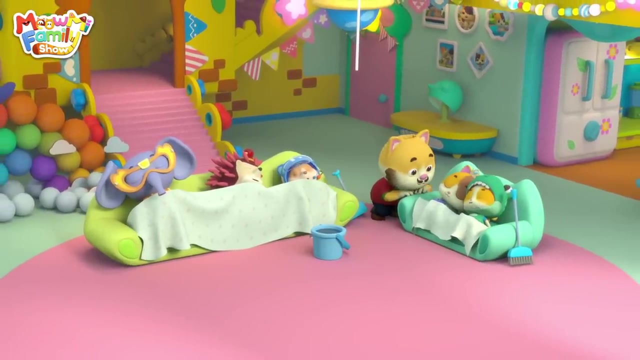 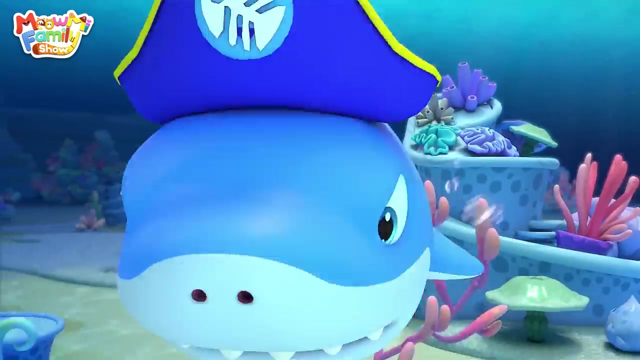 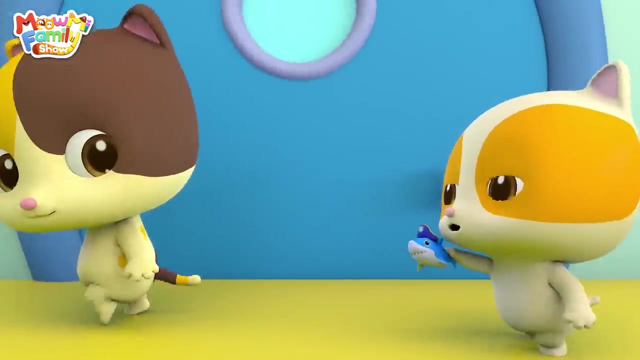 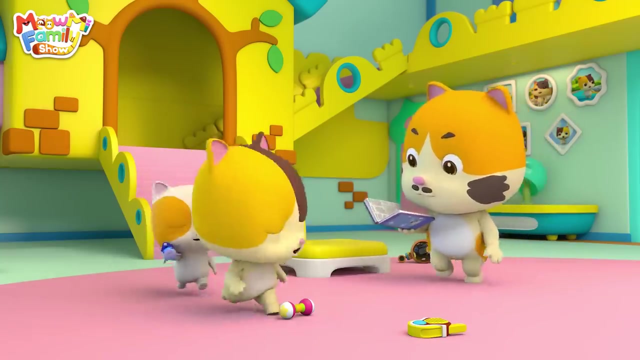 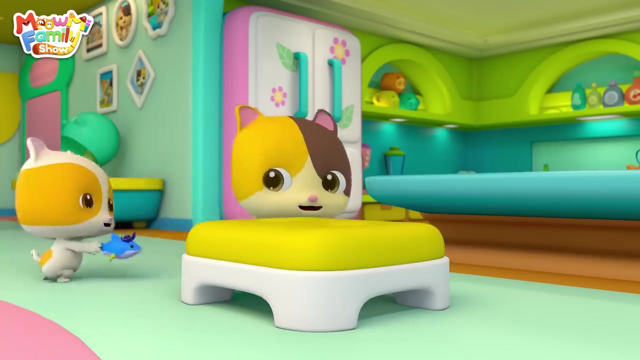 They did all the cleaning. They did all the cleaning. Klaus' work is so hard. We need to help daddy Kids. you're all grown up now, Uh… Oh, Shark, Shark, Shark Kids, be careful, You can't catch me. 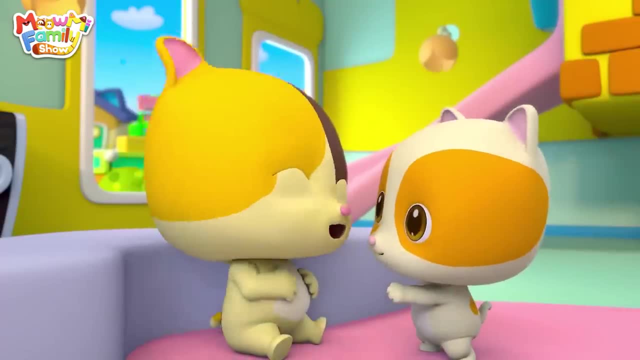 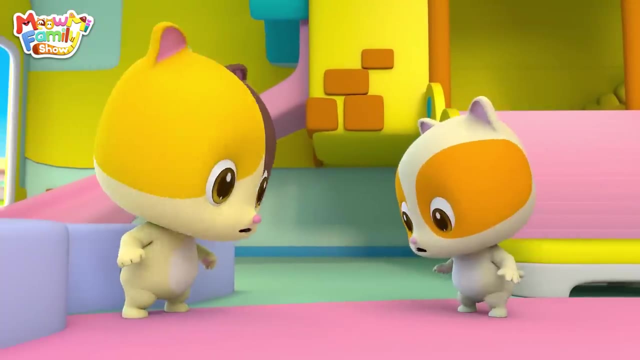 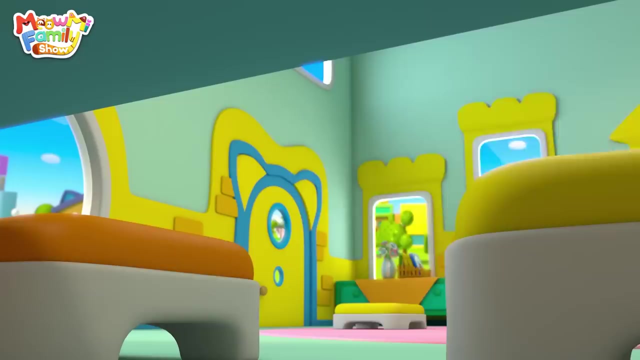 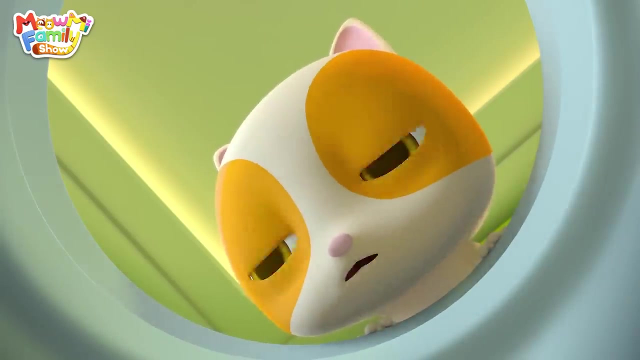 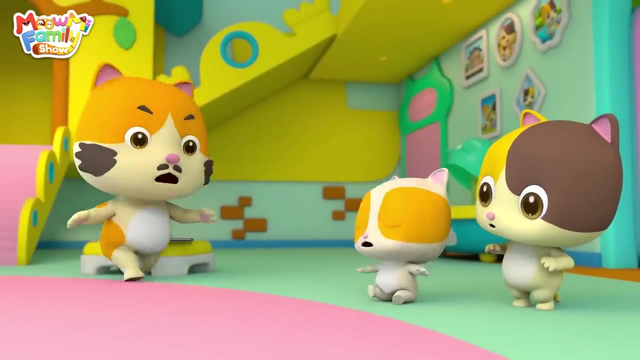 Ha, I got you. This shark is awesome. Where's your shark? Where did it go? Let's split up and find it. I can't find it. My shark Timmy. what's wrong? Daddy? Timmy's shark is missing. 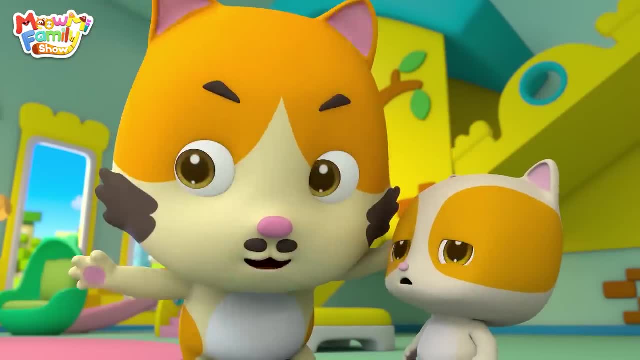 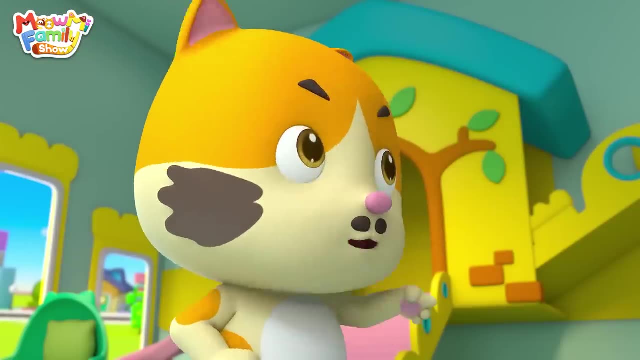 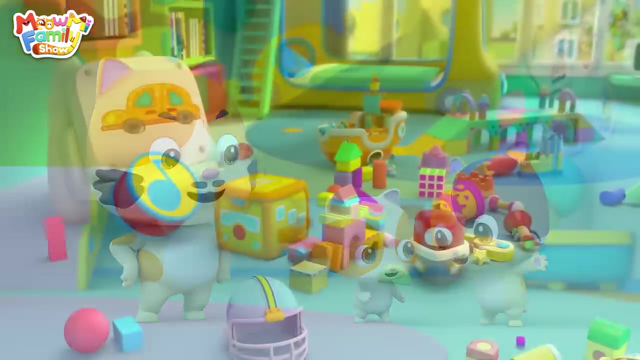 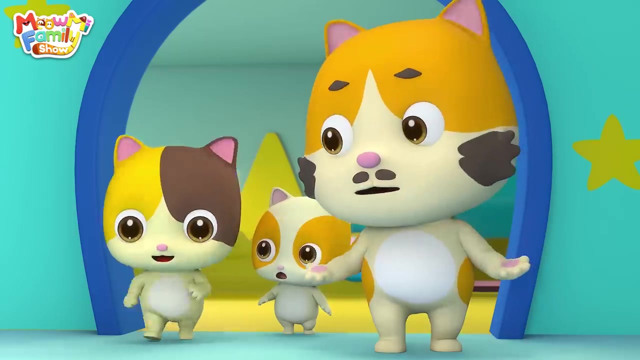 Don't worry, it must be somewhere around here, But we couldn't find it anywhere. Did you check your room? Oh, our room. Oh no, The toys are everywhere. I feel like I'm in the sea. Yeah, daddy. 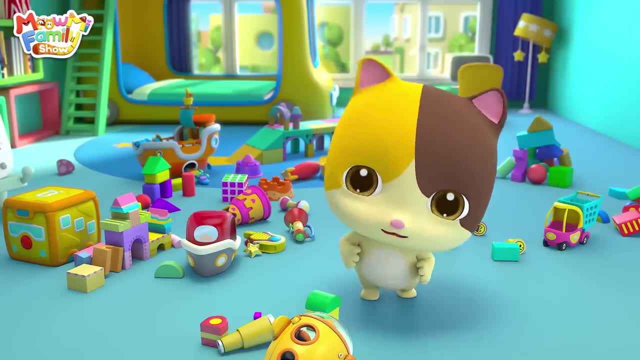 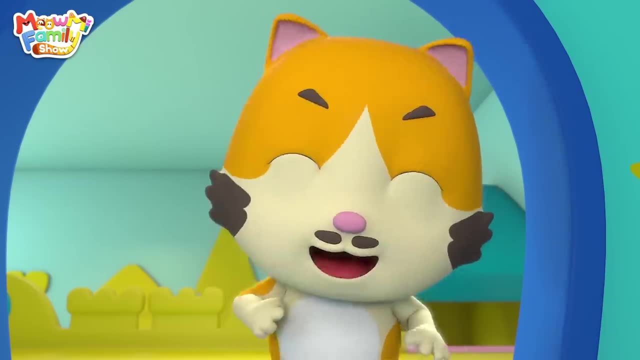 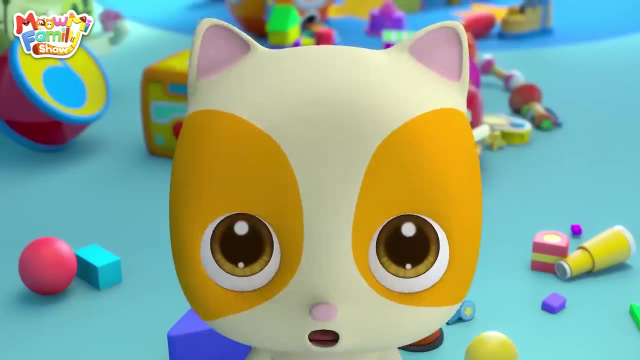 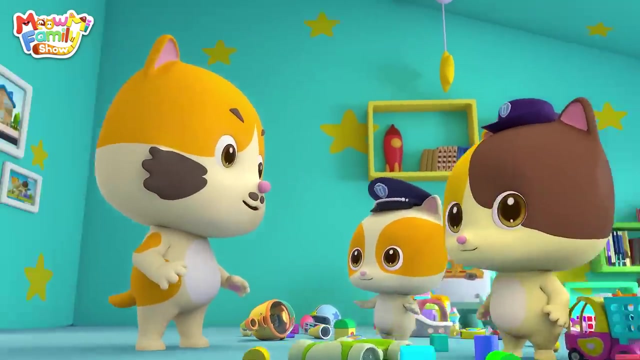 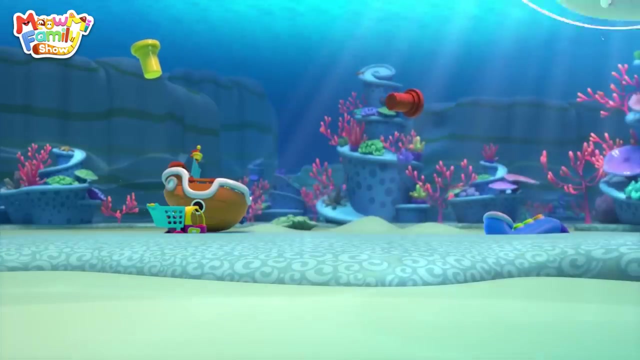 So we played pirates many times here, But where is my shark? The pirate shark must be in the sea. Change into little officers and find the pirate shark. Okay, Officer, Mimi, Officer, Timmy, Let's go, Shark, Shark. 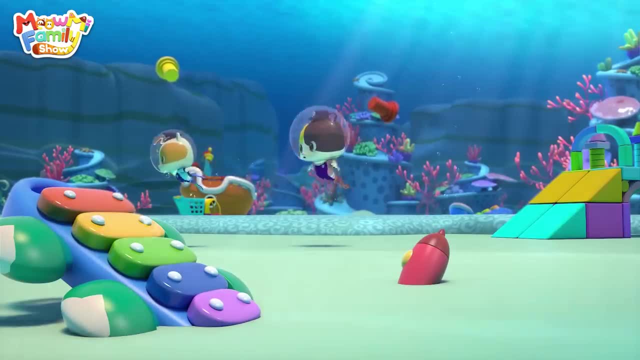 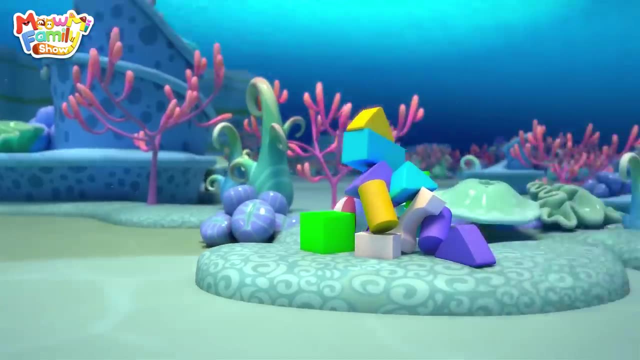 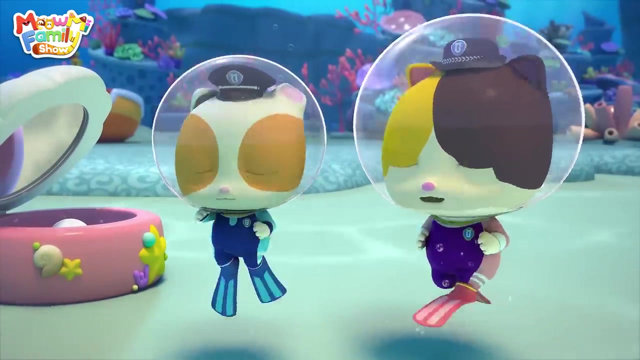 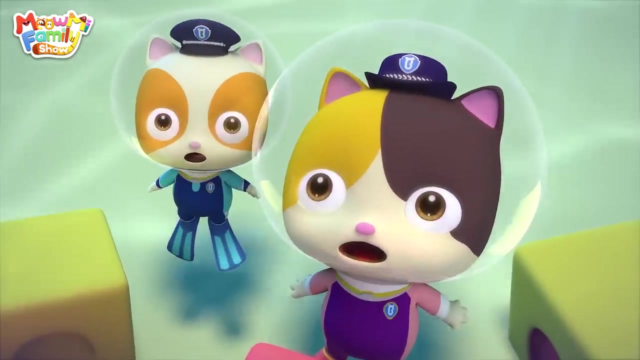 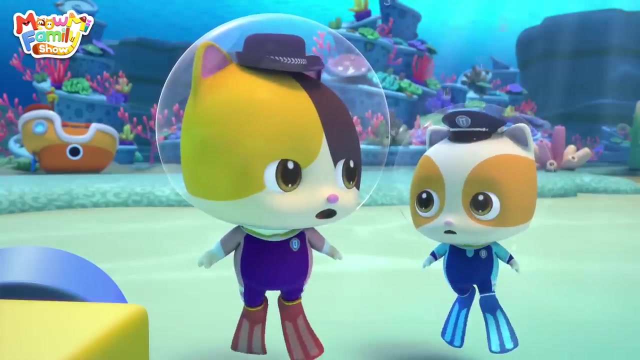 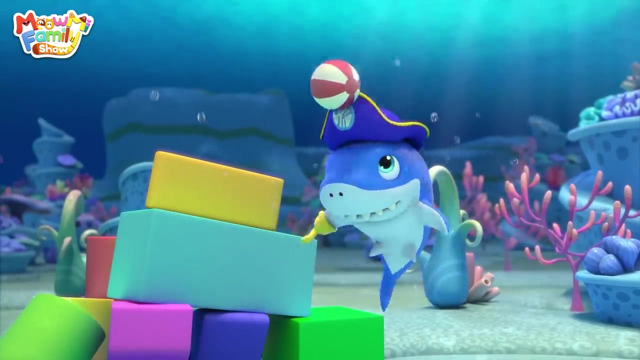 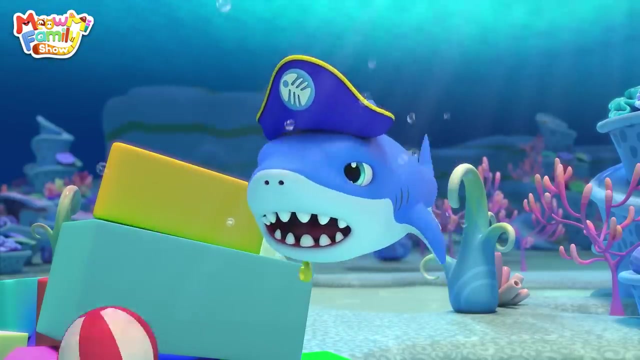 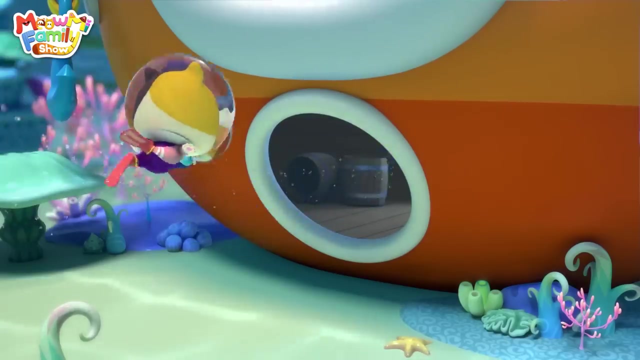 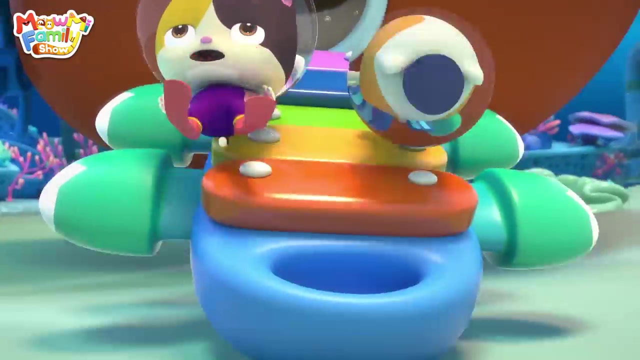 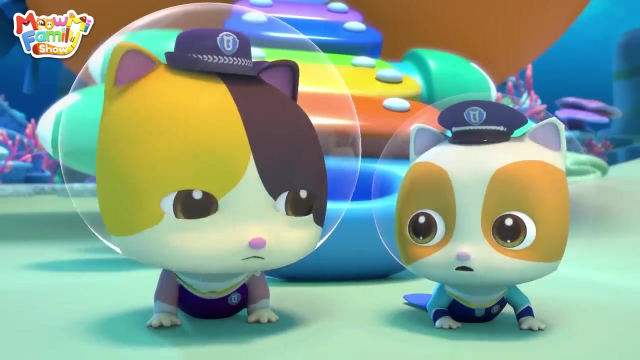 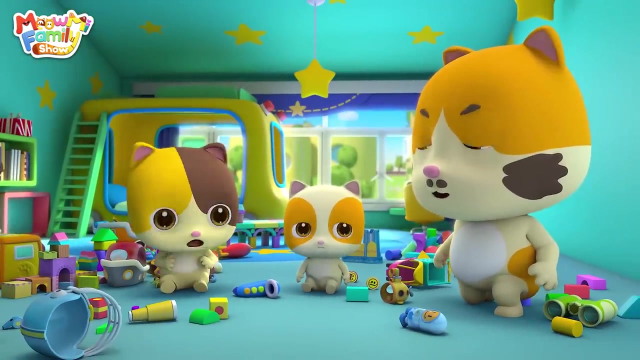 Where are you? It's not here Over there. Woah, Ahhh, Weeeeee, It's a rocket. Wh-what? Oh, my shark, We found you. Hurry. There are so many toys. The shark keeps hiding among them, so we can't find it. 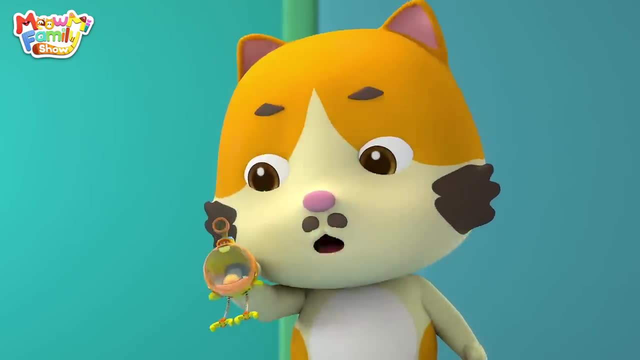 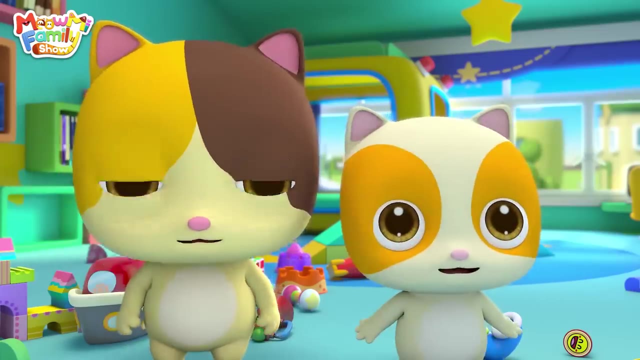 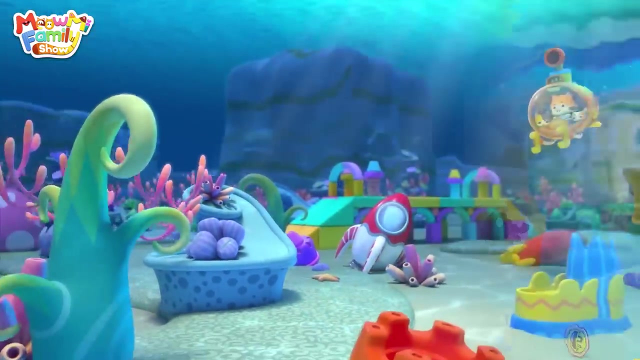 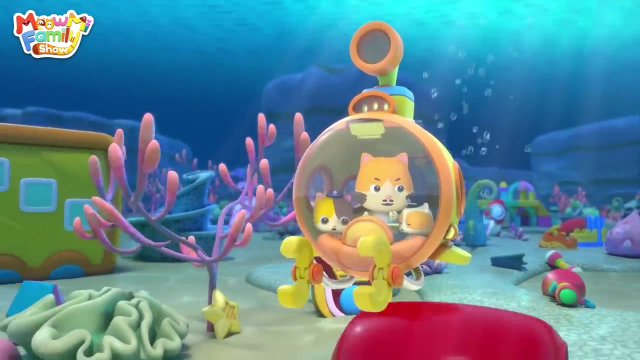 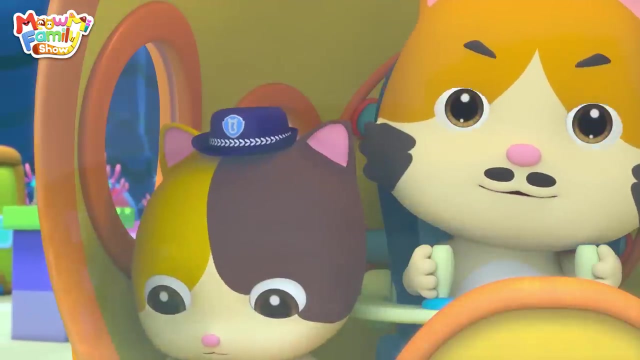 Well then, how about you put away all the toys first? That's a good idea. The shark will have nowhere to hide. There are so many toys, Which one shall we choose? Which one should we put away first? The shark likes to hide behind the big toys.